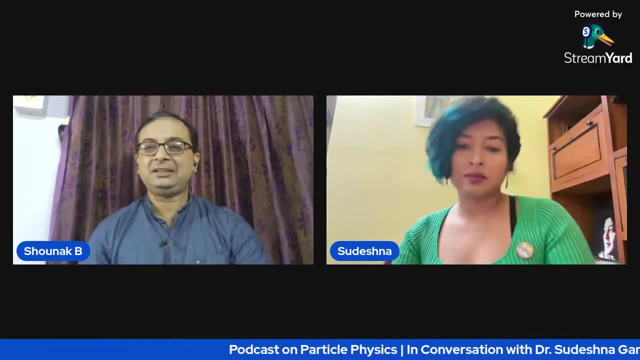 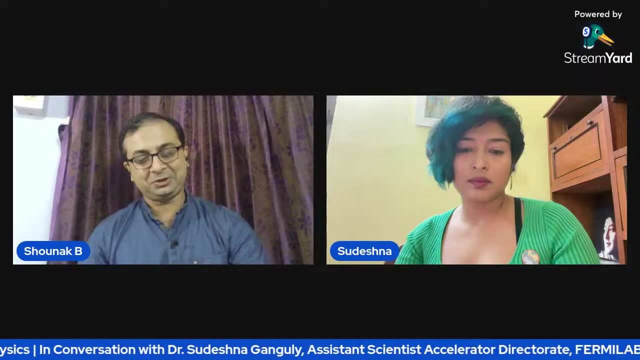 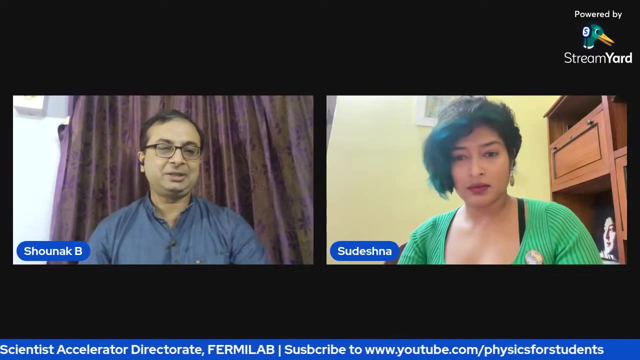 She started at Bethune College and, traversing through IIT Delhi to Wayne State University, her academic pursuits have been a testament to her passion and dedication. Her invaluable contributions to experiments such as Bell and Fermilab Muon G2 exhibit a profound expertise in this intricate field. 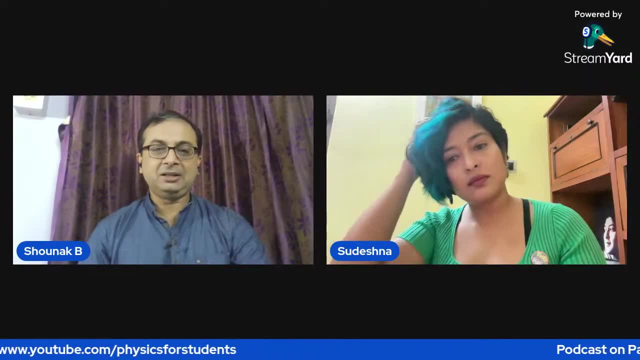 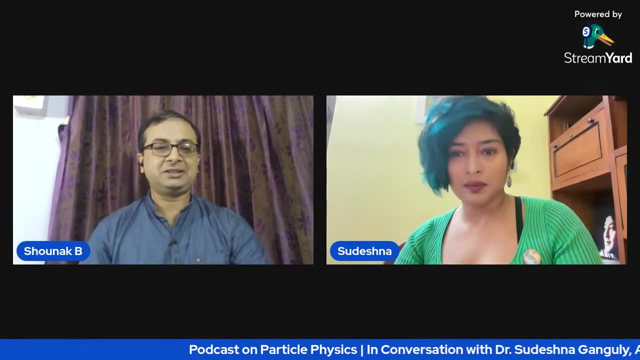 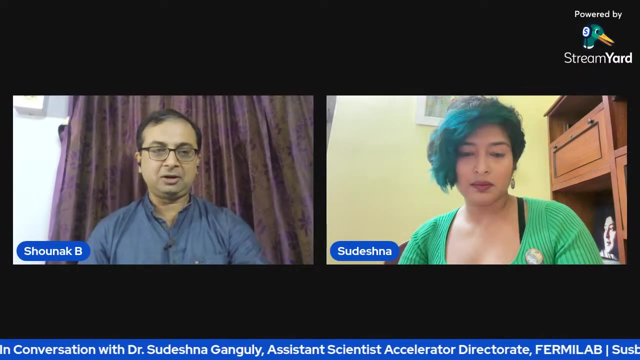 Currently serving as an associate scientist at Fermilab. her dedication to advancing neutrino beam instrumentation for the LBNF beamline showcases her commitment to the forefront of particle physics exploration, To our live audience on YouTube and our esteemed guest Dr Ganguly. 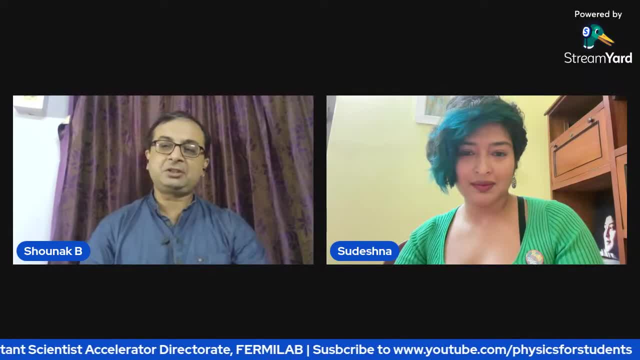 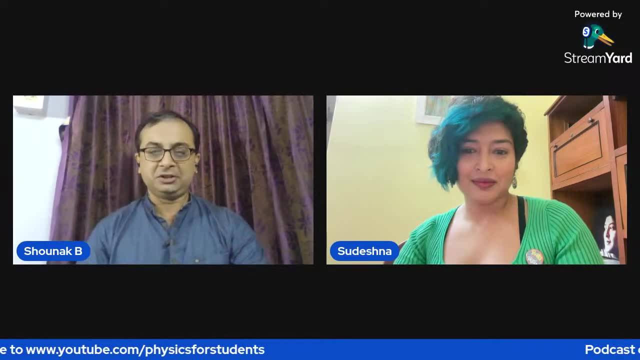 thank you for joining us on this captivating journey into the depths of particle physics. And Dr Sudeshna Ganguly, thank you for gracing us with your presence and to all of our viewers. let us get ready to be enthralled by her expertise and passion for particle physics. 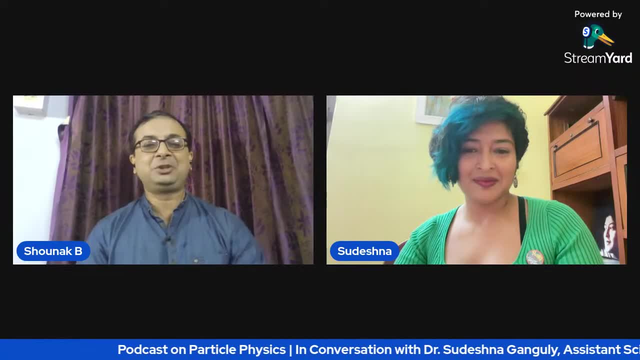 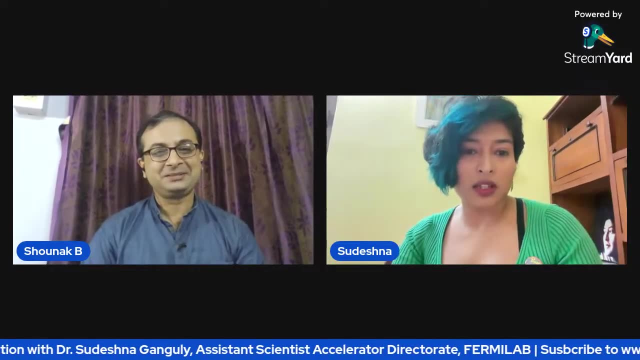 Let us delve into the mysteries of the universe together. Welcome, Dr Ganguly. Absolutely. Thanks so much, Rona, for this opportunity. This is… time actually, i'm talking to people from my own country about my work. i have given talks to many. 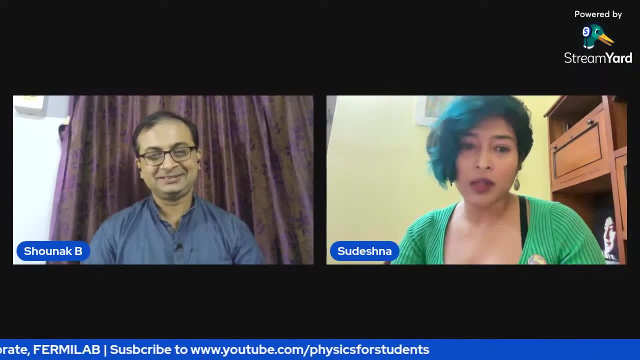 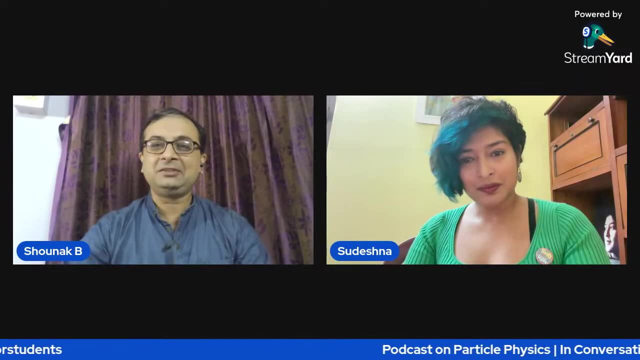 other countries, people from any other countries, but not to my own people. so i'm super excited, thank you. thank you very much, doctor. we will have, uh, many people joining with us, because they are all excited. they're very knowledgeable in terms of asking questions, etc. but first of all, as you, 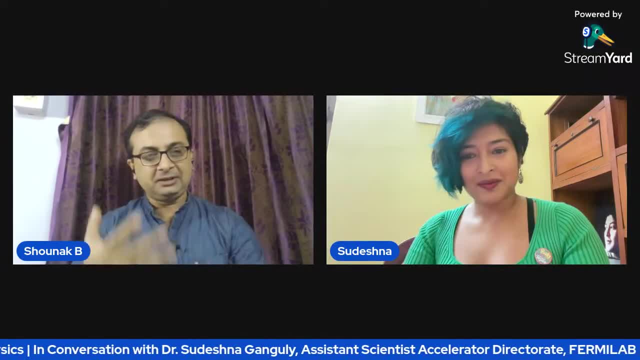 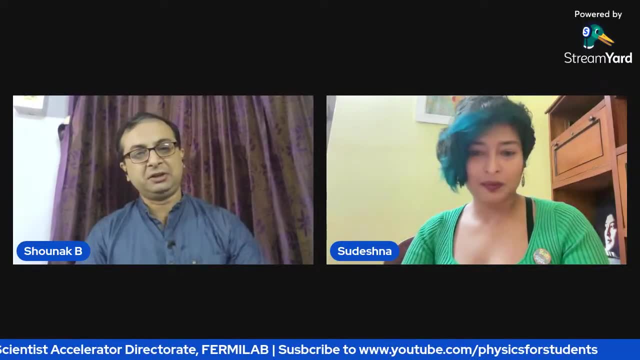 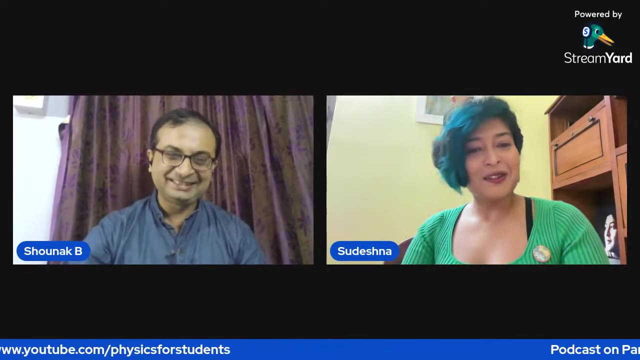 have already told you, have a kind of a prototype thing which we actually need to go through. my first question to you, doctor, would be: what are the fundamental forces in the universe and how do they manifest at the particle level? perfect, i do have the answer prepared already, so, if you can, 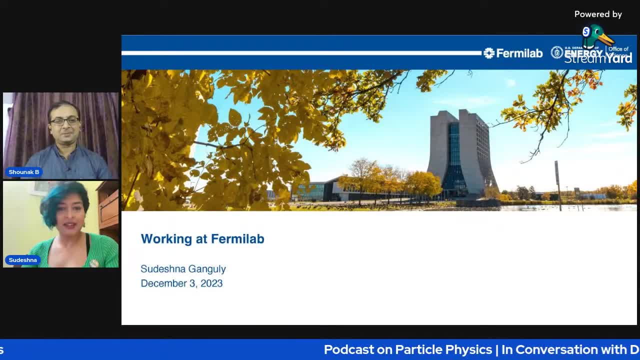 show the slides. thanks so much, all right, so, so, yeah, to answer your questions, we will, of course, talk about the fundamental particles and fundamental forces and the basics absolutely, and then i will try to talk a little bit about my work, um, the experiments specifically that i work on at fermilab, and, uh, in doing so i might be able to. 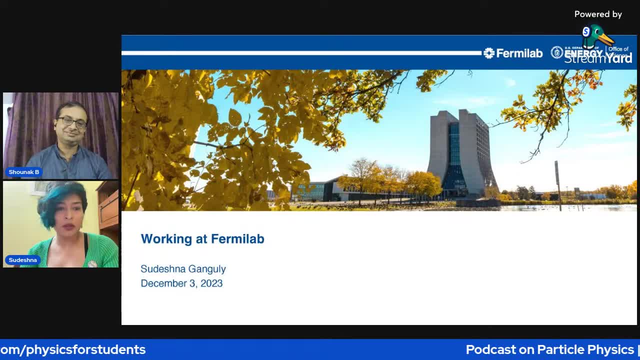 encourage many people here to come work with us at formula. that'll be exciting. and then um, on my slides. if the slides are available, i have shared some links which might be useful. uh, for future purposes. awesome, so. so let's get into the questions and the content of the slides. okay, so i wanted to 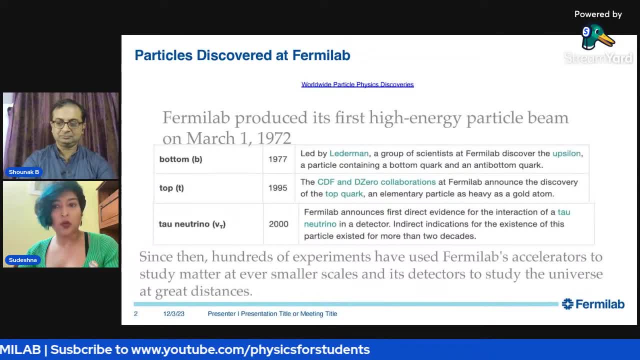 start with sharing a little bit of history. so all that happened before, way before my time, before i joined the lab, but i just wanted to share a little bit of history. so in 72, that's when formula produced first high energy beam, and you can see uh. on this link you will get more details. 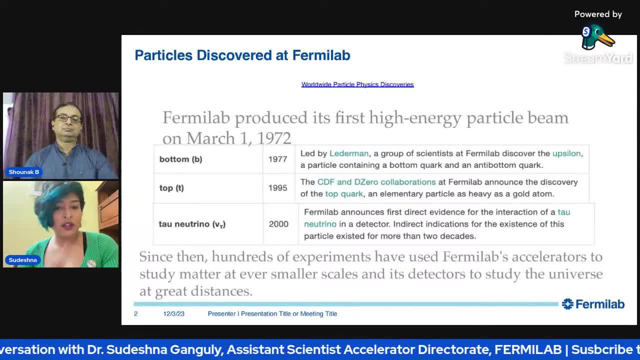 just wanted to highlight this for you. uh, in 77, uh, led by letterman, leon letterman- he was one of our directors, i think he became a director from 1179. so a group of scientists led by letterman. they discovered this epsilon particle, which is a. 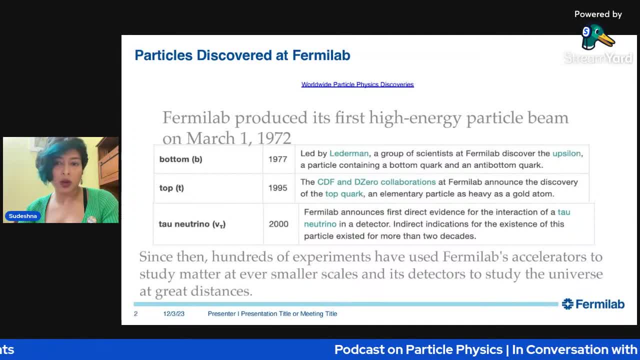 meson. so that's made of bottom quark, bottom and anti-bottom. then in 95 top quark was discovered by cdf and d0 experiments. those are two famous formula experiments. that was in 95, um- i was really a small child back then- um 2000 and they first saw the direct evidence of another fundamental particle. 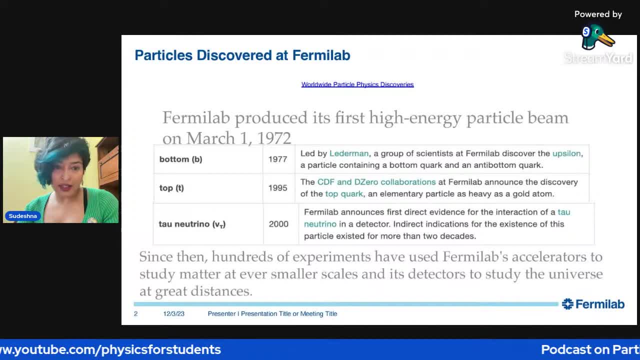 tau neutrino. so so all these exciting things already happened before i joined the lab, but that doesn't mean that we're not doing something exciting now, so we are continuing to do that, um. so so i mentioned a few particles here: bottom, top, tau neutrino, all these. 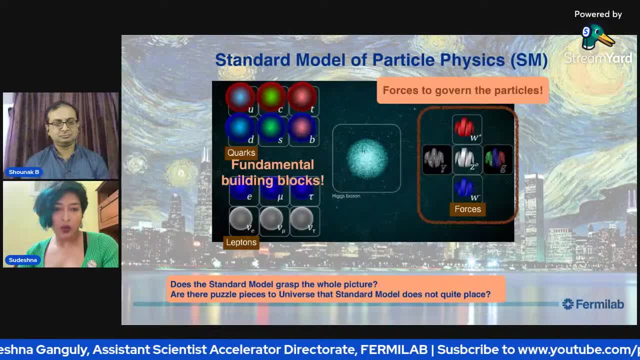 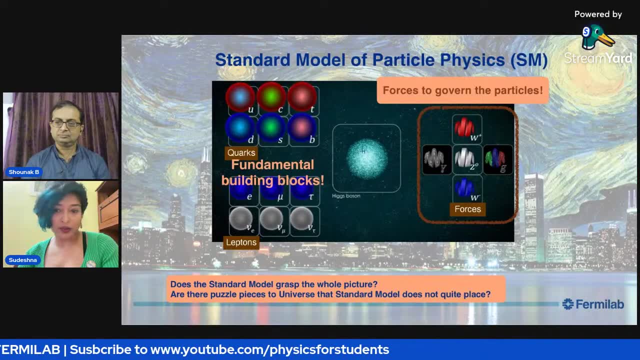 are fundamental particles, so let's now get into what these particles are so. so what happens is that in in physics scientists, we we have a theory that describes almost everything that we perceive around us- um. it is called the standard model, um, so it has been incredibly successful in predicting experimental results over many, many decades. so we can argue. 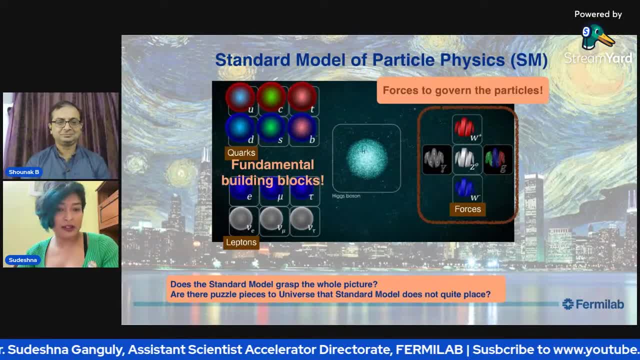 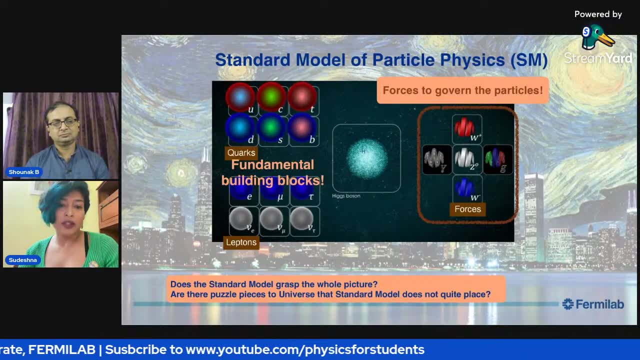 that it is humanity's greatest achievement because it has been so successful, right, um so what does it tell us? it tells us that the fundamental building blocks, uh, they come in two types: quarks and laptops. so so the quarks are like this tiny, indivisible particles. uh, they're the building blocks, basically, that make up protons, neutrons. 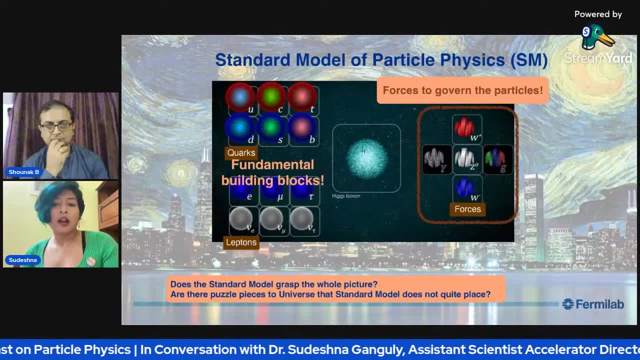 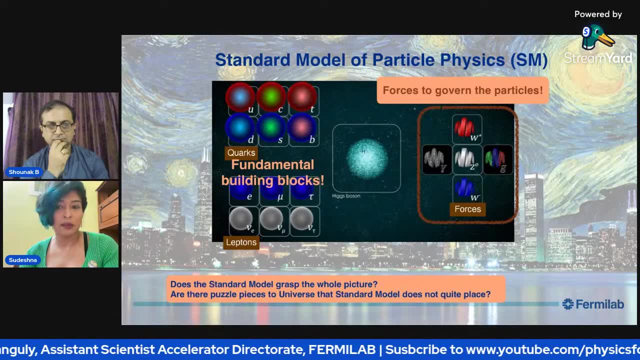 uh, those reside inside nucleus of an atom, right um. and then we have leptons. these are another types of fundamental particles. they they come in one piece. that's why you call them building blocks. so we know of electrons, most of us know know of electrons. electron is the type of electron, right? 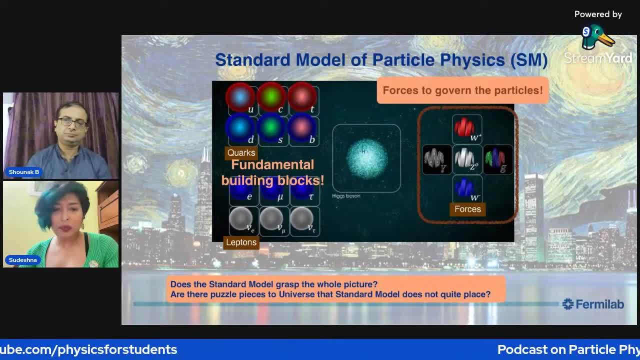 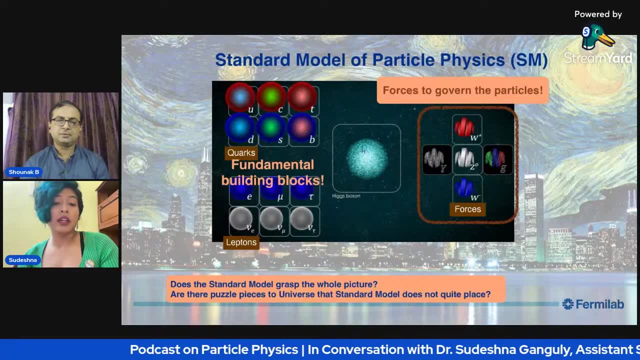 so, again, they are tiny charged particles, um, and they, they are the ones. electrons are the ones that make up the nucleus of an atom, right, okay, and we cannot forget higgs. uh, in 2012, higgs was discovered by our fellow lab in europe, cern, um. so for higgs, i like to use this analogy. 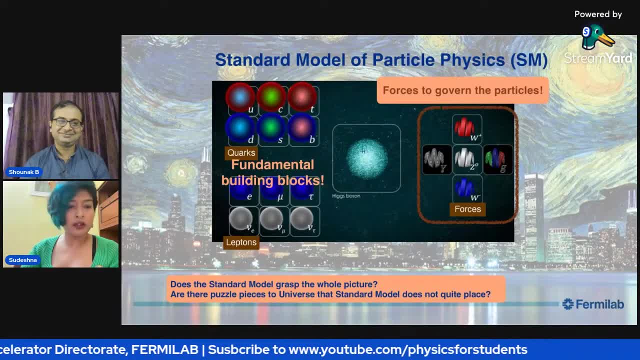 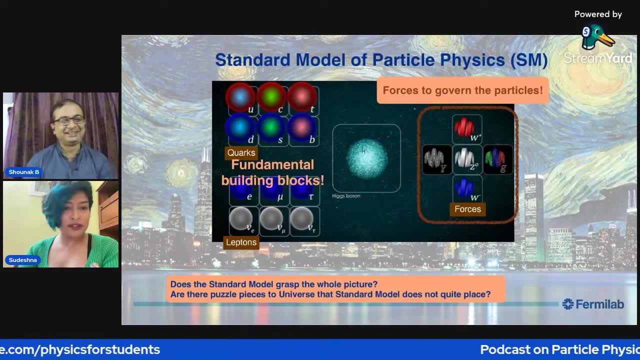 of a celebrity at a party. so when you are near the celebrity then you gain more attention. so higgs somewhat, does that. this is like a special particle, yeah, which is mass to other particles. so it helps us describe, like, why some particles are heavier than others and 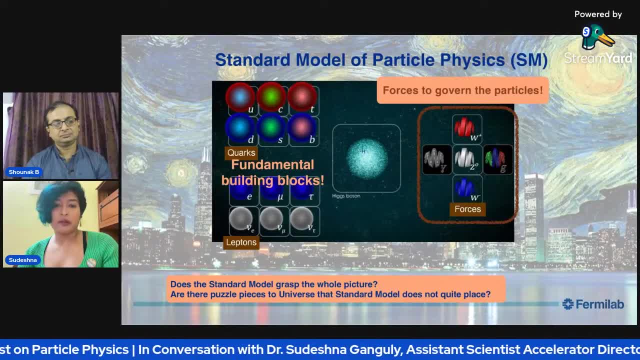 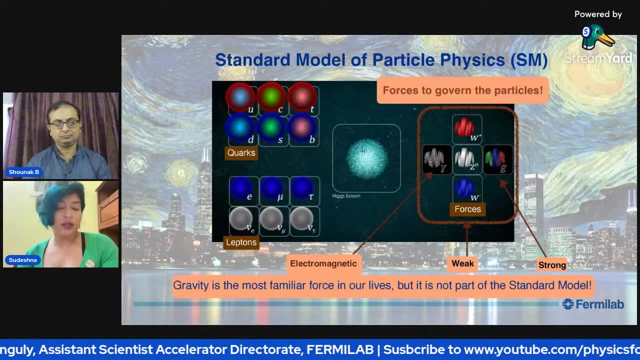 universe. so so we do have these fundamental particles, right, and so we need something to govern this particle, um, otherwise they will just go unruly, right? so we have these three different types of forces: fundamental forces, electromagnetic force, uh, nuclear force, weak force, weak nuclear force and strong nuclear force, right? so electromagnetic force is the one that is. 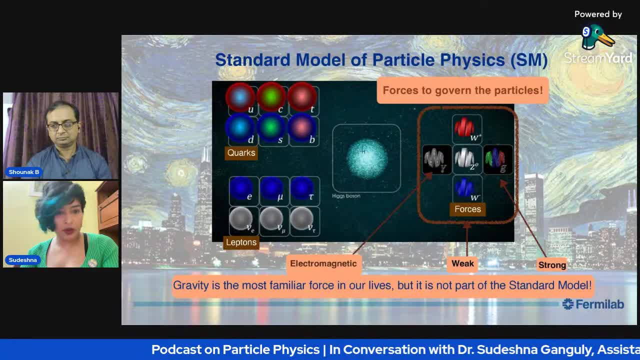 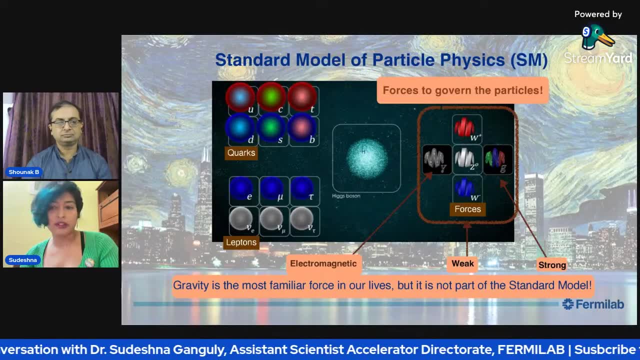 responsible for interaction between charged particles, electrons, protons, um. so. so this is the one that is responsible for interaction between charged particles and neutrons, and then we have weak force. so this is something, uh, which we would see in radioactive decay, so it changes one type to another type and then the strong nuclear force that actually holds the 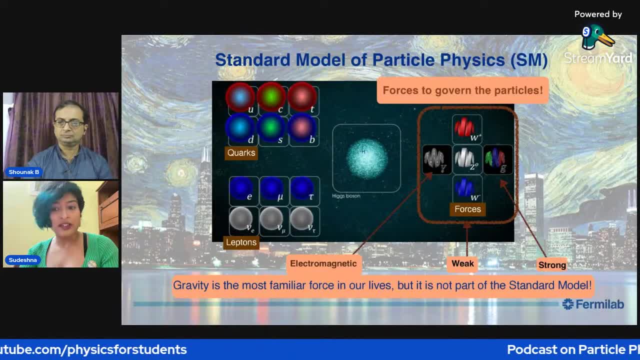 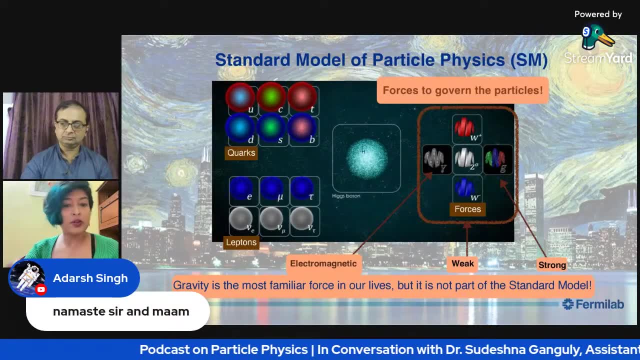 quarks together. that's why the protons and neutrons exist. so it's a very short range but extremely powerful right. so. so these are the fundamental forces which will govern all these building blocks and- uh, disclaimer- gravity, which is most common in the nuclear world, is a very 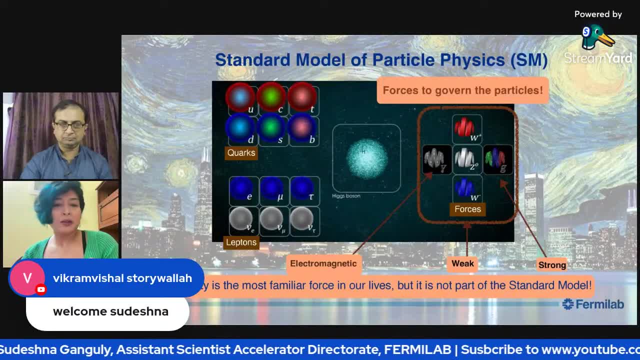 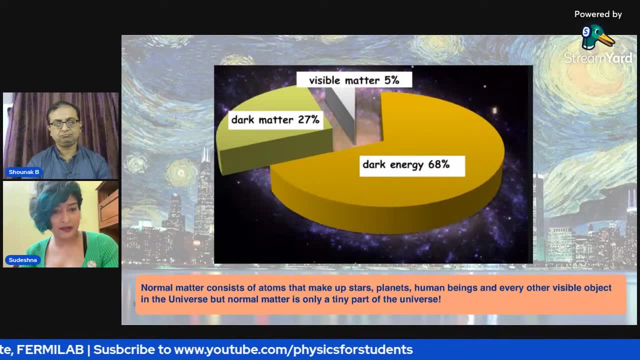 common. that is not part of standard model, right? so so then i i want to come to the next point. we are calling it very, very successful, the standard model, which is extremely successful, but then it is kind of annoying that it has been so successful. but it must be incomplete. it is not complete, right. 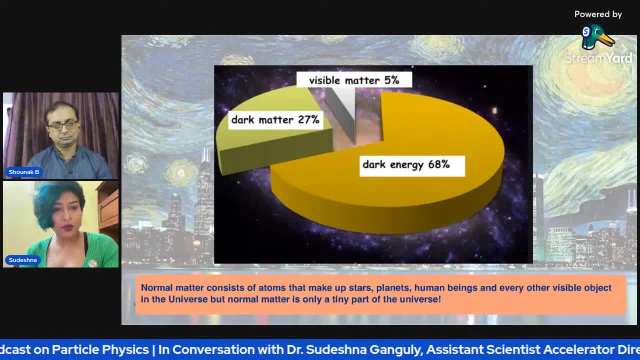 because there are still so many unanswered questions that we want to learn more about, like the why's, about, like why gravity is not complete, right, and so that's what we're going to talk about today is not part of standard model. and then the question of dark matter and dark energy. 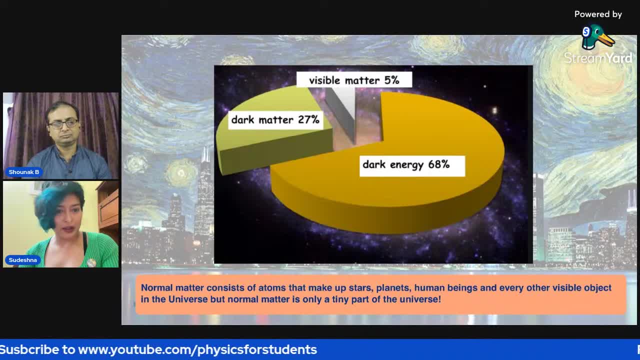 so standard model does not say anything about dark matter and dark energy, And the standard model only applies to the five percent of the matter and energy in the universe. so so the visible matter, that's just five percent, And it doesn't say, doesn't utter a word about dirt matter and and dark energy. right, so so for dark matter and dark energy, i just 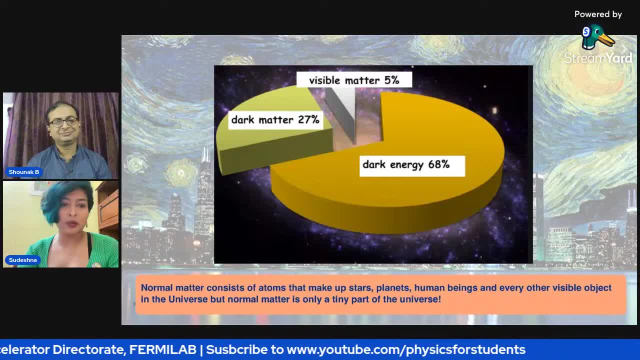 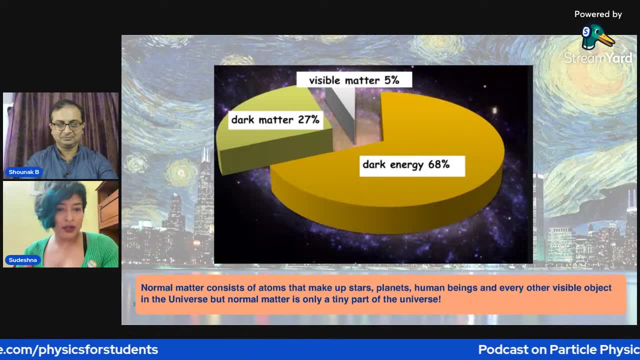 wanted to. Okay, again, this is not my area of expertise. I just wanted to briefly explain what I mean by dark matter and dark energy. So let's take the example of a spinning merry-go-round right in a playground. So when you are seeing it, looking at it from an outer edge, 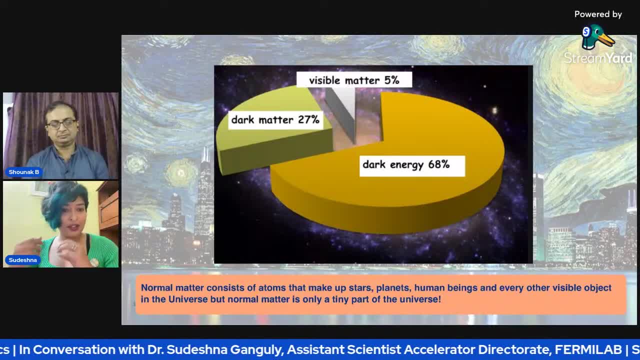 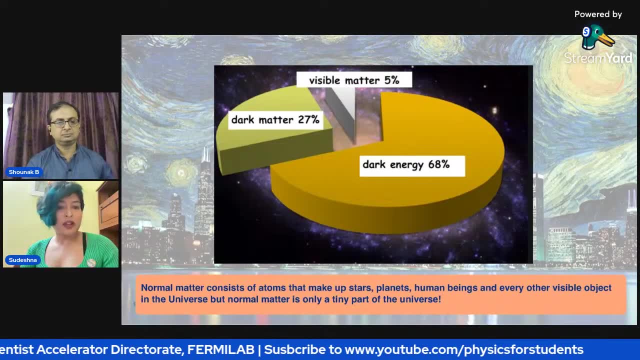 you'll see, the outer edge of the merry-go-round is spinning faster And, based on the things that you can see, like the seats, the pole, compared to those, the outer edge is spinning faster. So dark matter is like an invisible friend. 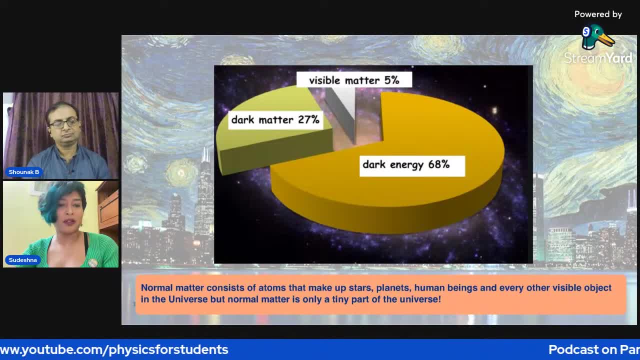 who is giving this extra weight to the spinning merry-go-round? So dark matter is this invisible friend sitting somewhere on the merry-go-round and giving extra weight For that? the merry-go-round is behaving that way that the edge is moving faster. 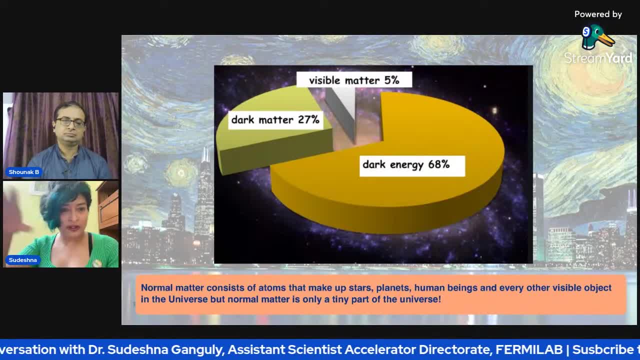 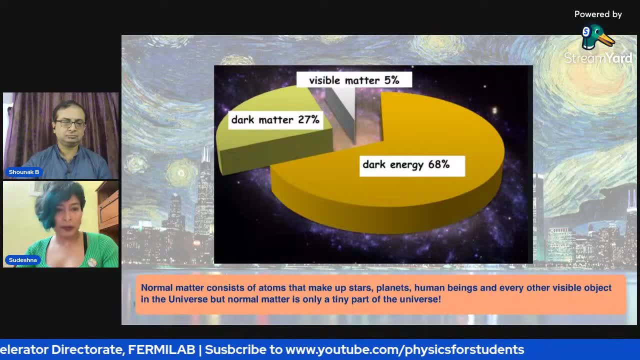 So imagine, the galaxies are like that, the merry-go-rounds, So the stars which are the edge of the galaxy. they are moving faster as compared to what we expect, right, What we expect compared to the visible matter. So scientists think that the dark matter 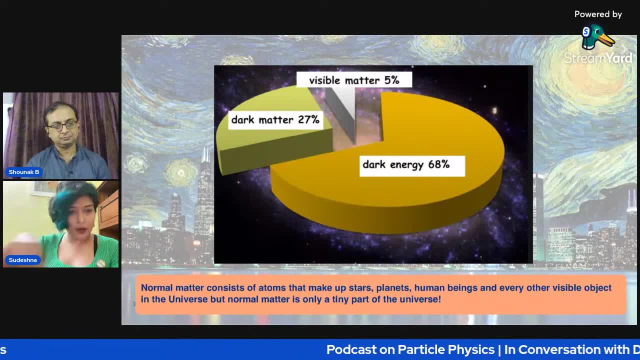 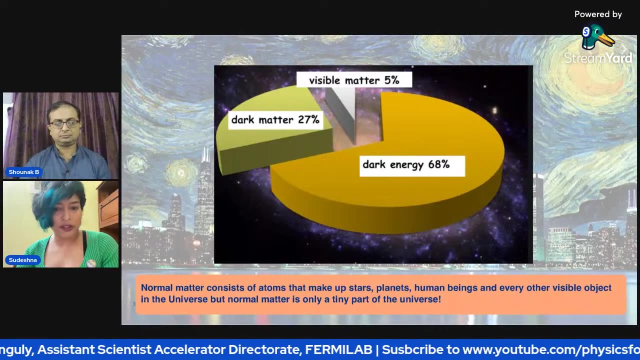 is this invisible friend who is causing these outer edge stars to move faster. So they're creating this extra gravitational pull to explain this movement. So again, so that is the hypothesis, but standard model does not say anything about that. So then, what are other examples? 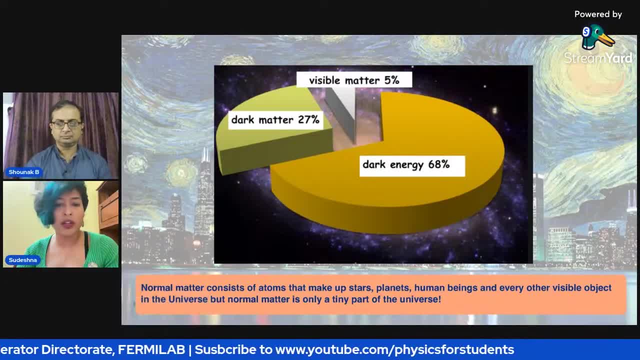 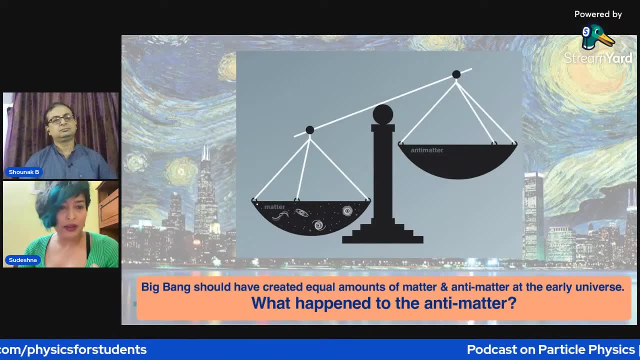 Like: how do we know that standard model is not incomplete? There are quite a few other examples, Like what happened to Antony, What happened to antimatter? Big Bang should have created equal amount of matter and antimatter, but if that happened, then we wouldn't be. we wouldn't exist. 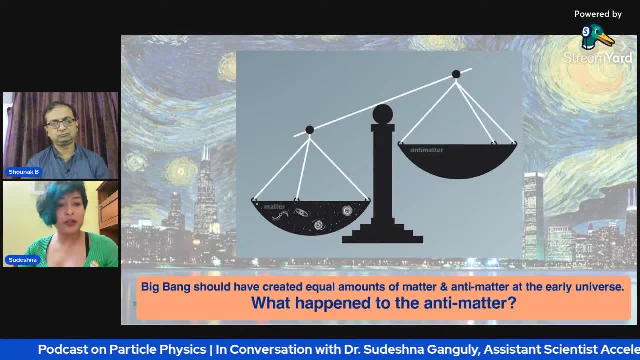 If equal amount of matter and antimatter happened, then everything would annihilate and we wouldn't be here, We wouldn't be talking today. So then, what happened to antimatter? We don't know. this answer, right, Neutrinos? that's something I'm quite interested in. 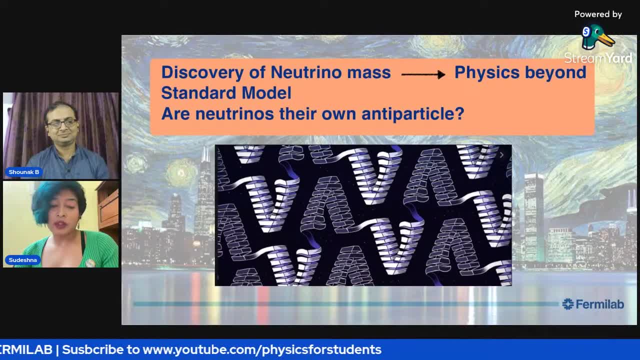 at this moment because I'm working on them. So the standard model predicted that neutrino are massless, but from recent experimental results we know, even though very tiny, they have masses. So then the open question is: are neutrinos their own antiparticles? 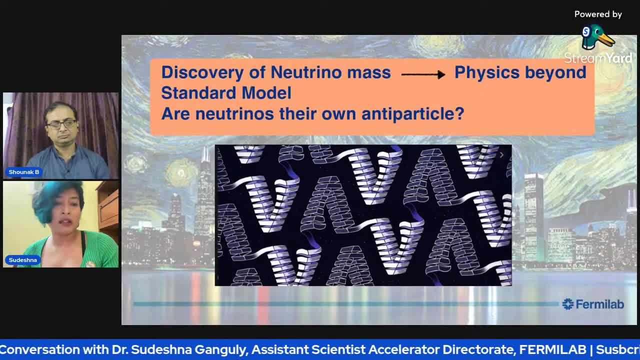 We don't know yet. We don't know yet Standard model does not tell us if neutrinos are their own antiparticles. So there are this outstanding question that standard model doesn't tell us. Just to interrupt you, doctor, I think neutrino is something. 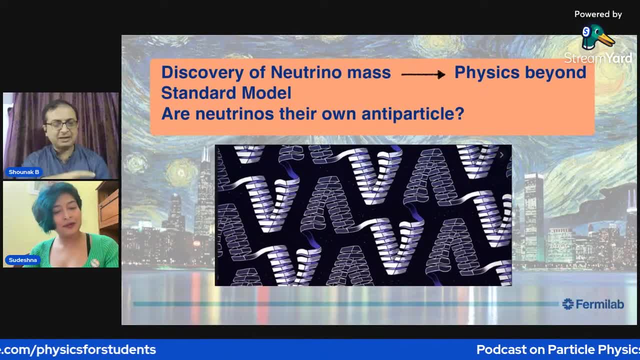 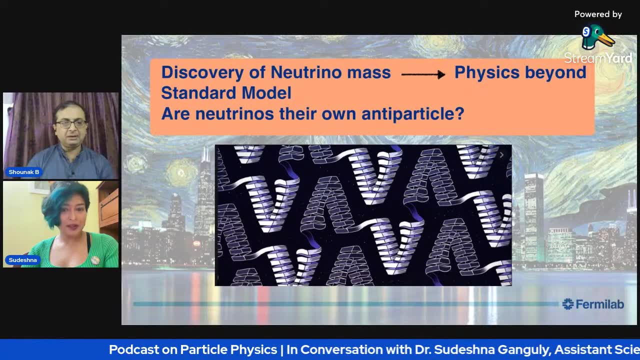 that a lot of research is going on in order to know, because standard model tells there is no mass, but experiments detect, and possibly we are going towards the theory of everything or maybe, which will help us to know a lot Exactly exactly. 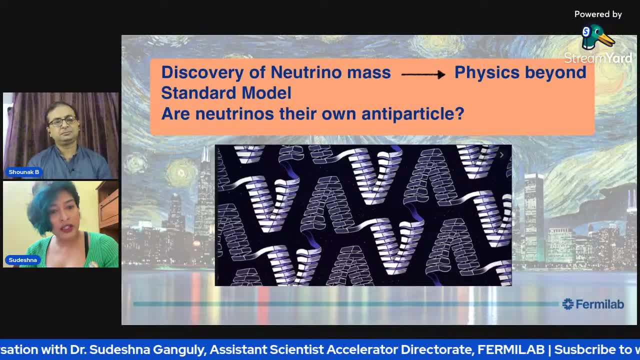 Neutrinos are? yeah, because they are so elusive, they are so tiny and they interact so rarely, so they're extremely hard to detect. But that's why, at Fermilab, neutrino science is extremely important at this stage, because it gives us an indirect way. 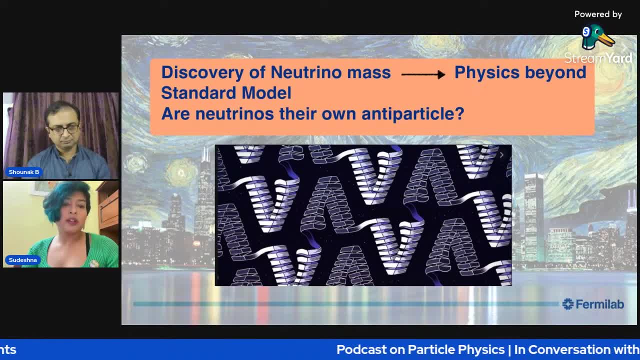 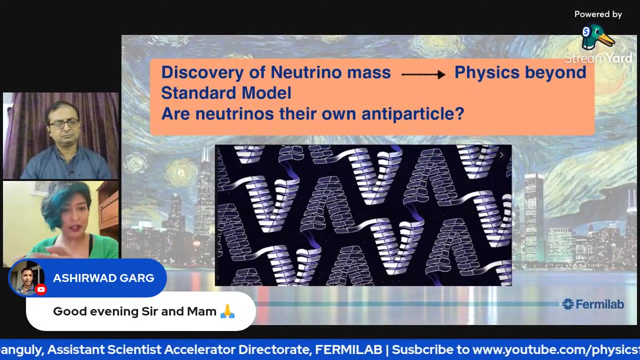 to look for physics beyond standard model. Because there are two different ways, and I'm going to talk about that in a bit: by going trying to create a high energy and try to look for new physics in that high energy range, Or we can look indirectly for new physics. 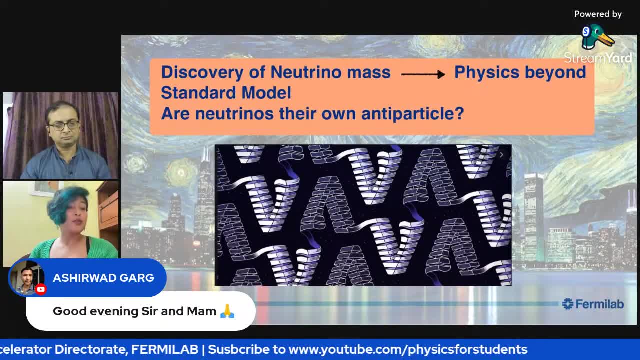 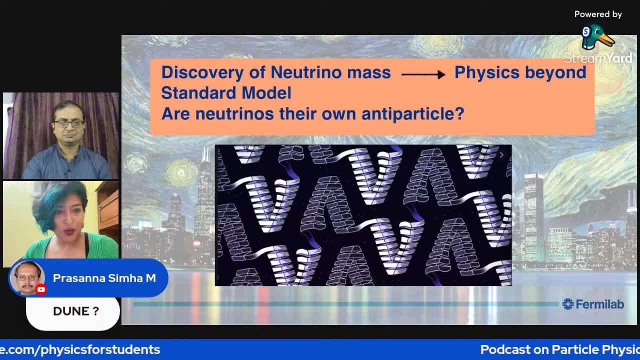 and neutrinos are a proof to do that. Neutrinos are new ones, so they're a really good proof to look for new physics. Yes, Dune- Yeah, I saw a question. Dune Dune will be upcoming. 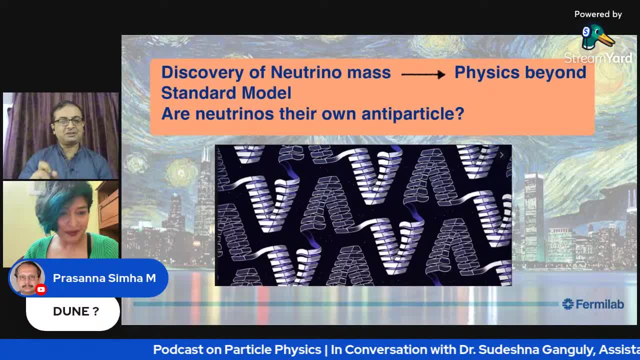 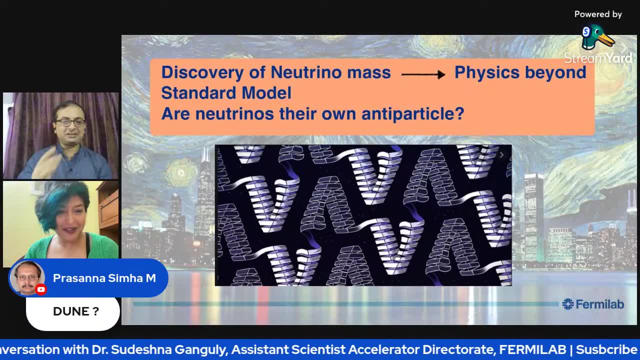 I would like to interfere here. Dr Prasanna Sinha M. he is basically a cardiologist and a surgeon, Yeah, And he came to my class yesterday and he asked me that. he told me that there are a lot of physics which is being used in cardiology. 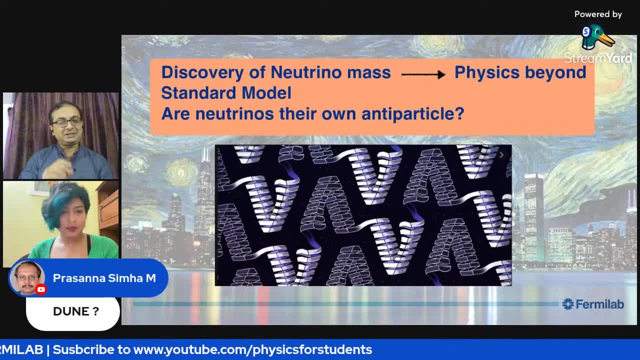 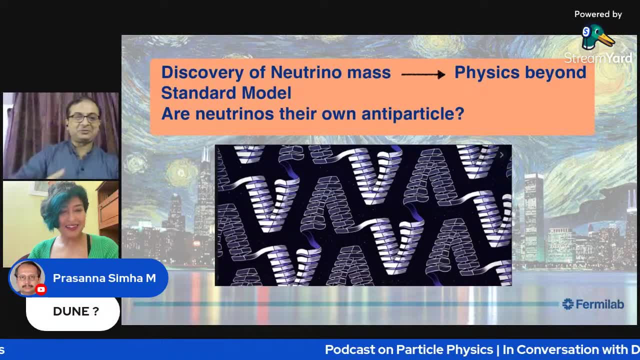 He is attending to some of my general relativity classes and he is a surgeon and a very famous cardiologist in one of the institutes. So welcome, doctor. Yeah, we have already got a list of questions, doctor, coming up, So you can just continue. 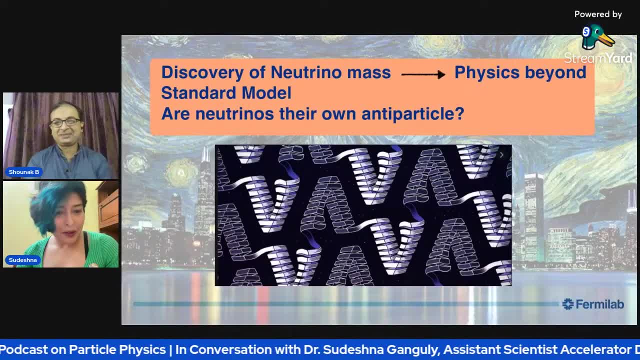 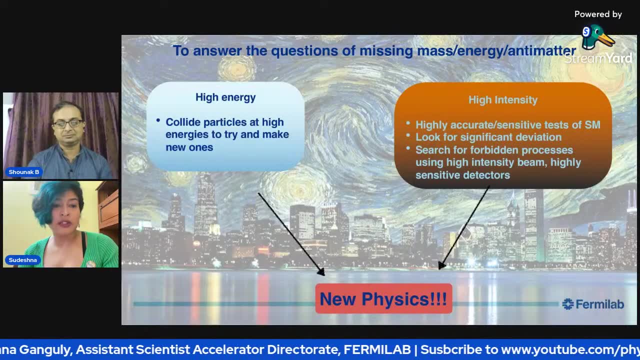 I will take one by one: Sure, sure, All right. So where were we? Yeah, So we were just setting the stage to show everyone that standard model has been extremely successful, but it is not complete And there is physics beyond standard model that we don't know yet and we want to know. 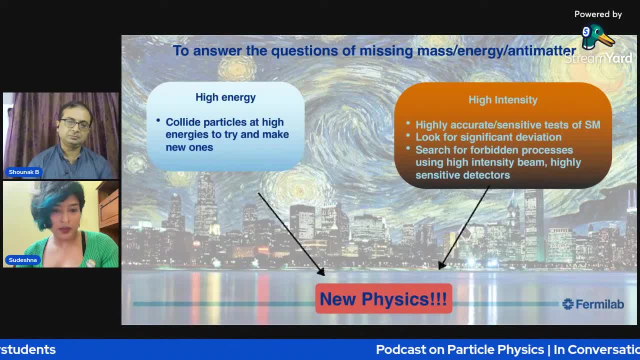 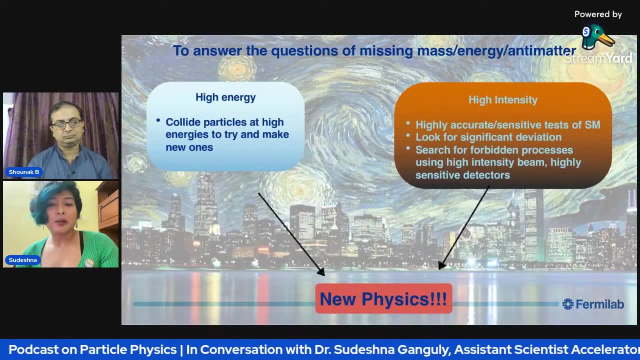 So that's why there are two different ways to look for new physics, right? So one is high energy and another is high intensity. So high energy. you have heard of elliptics. It is a very common phenomenon in the Great Collider, where the Higgs boson was discovered, right? 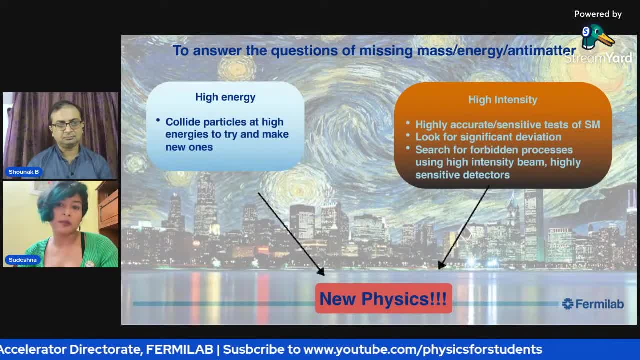 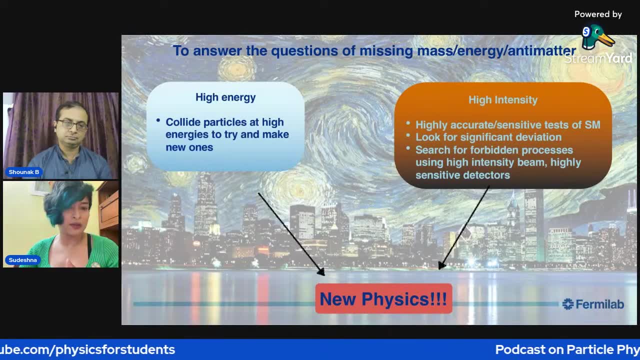 So they are searching furiously for new physics there as well. So if a new particle exists within their available energy, then it will just go bump in their data. So they will see a bump and discovery, And but that has to happen within their energy, available energy range, right? 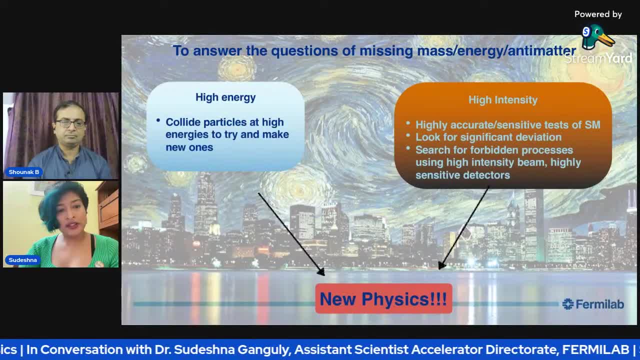 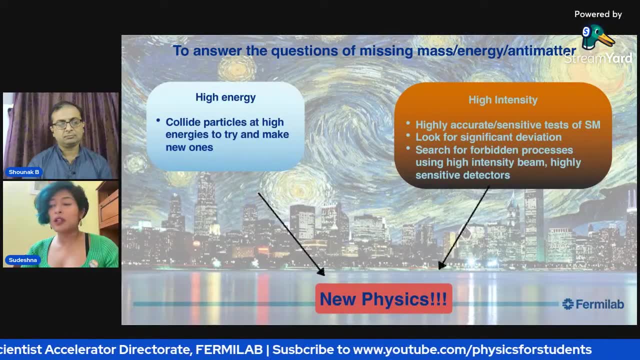 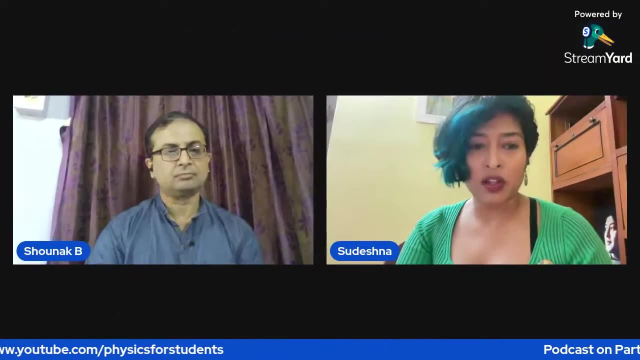 So the possibility is that where new energy exists could be far beyond their reach, The reach of LHC. So I want to give an analogy here. So suppose the reach of LHC is like a wall of a cell on your nail, Just one cell, wall of that one cell. 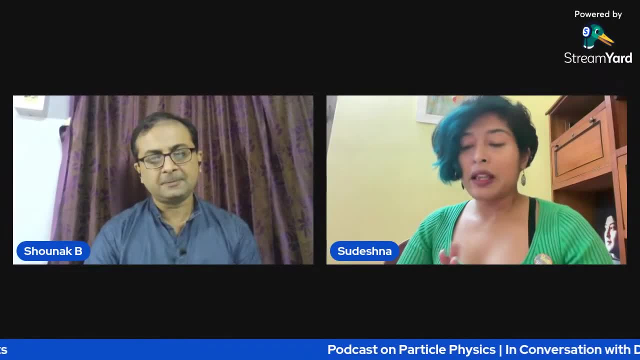 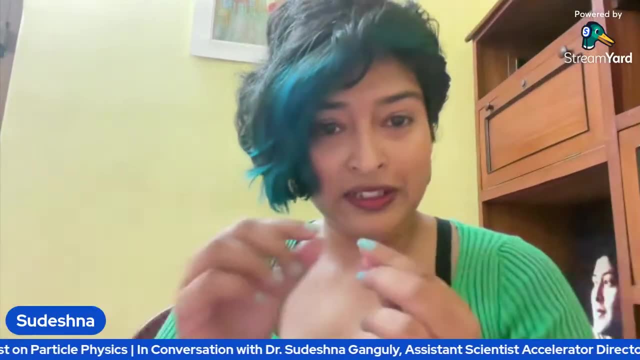 That's the reach of LHC. And then, where new physics can exist, could be the size of planet Earth. So you can imagine the discrepancy: the size of the wall of your nail: just one cell and planet Earth, right. So what is the new physics? 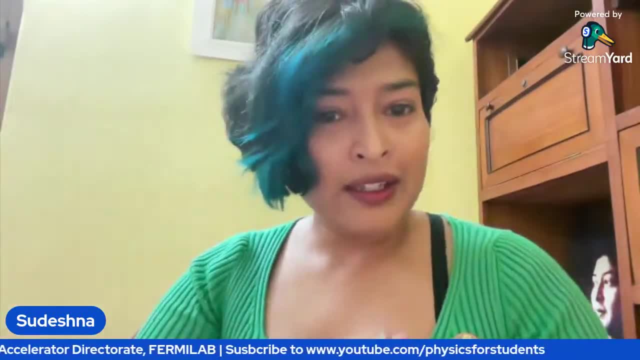 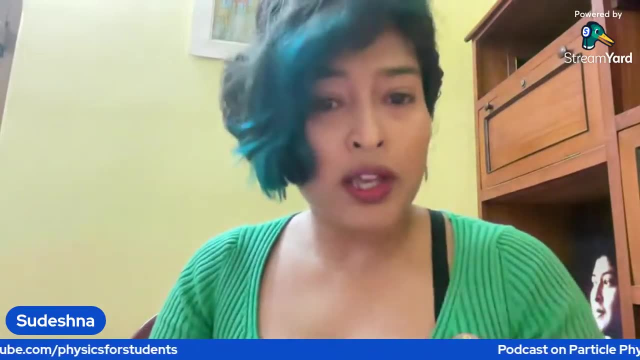 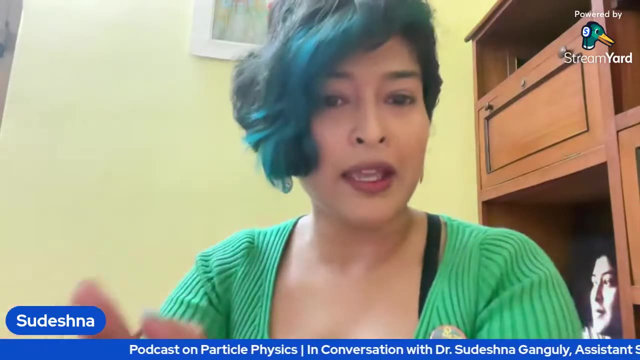 The new physics exists somewhere in between, say a car or a cat right. So if LHC is only able to measure like go as high as just a wall of a cell, it will still be not be able to find a cat or a car right. 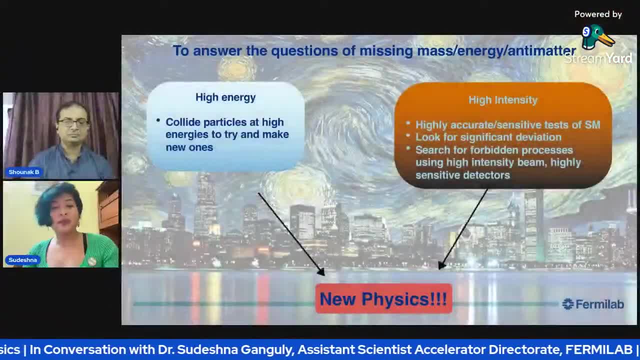 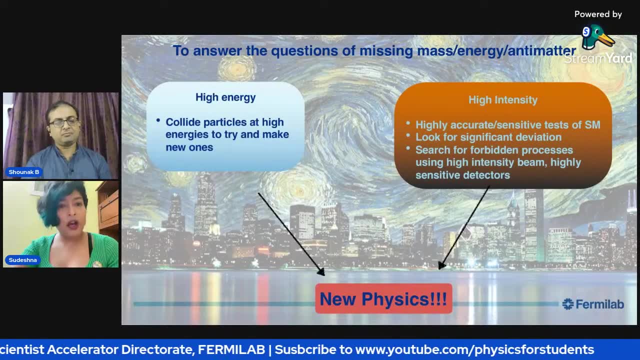 So that's when we need an indirect way to measure, like very high precision, high intensity measurements, where we indirectly try to look for this car Or the cat in this analogy. So that's why both of these ways, these methods, are important to look for new physics. 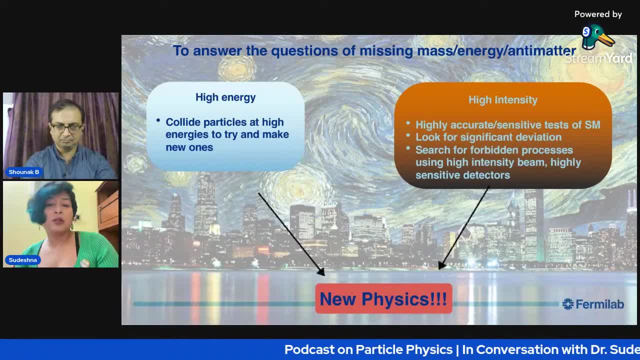 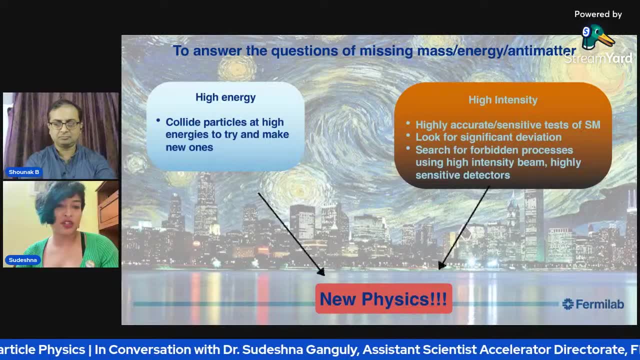 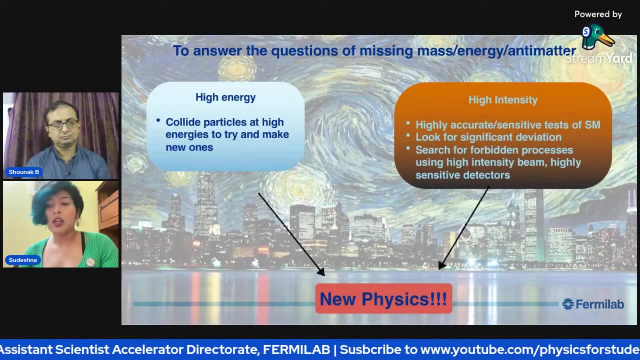 High energy, high intensity, high precision. So at Fermilab what we're trying to do is high precision. So even at low energy beam we can do very high precision, create more beam and make very high precision measurement, make very good sensitive detectors and make sure that the human errors are very, very limited. 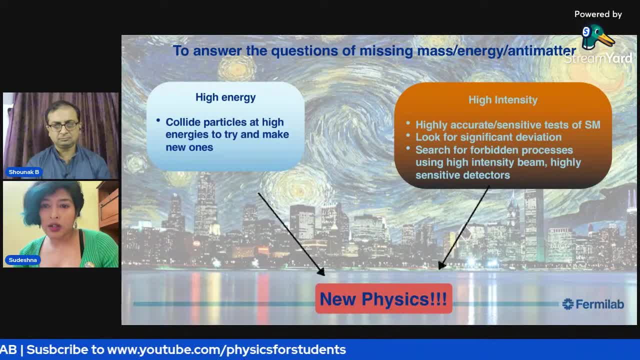 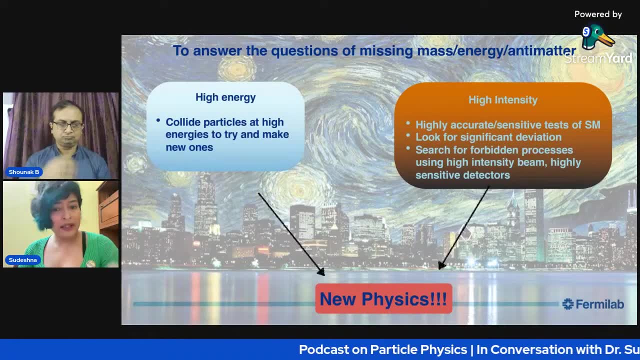 So that way we can look For new physics. So that's why I jotted down these pointers here on the slide, So so we can search for forbidden processes. So by that I mean standard model will tell us: no, it's not possible to see. you should not be able to see this special, rare process. 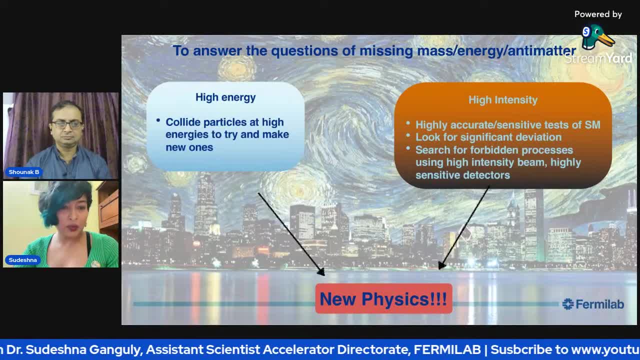 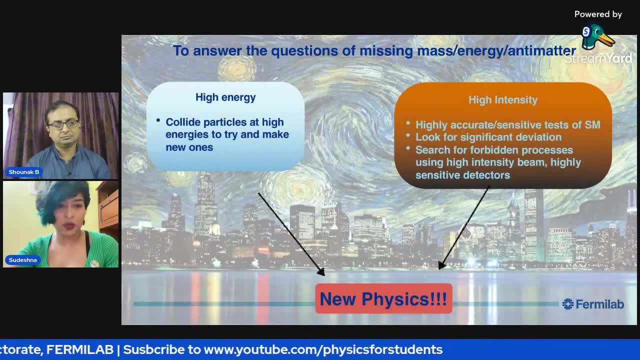 But if we see that just one such event, then we can. we can prove that new physics exist. And then theorists will have to come in and have to hypothesize: was what caused this, this new process for your process? Or it could be A parameter value, like the G minus two experiment. 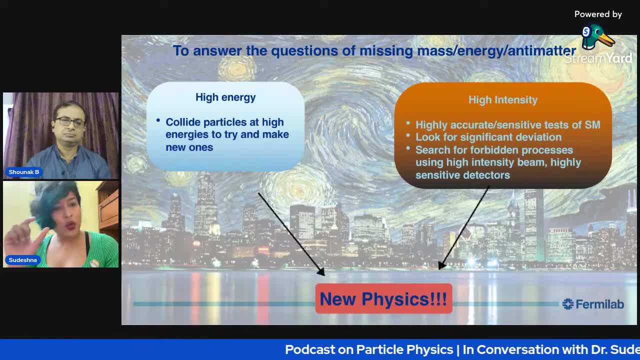 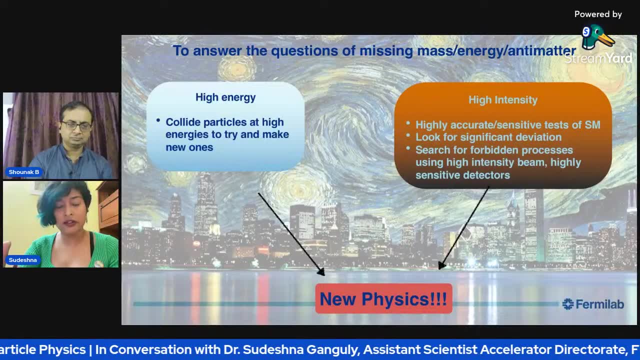 I will. I will talk about it in a bit of a particular. just one value, Right? So we measure it as a value, as something, and theory predicts is something else. So what's causing this discrepancy? So there there could lie the new physics. 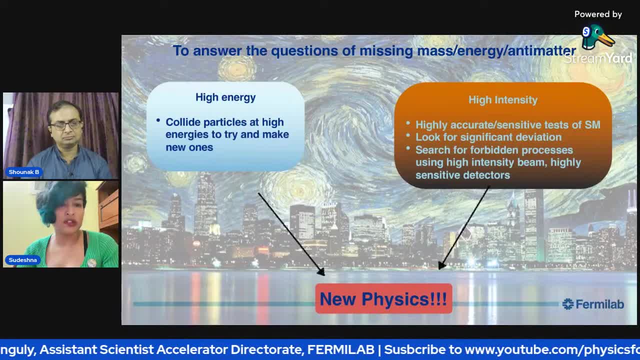 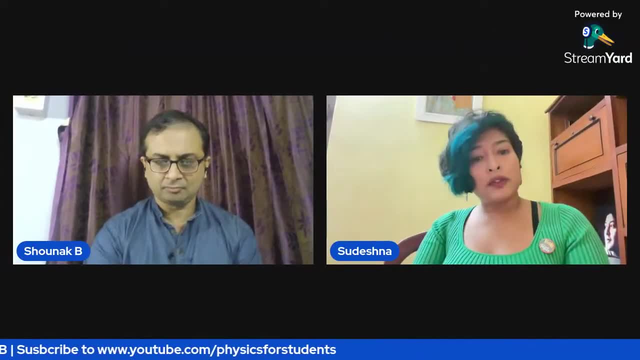 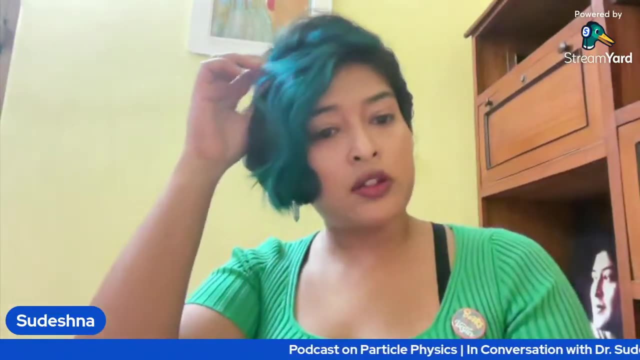 So that's why it's so exciting that it gives us access to new physics very easily. Right, There are both ways, And Fermilab actually is involved in both. So even though the high energy is actually happening In CERN- but Fermilab has a very active collaboration with CERN- 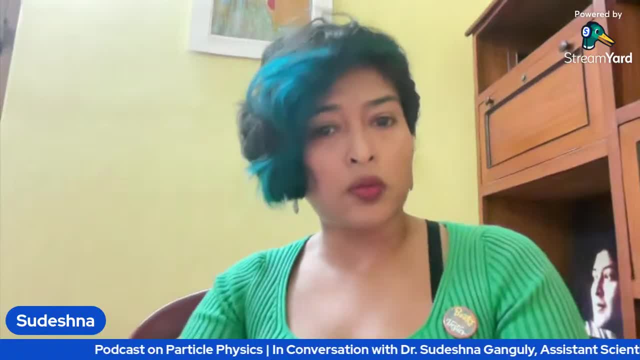 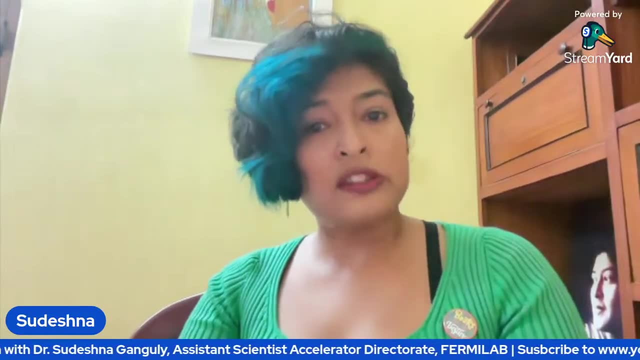 So there is a big collaboration of US scientists to work with our CERN colleagues on the high energy frontier, And then in the intensity frontier, we have neutrino physics, we have muon physics, So I think we can go to the next slide. 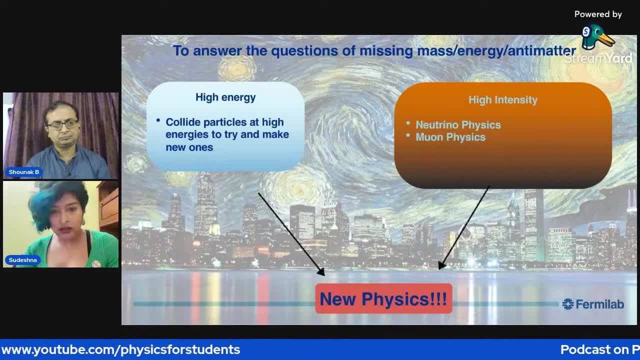 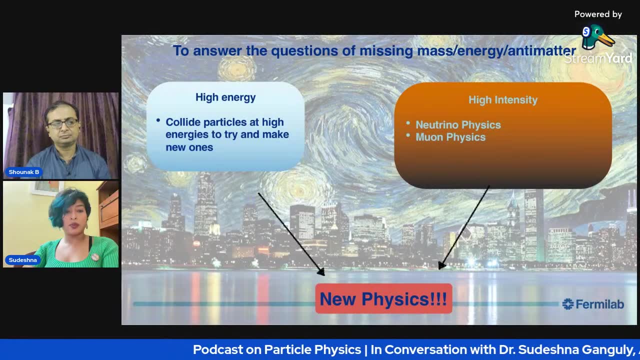 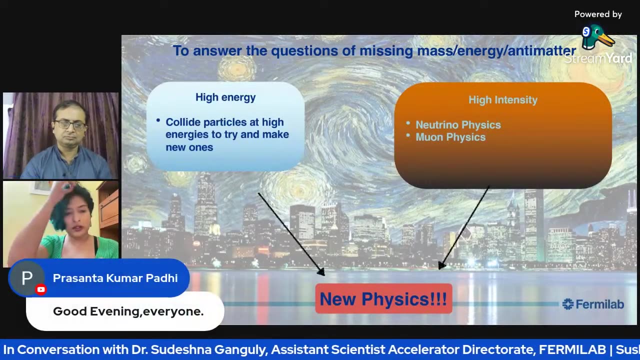 Yeah, so that's. that's what. I am Sorry It's here. Yeah, So. so neutrino and muon physics are the two Most important active, like beam and facilities of Fermilab. But we do have an active collaboration on CMS to work with our CERN colleagues. 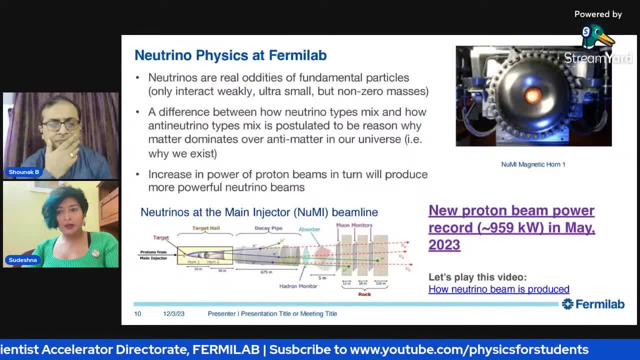 So neutrino physics, So, so, So. somebody mentioned DUNE already. DUNE is what is upcoming. We do already have an existing neutrino facility at the lab which is called NUMI neutrinos at the main injector. So NUMI is basically the prototype of 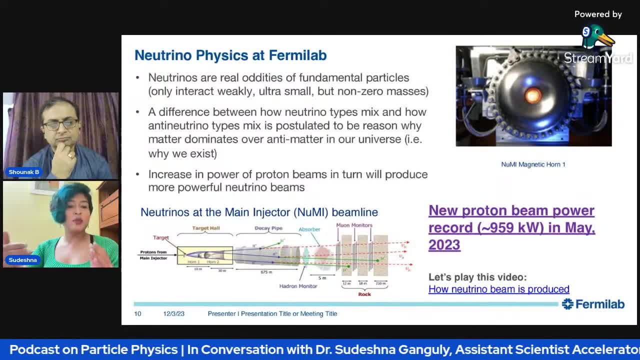 What DUNE will become just bigger, better. but NUMI is already giving us valuable lessons, and like all the beam lines. So so when we just talk about these theories and these hypotheses, we don't talk about the experimental side at all. So I'm an experimentalist, so we don't really appreciate the details, like how much details would go into just building a beam line, extracting the beam, putting it onto targets, like building the target itself. 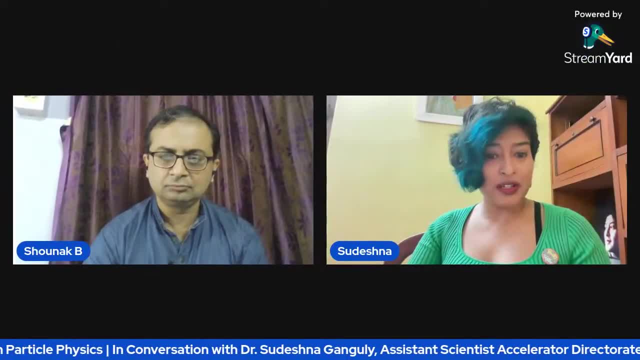 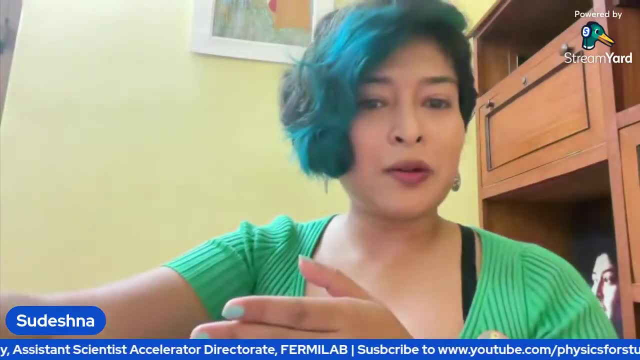 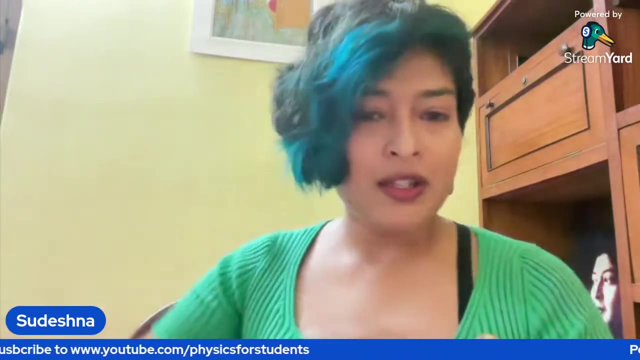 That's like a different division, The material science, and just to just to create the target and then getting the beam out of the target, focusing it, sending it down some decay pipe, sending it then farther down underneath, 600 miles or more, to a fire detector. 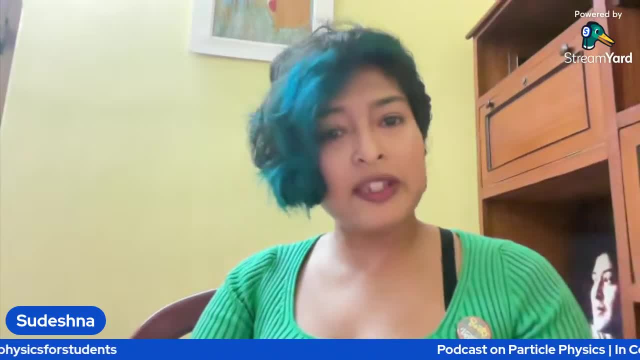 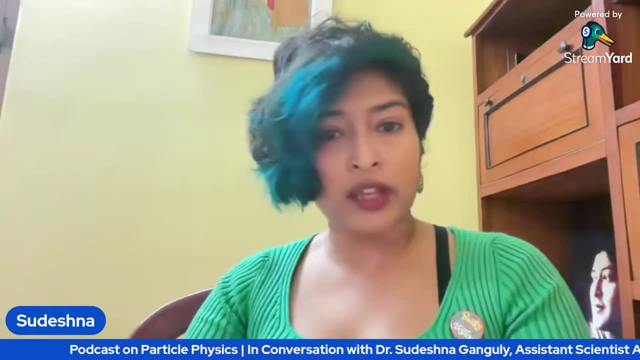 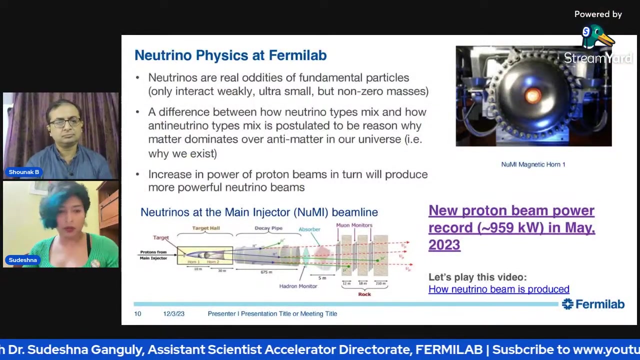 So so all these like experimental steps. they're extremely complicated and it requires lots and lots of collaboration with scientists, graduate students, postdocs, engineers, many, many people. So it's Like a massive, massive work every day, like every step put together. then finally we probably find one answer. 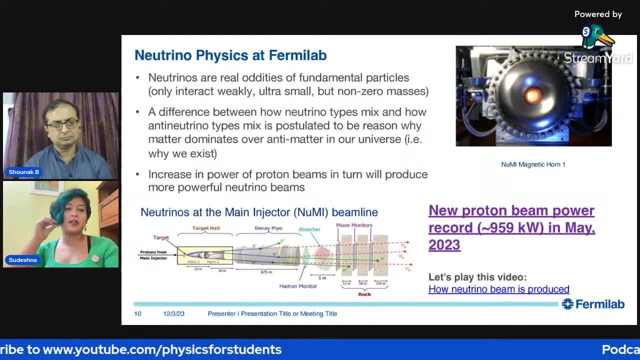 So that's what's, that's the beauty of it, That's the, that's the interesting part of this work, that day to day you're just working on a tiny specific subset, But when you put it together, then you can. you can you just realize suddenly: oh yeah, so this is almost spiritual. 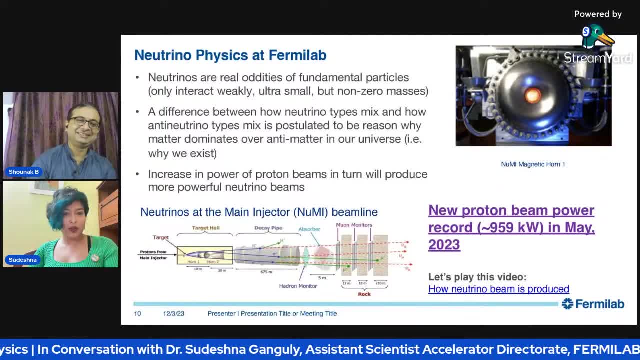 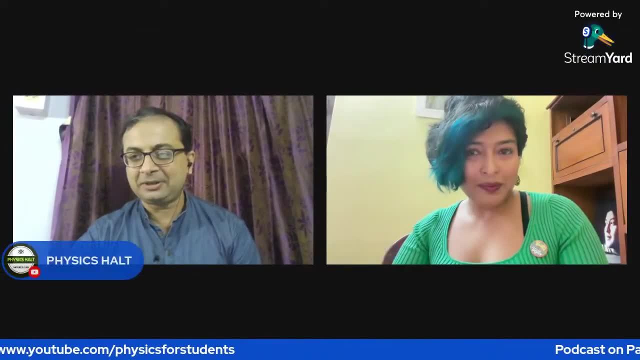 We are doing it for the spiritual reason. We're trying to find these amazing questions and answers, Right? So Yeah, Are there any questions? There are a lot. OK, Just remove your, with your permission, this slide, And first of all the thing is coming up, is from physics, halt. 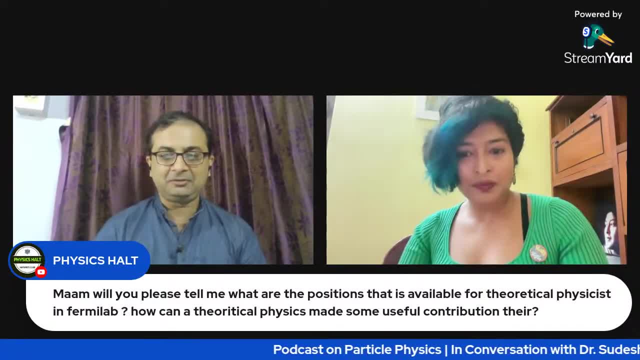 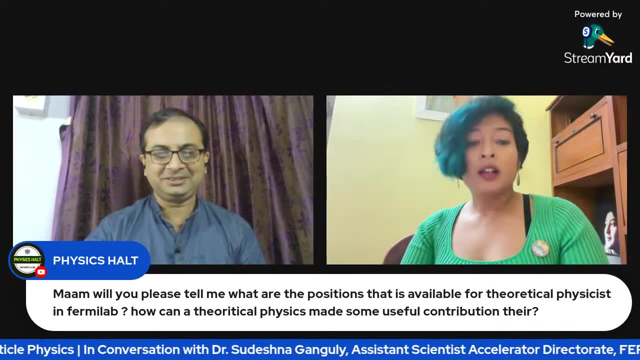 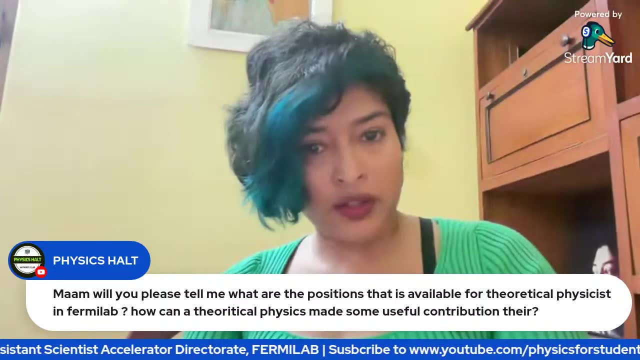 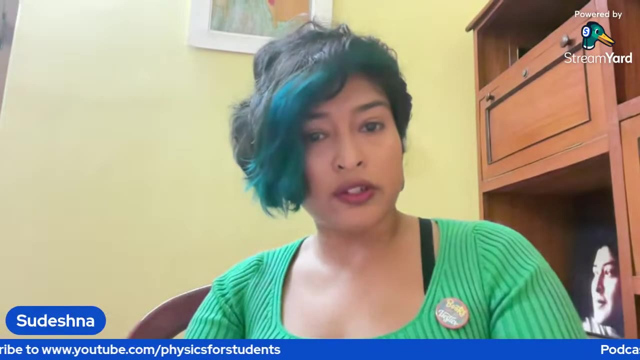 Ma'am, will you please tell me what are the positions that is available for theoretical physicists in Fermilab? How can a theoretical physics made some useful contribution there? Yeah, So so well, the positions there would be. There are three different ways to work as a theorist, theoretical physicist, from a lab- if you're a grad student and you are working for an university who has any collaboration with any from a lab experiment. 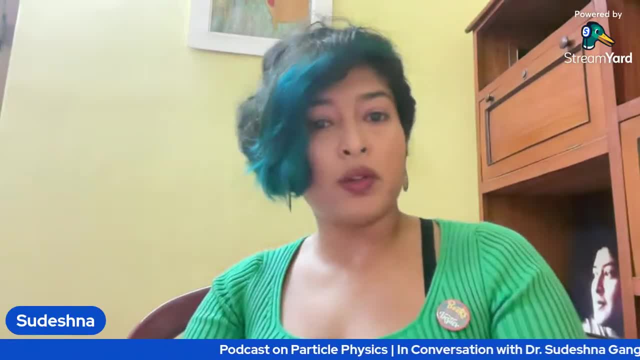 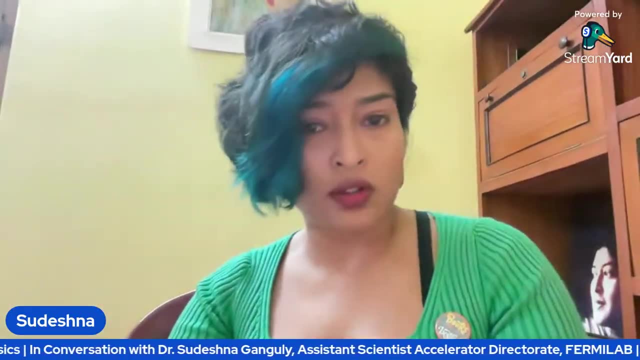 It could be me on physics related theory. It could be neutrino physics related theory. It could be astro- We also have a very strong astro astronomy department and my theories of that. So you could come in as a grad student, You could come in as a postdoctoral researcher or you could join. 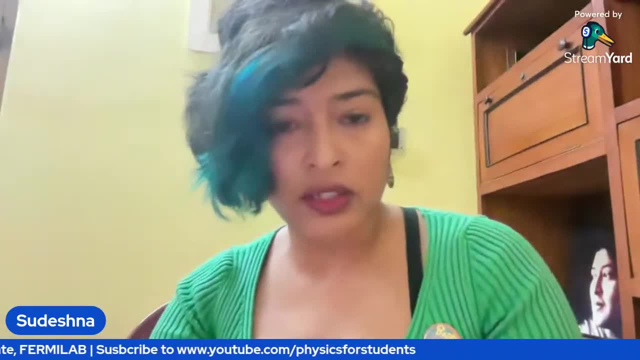 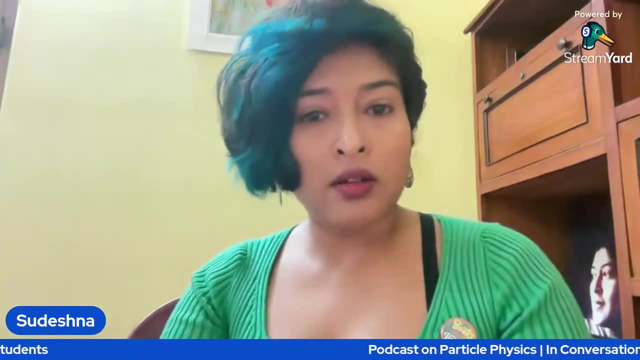 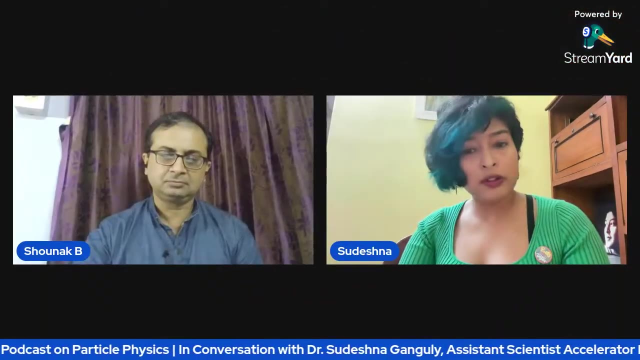 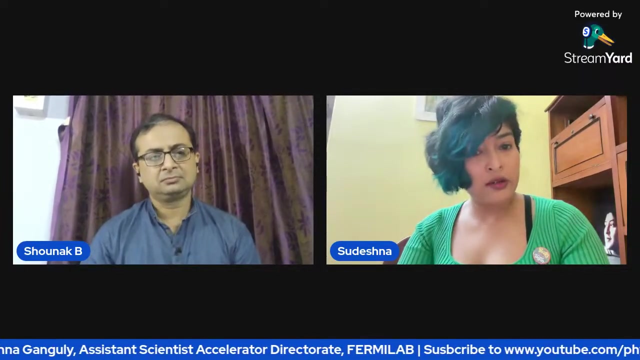 As an associate scientist or application physicist. There are all those different positions as well. So, depending on where, what stage of your career you are in, there are mainly these three different ways you can come in and for contributions. So so, yeah, So you can, again, depending on your interest. you can go to astro, you can go to neutrino science, you can go to me on. 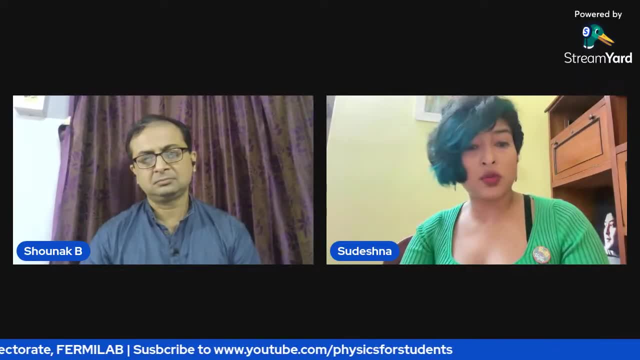 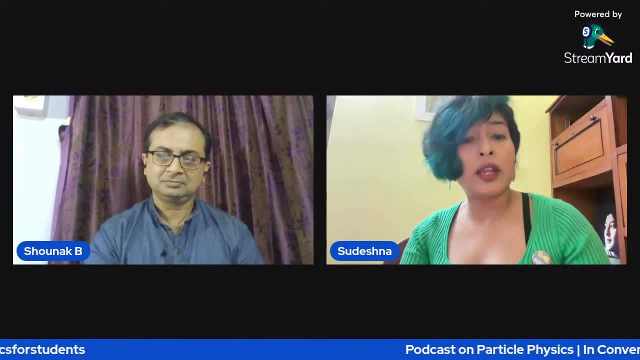 So right now, for me, I'm quite excited because- G-minus- We have just published our second front two and three data recently and there's a lot of work in the theory front for that. So, yeah, So there is a lot there that you can contribute to. 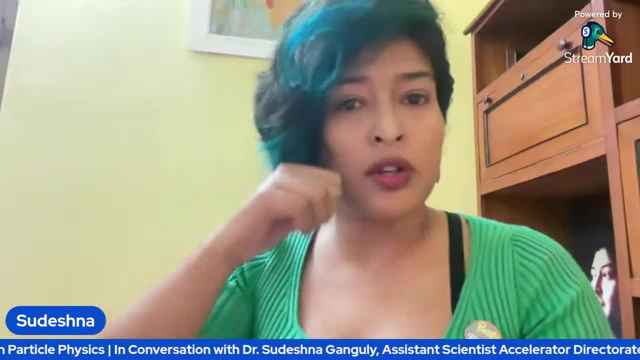 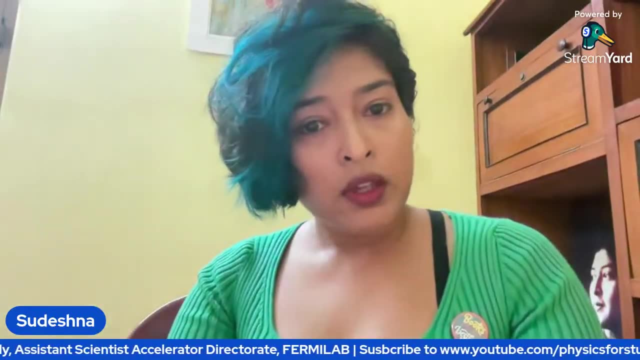 If you're interested in that, For neutrino dune is upcoming so we need our theory colleagues to keep up and also working with us together. So these are a few ways you can come in And if you are interested, always like, you will have my email id. 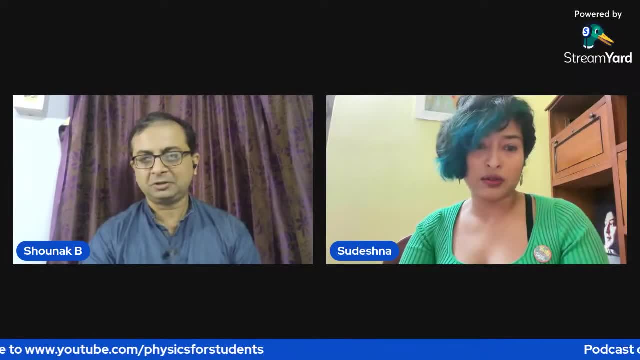 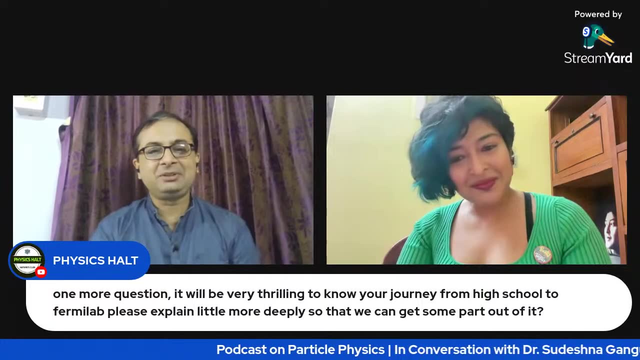 Just hook me up with people and I will try to help as much. Sure, sure. Next is to the same person. I was also willing to ask this to you. One more question: It will be thrilling to know your journey from high school to Fermilab, Please. 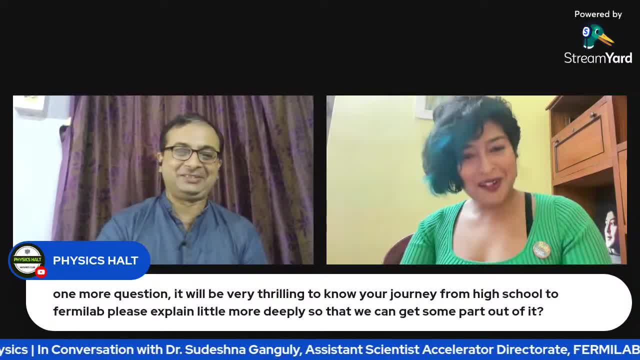 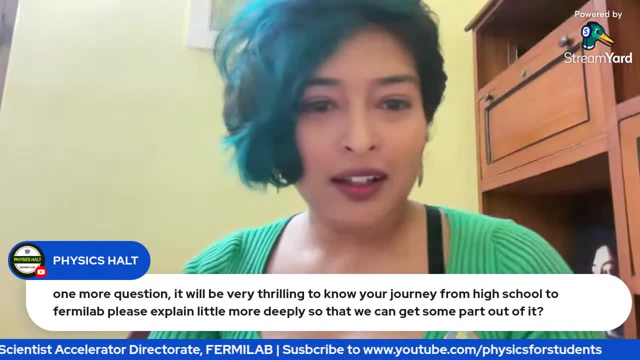 explain a little more deeply so that we can get some part of it. Sure, Well, I mean so I am from this tiny- maybe not tiny- a suburb of Kolkata, Hinmotor. I'm there right now. I'm at my parents'. 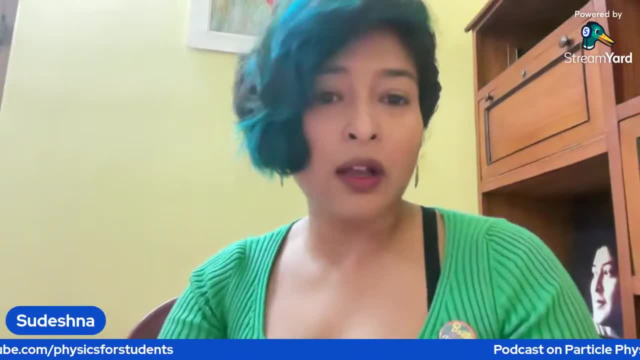 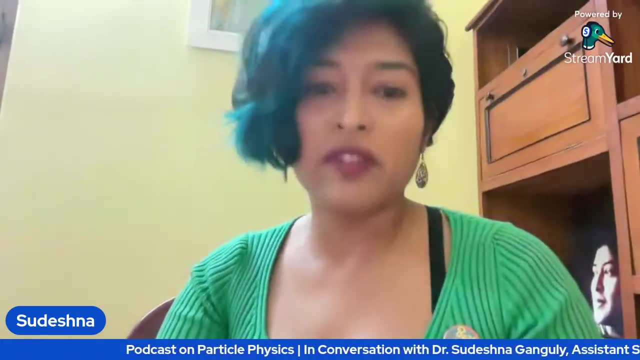 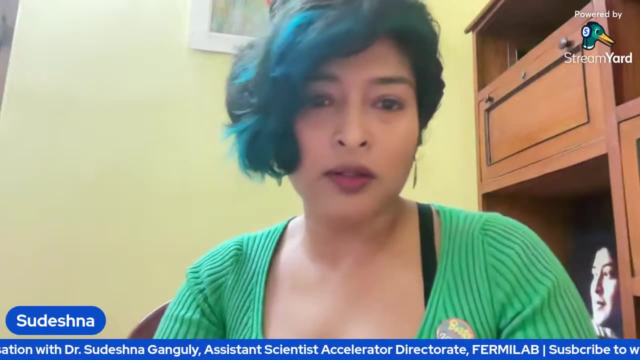 house. I went to a local high school, Bengali medium. but I was always interested in science as well, in literature and history. I liked all but physics the most right. So yeah, so I just did physics, just studied hard, got good grades et cetera, et cetera, all the exams. Then I went. 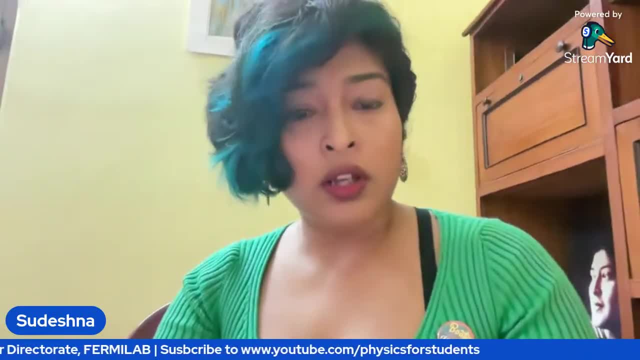 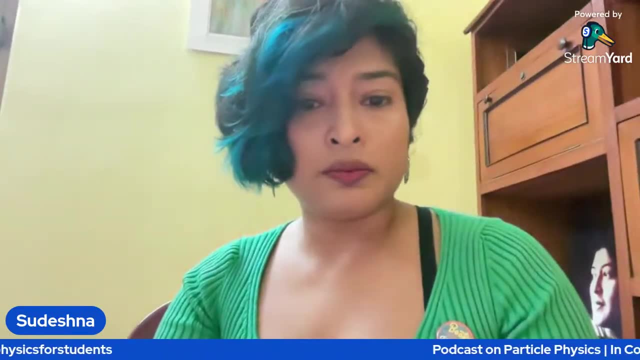 to Bethune College And again at this stage, I did not know that I would do particle physics. I had no idea about particle physics, to be honest. So I went to Bethune College, did our basic honors in physics, did the basic courses, 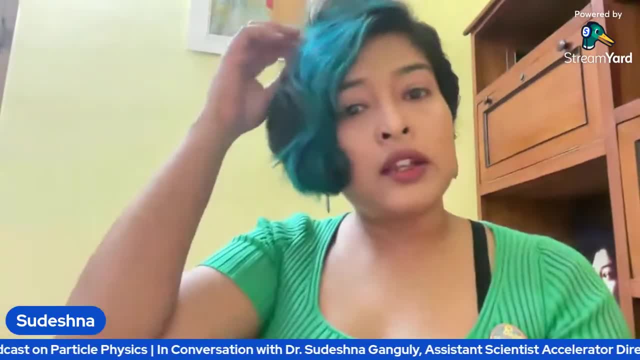 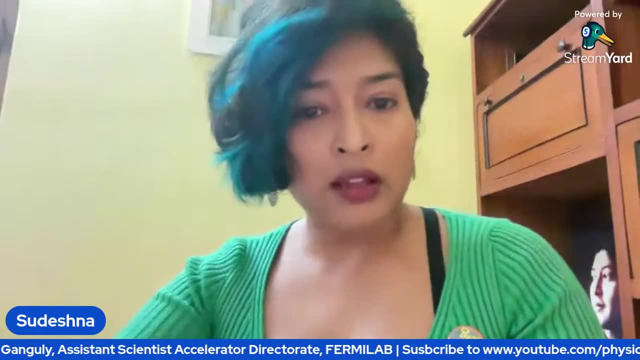 afternoons: classical mechanics, quantum, et cetera, et cetera. And then at that time, when I was in Bethune College, I was interested in going somewhere outside of West Bengal and trying something else, somewhere else, just to gain more experience and exposure. So I was. 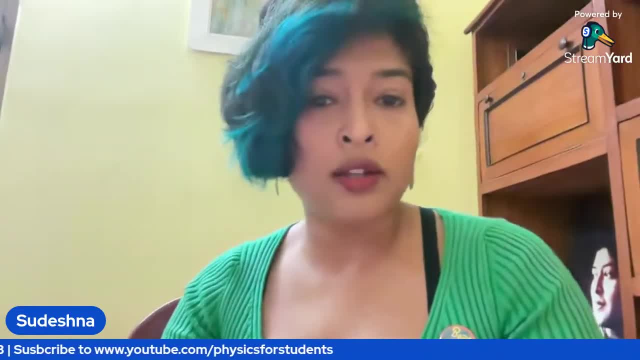 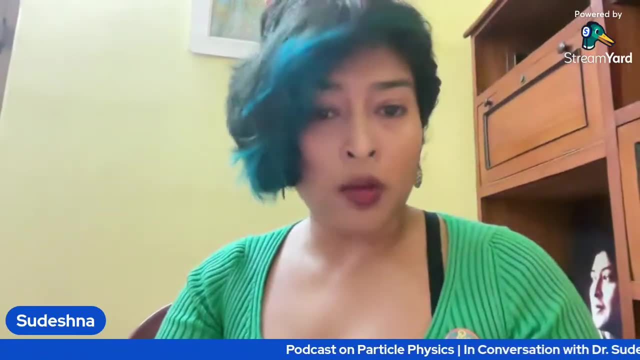 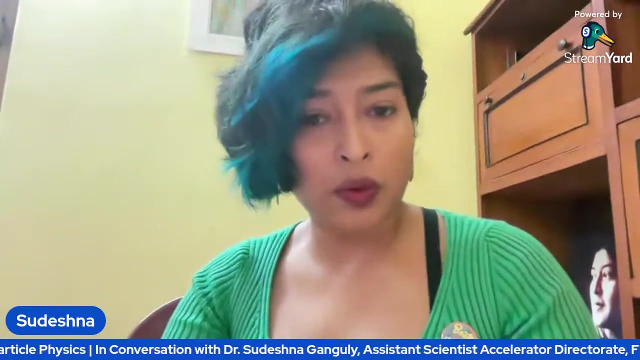 taking these entrances, different entrances, and I got into the program for master's in IIT Delhi- Now IIT Delhi is famous for optics and electronics. but then there was only one professor in our department who would do particle physics And I happened to take a course with her and I really 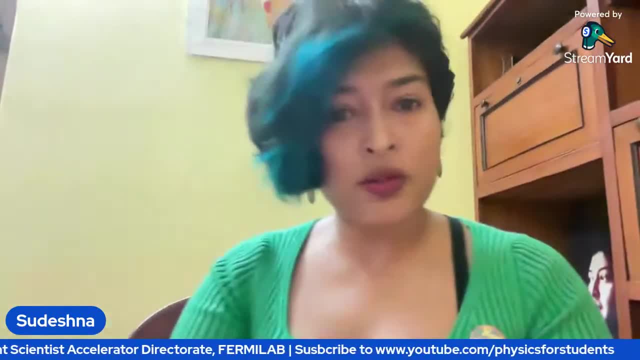 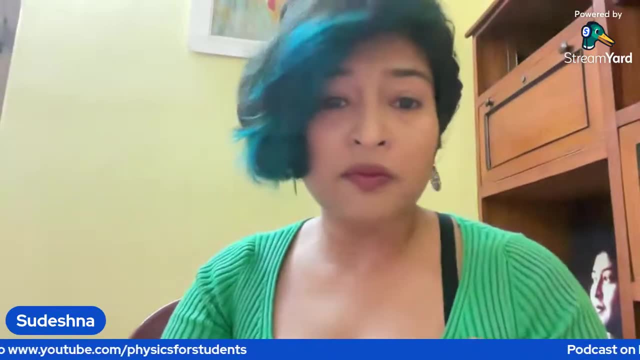 really loved it, Just loved it, Just spoke to me. It seemed a little bit like detective work to me, like finding all these mysteries, And for the same reason I'm interested in history. it's like detective work in the ancient world And this is a different sort of detective. 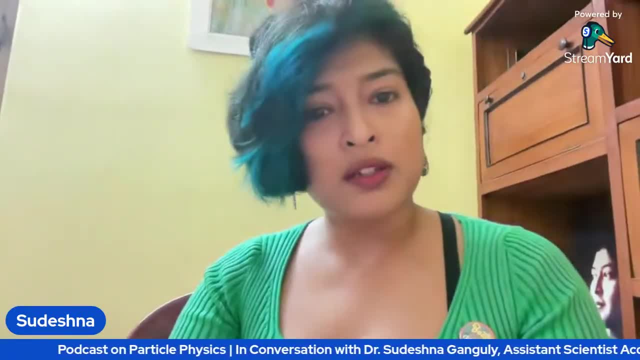 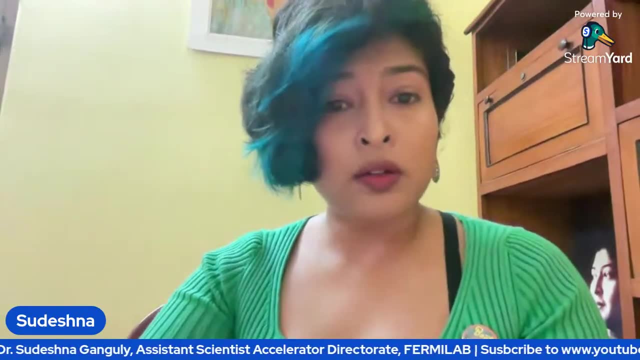 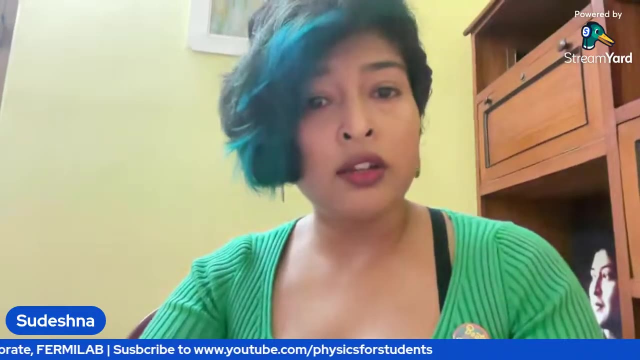 work, So yeah, So I liked particle physics very much, Got my master's from IIT. At the same time, I learned about from my fellow friends that there are many universities in the US where we can apply, We can take GRE, And at that time we had to take GRE. subject: GRE and TOEFL. 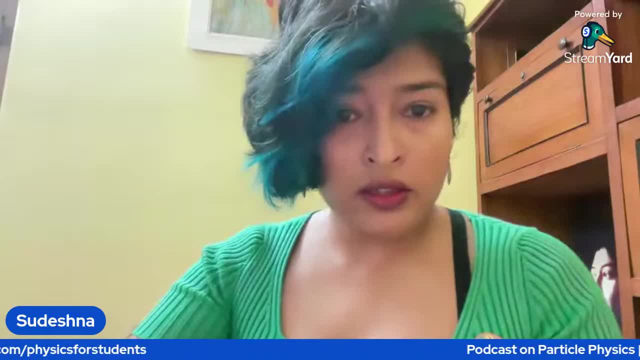 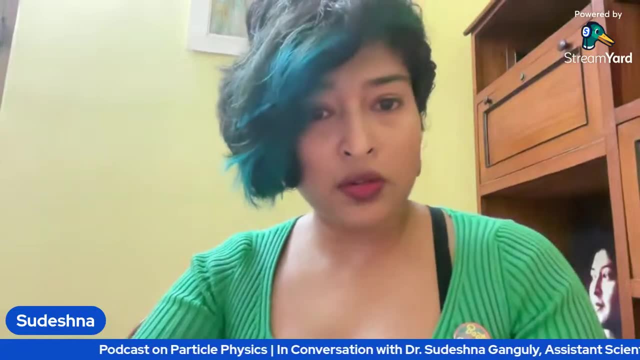 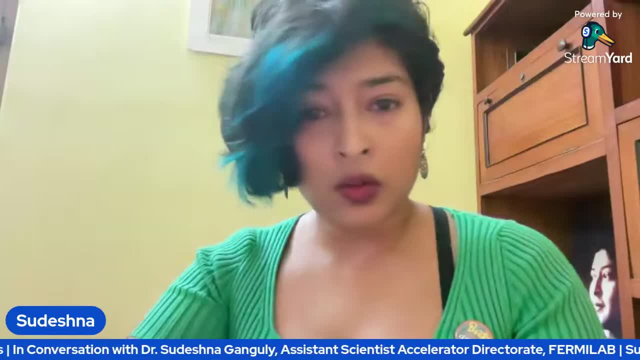 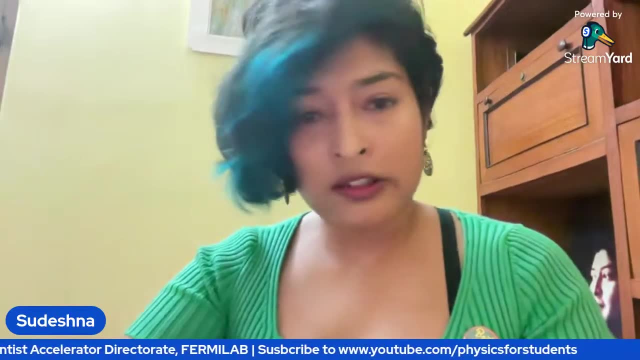 schöne Arbeit. they tell the story of these great foundations. who did hardcore particle physics and collaborated with these famous collaborations like Bell, KEandro, Cucull, CERN, Fermilab? So once you get into such university, it doesn't matter which university you're. 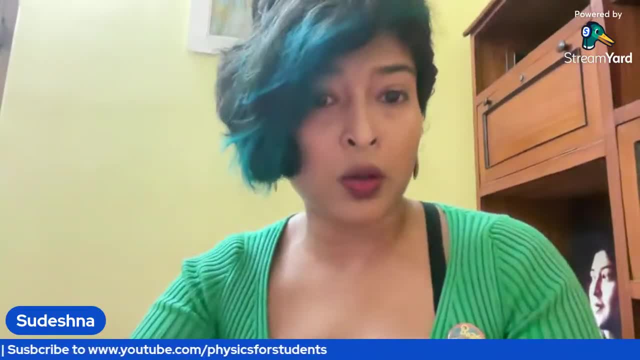 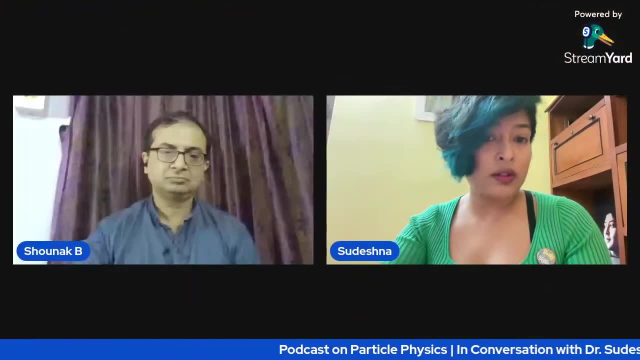 in The collaboration you're part of the collaboration and the quality of work that matters So. so that's how I got So. in doing my PhD I was working for the exceloratory in KE and in Japan And then I got a postdoc And then I got to Fermilab worked on G-93F. 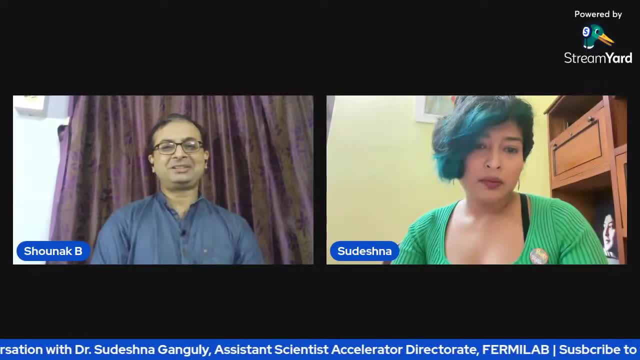 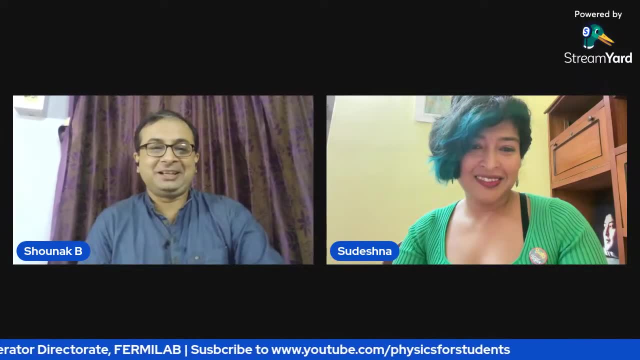 too. so that was my journey. basically, thank you very much. i think, uh, physics, all you asked everybody's question and i was also willing. i was feeling a little bit, you know, uh, you know, i would say i'm a little bit skeptic, but what would dr ganguly think if i ask a little bit personal? 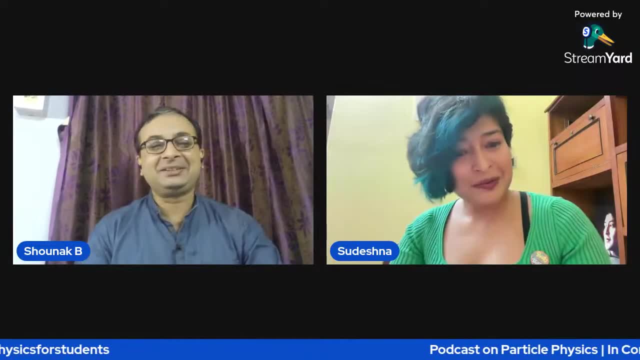 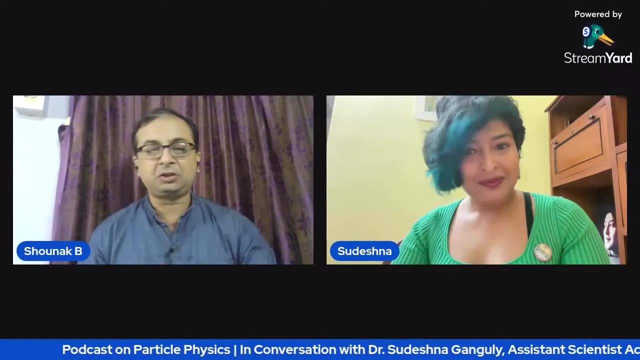 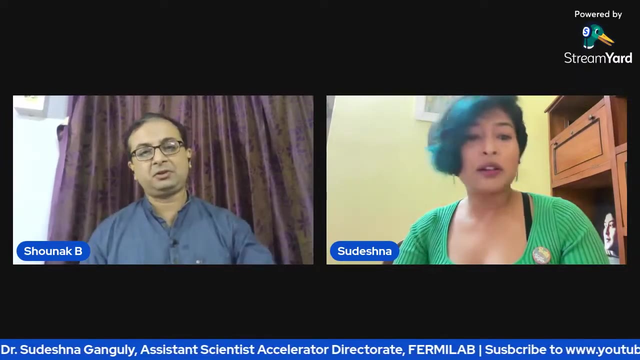 question? absolutely, but this is a wonderful thing. so you know, i think everybody is watching. today already 25 people were watching. this is a kind of a motivation which takes us. that means vernacular, medium or in medium, actually doesn't matter, it is the passion at all. yeah, so something. 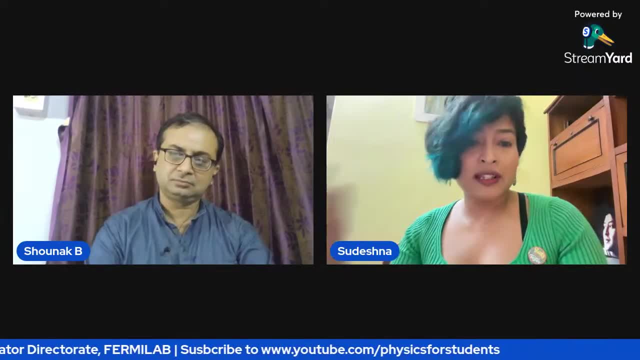 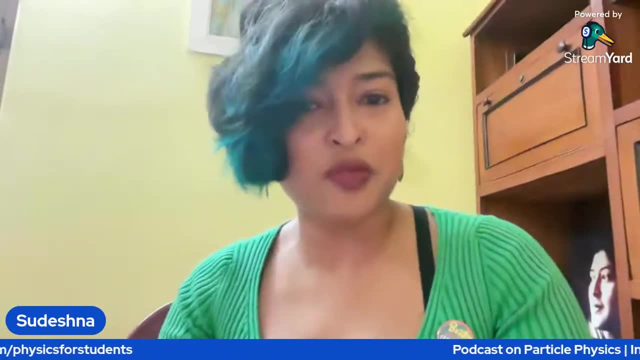 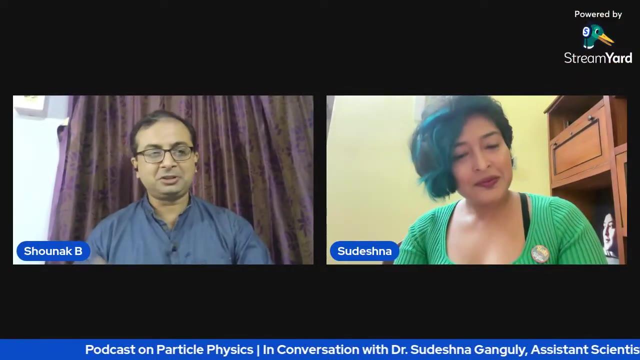 i picked up um when i was in us. just listening and just interacting with people just helps you. it's just another language. so just learning another language by listening and talking more, that's it absolutely. i often tell that you need to to all my subscribers who are just like my. 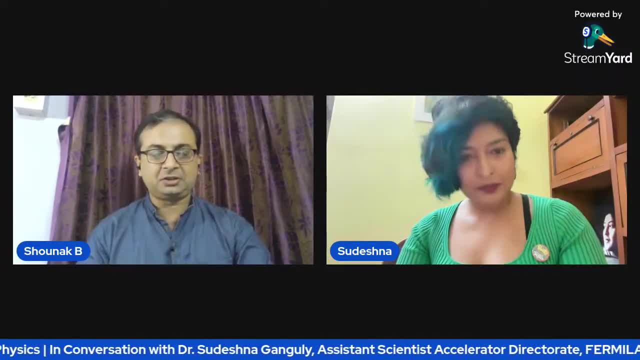 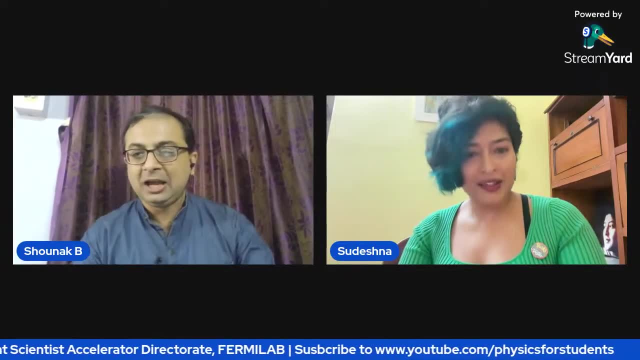 children, that communication is something, whatever the level of physics you know, if you are unable to communicate, not in an any kind of an american or british accent, but you need to actually communicate. uh, dr ganguly, we have got another question a little bit technical, coming up from vikram vishal. 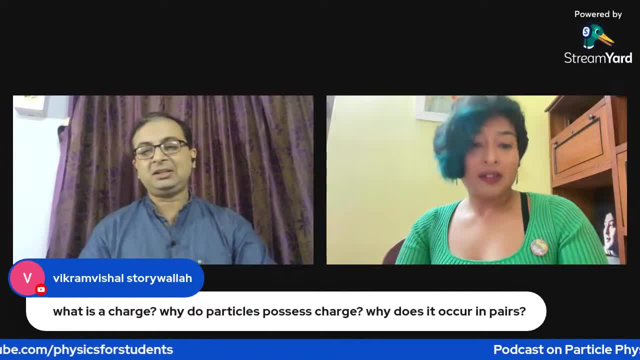 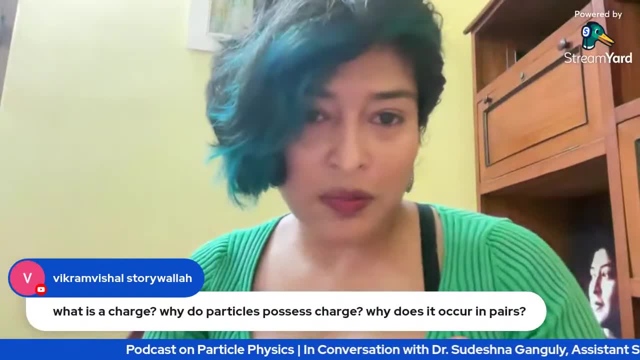 what is charge? why do particles put this charge and why does it occur in peers? so yeah, so this is a fundamental property, right? uh, the charge that that's the fundamental property of those. so so all the particles would not have charge, only some of those particles would have charged. 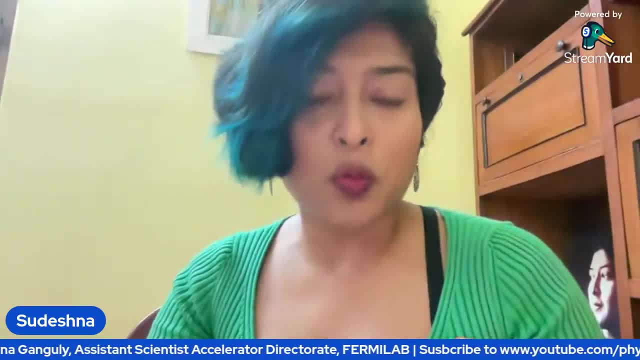 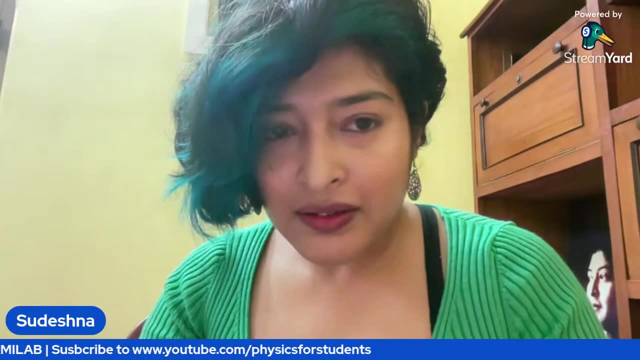 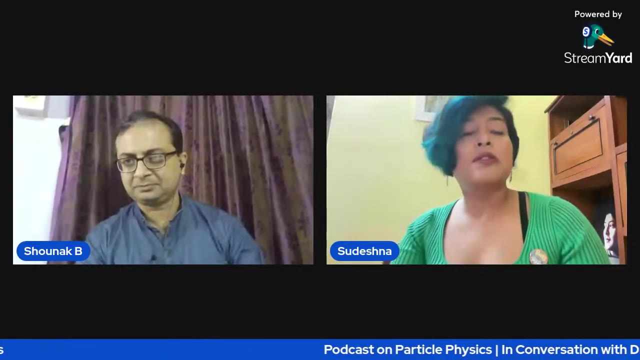 the liftoffs are charged particles and and so so what was the question? why? why do they come in pair? uh, just a second, i will just uh, yeah, yeah, i think that. what does it mean? yeah, so so by coming in pair means, so, suppose, electrons, so it's negatively charged fundamental. 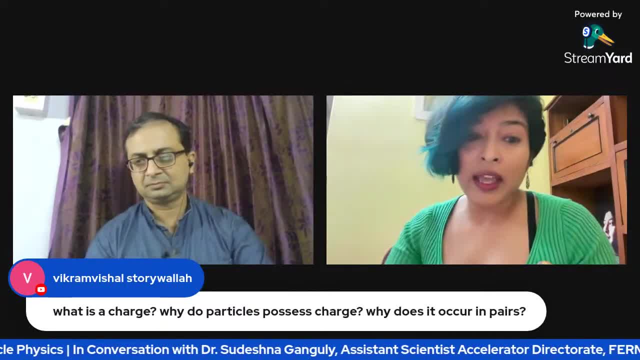 particle, right, so so it has an anti-particle and again, that's all covered by a standard model. so that's the fundamental blocks, that's how they are already created. so that's the fundamental. that's the fundamental blocks, that's how they're already created. so that's the fundamental one. yeah, i'm thinking. you know, you saw a couple of examples where you primarily have an anti particle right and it also has a bunch of electrons, and so you have a one like a and then you can you have something called a work of six, five, six plus, and then you have a product like a particle. it's a. 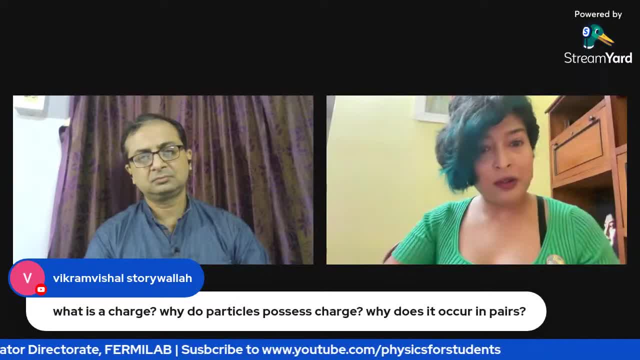 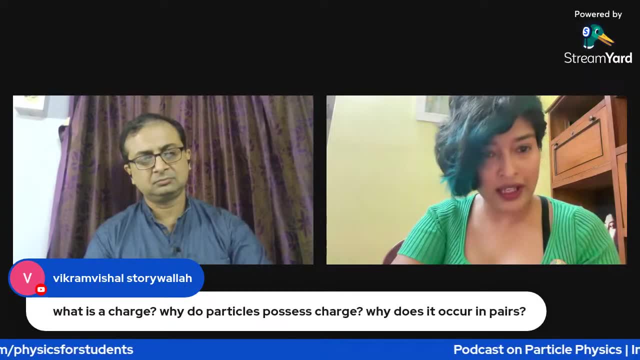 very basic type of a plant and it has a function corresponding to what that thing is, but it's a fundamental, so that's the lowest we can go down. so so all the particles, they have an antiparticle, so so the antiparticle would have a positive charge if the particle has a negative charge and the antiparticle 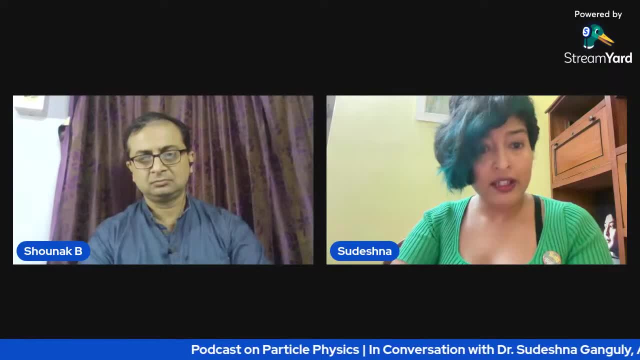 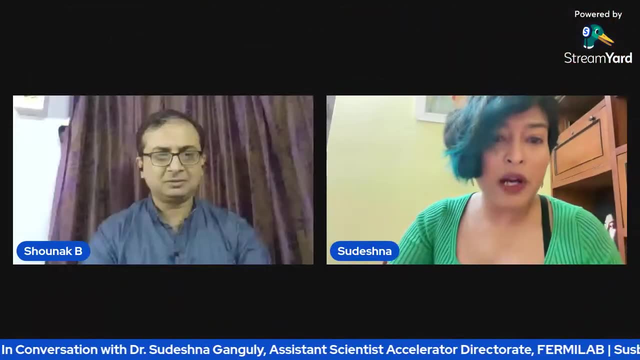 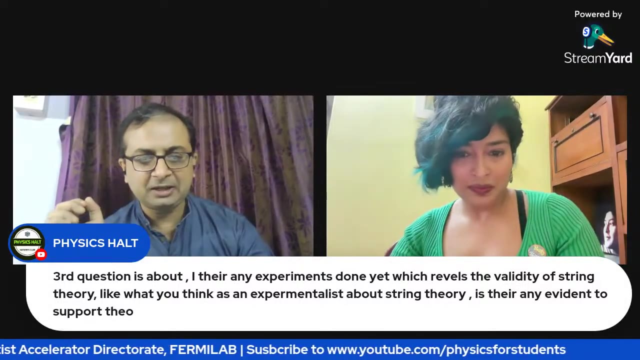 would have positive charge and because of the electromagnetic forces they are there to govern them, they would interact with each other. so that's that's part of part of the. so again, that's part of the standard model. yeah, absolutely got a question that any experiments done yet which reveals the 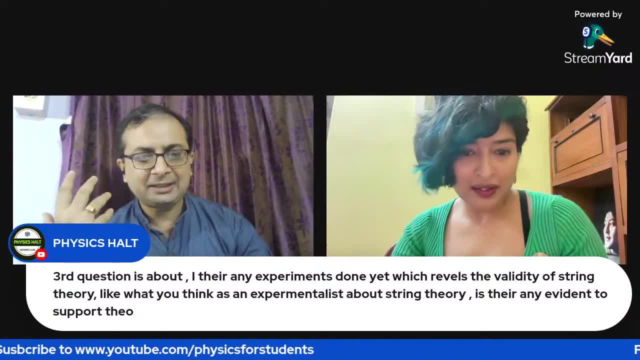 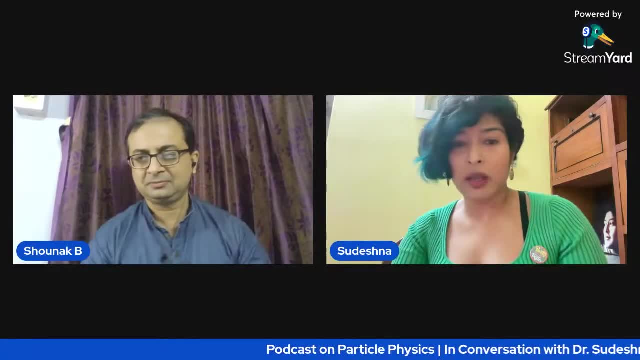 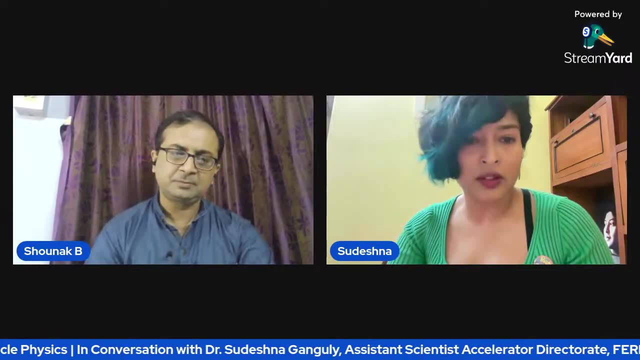 validity of string theory. like what you think as an experimental list about string theory. is there any evidence to support the theory? i i cannot comment on string theory because my work does not relate to that. what i can say, there is still no like a conclusive uh result. uh saying that okay. 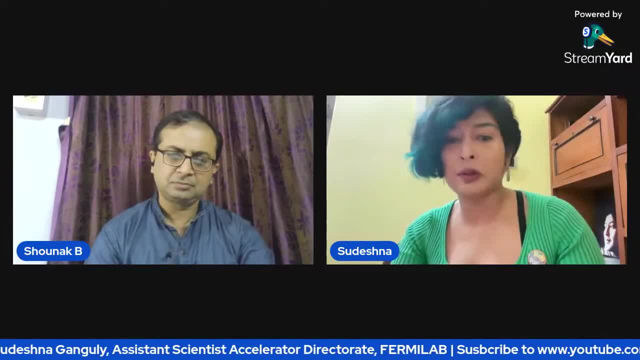 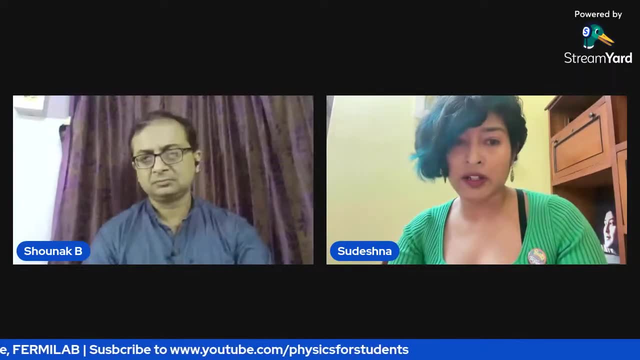 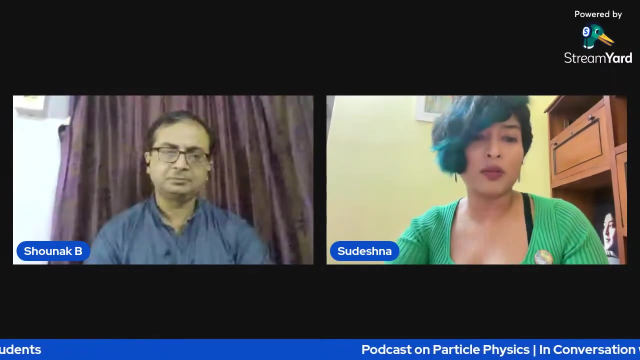 we have validated. there are still searches going on, but i'm not part of the, so so if somebody is interested, i can hook someone up to someone who is working on that. but what i know that, as far as i know, there is no like uh evidence, uh evidence as of now, uh to to confirm that? yeah, so it is exactly how it. 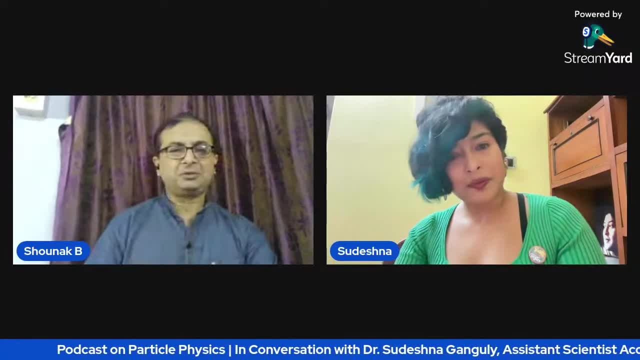 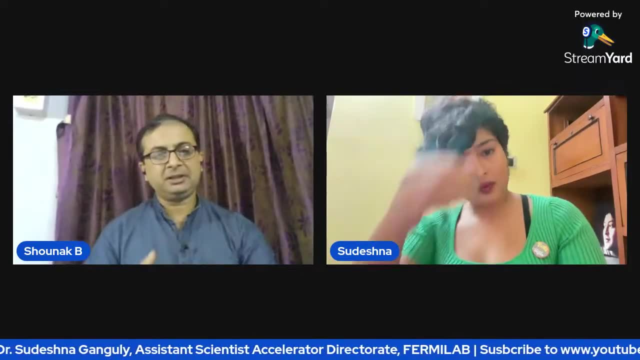 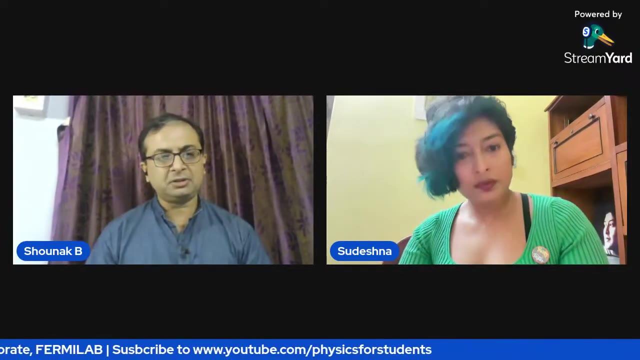 hypothesized, right? uh, before i go to the next question, dr ganguly, i have a question to you. is that, whatever this experiments that you are performing in lhc or in fermilab, etc. uh, starting even from the electrons and protons, these are i mean. just my question is that: are they all? 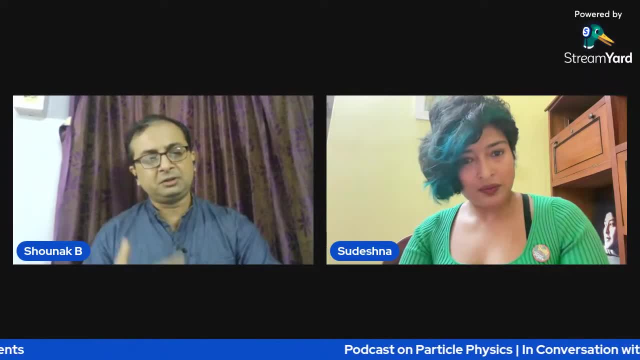 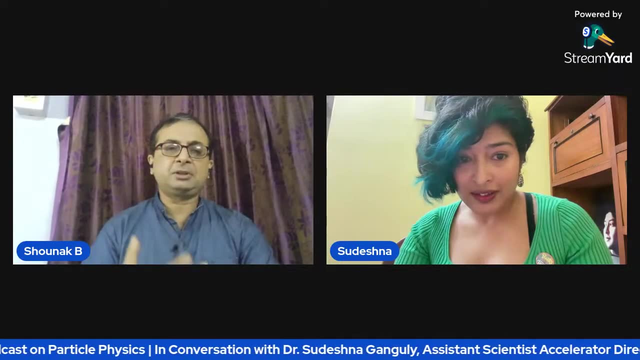 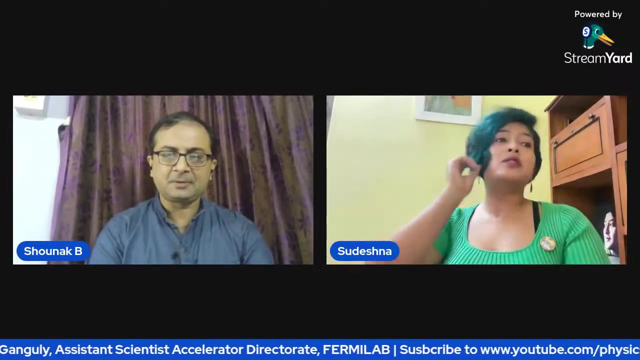 grammatical in nature, or some of them are observable through our eyes. you mean, uh, what we measure? so, for example, the quarks, the anti-quarks, the gluons or whatever that we try to? yeah, yeah, yeah, so, so, so it's not like. so, so for me and you managed to exam experiment. 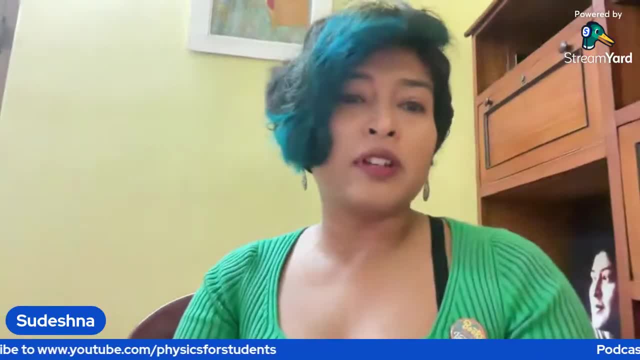 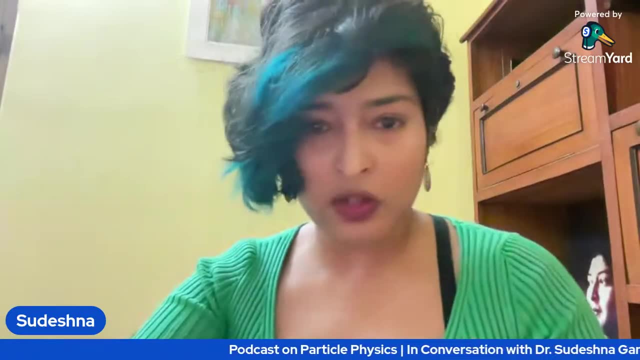 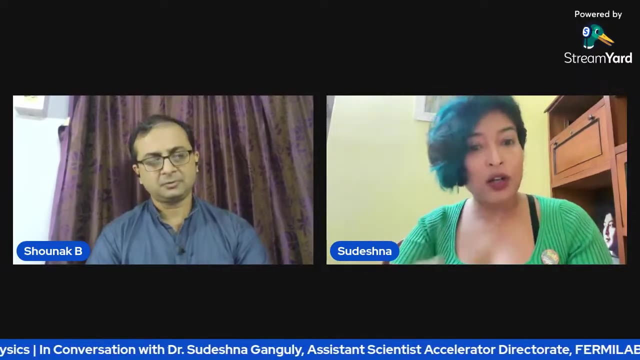 is a very good example of, uh, what you were asking. so in that in that experiment what we try to measure is property of a muon. right, muon is a fundamental particle. we want to measure a property of this particular particle, muon, but we don't really see it. we don't really see the particle itself. we see. 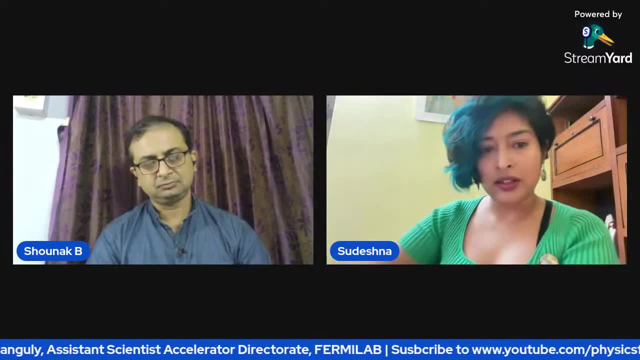 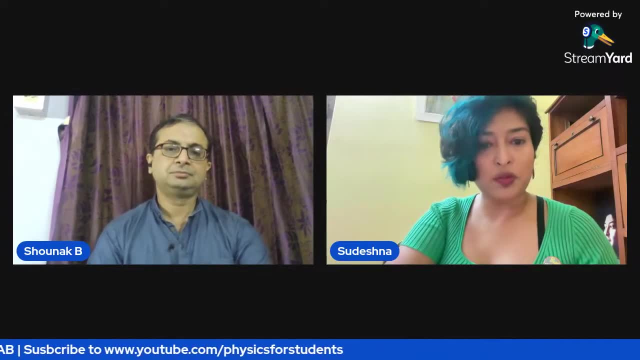 its end product, and even not that whatever energy, and it's depositing in a detector. so we are getting this end product and then mathematically reconstructing back to what we actually want to measure. so we are getting something out of an end product but we have the, the mathematics to correlate. 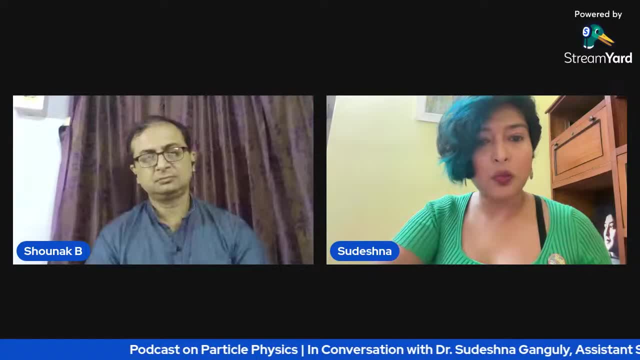 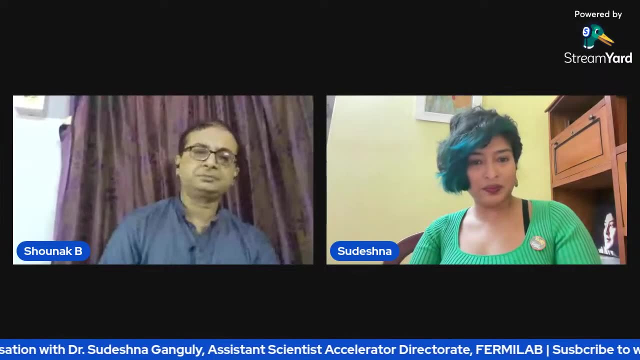 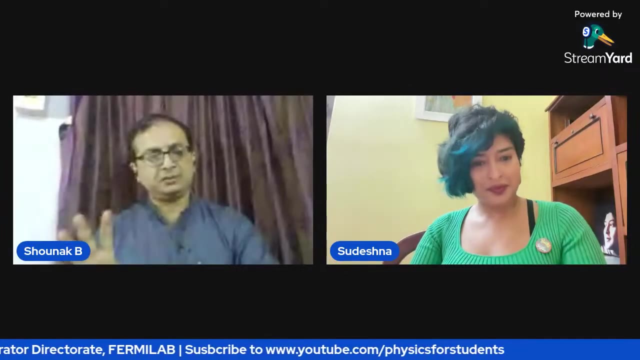 back to where it originated, so we will be able to gather whatever information we want out of that. so I guess it's both like what you were saying. it's a combination of both. that means the textbooks or whatever the blogs, articles that we read regarding, say, for example, 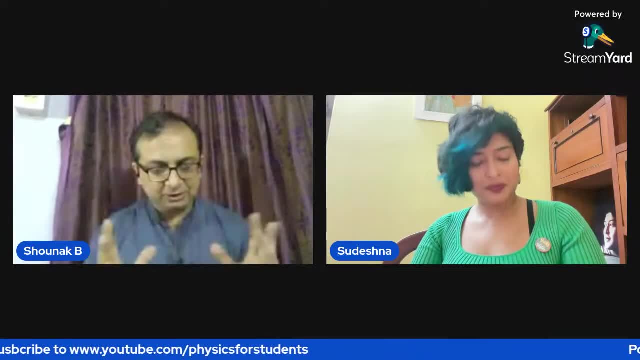 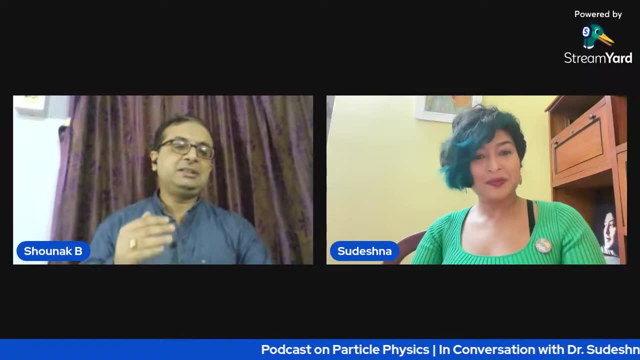 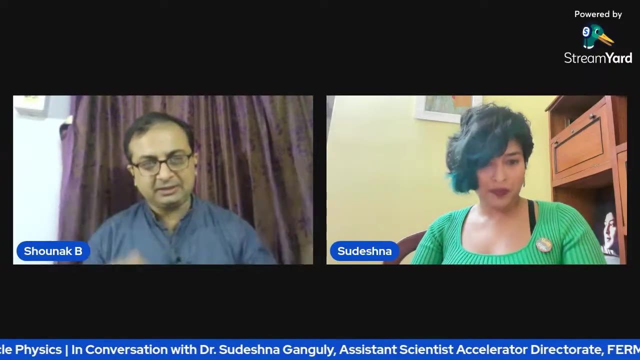 particle physics when we say quarks and automatic imagination of figures come into these things. when we stay of strong force, weak pros, decay of alpha beta particles. that means these are a kind of a I the the painters, or see they have actually created okay. okay, you have a detector, yeah. 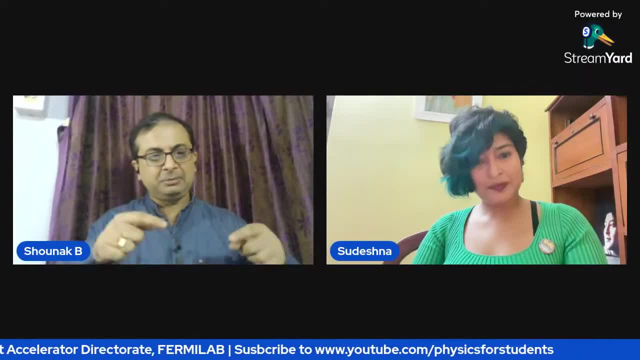 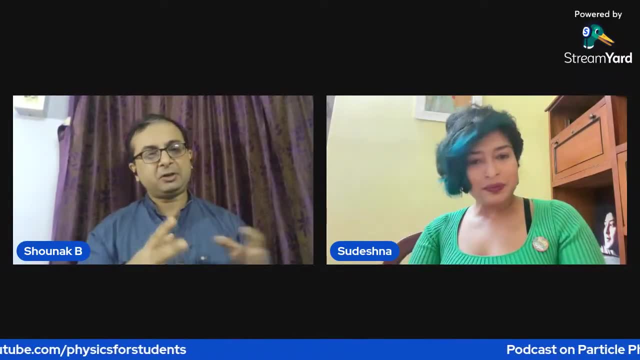 okay. so through the eyes, if I go to the detector, I won't be able to see a quark like up and down physically, something like that. yeah, okay, okay. and my another question to you would be because particle physics is something which is dealing on a fundamental level. 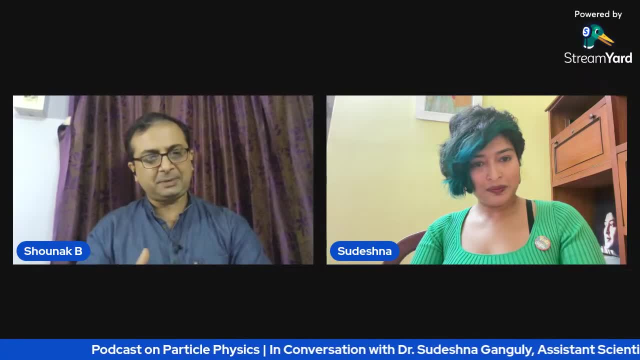 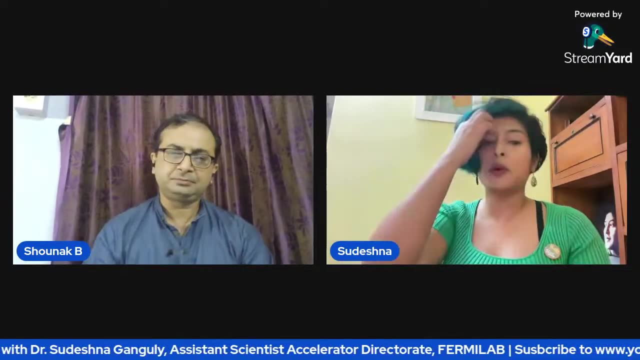 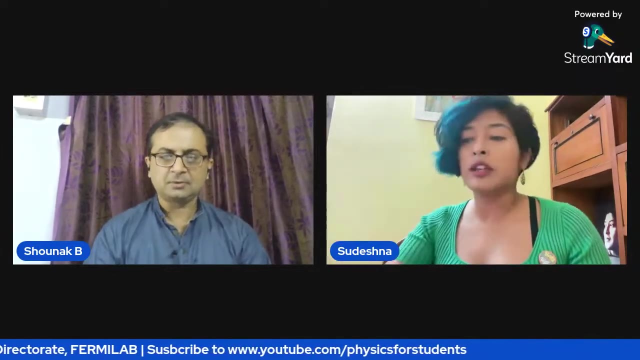 the very up upcoming Quantum field theory, the mathematics, et cetera. does it work with particle? it's a totally separate yeah, yeah, no. particle physics, yeah, the theory part is all is dominated by quantum field theory. quantum thermodynamics is delving in the quantum world, like where, like. 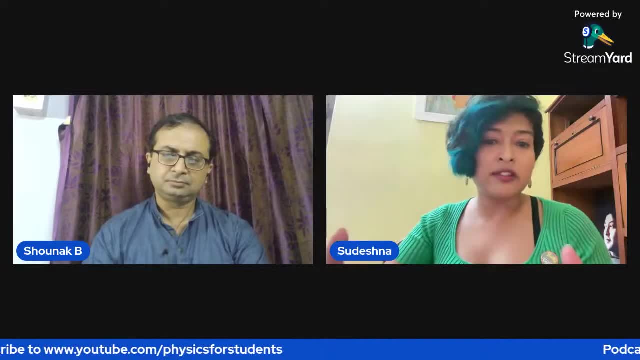 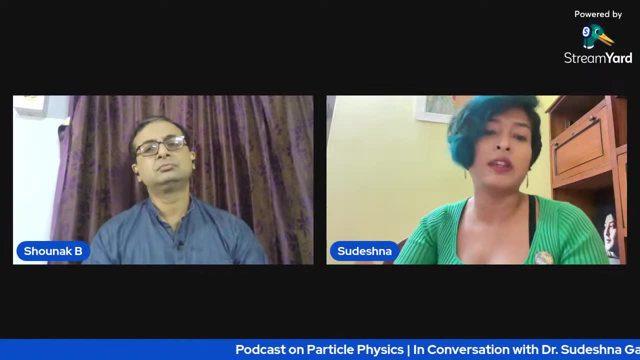 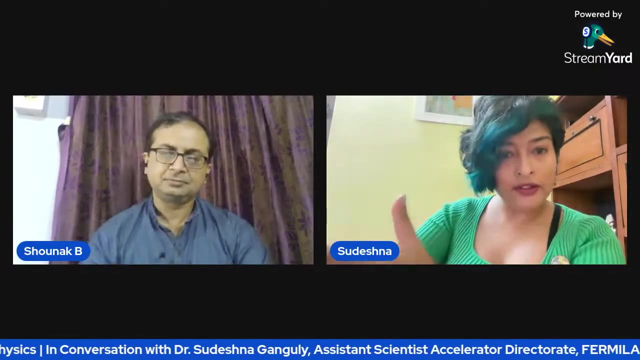 the basic say dynamics, that's completely newtonian, classical. but particle physics is um delving in the realm of new, uh, quantum physics, quantum field theory, quantum chromodynamics, that's the theory, basically. so we, experimentally, we show, we show. okay, here is the proof, we, we have proved something. 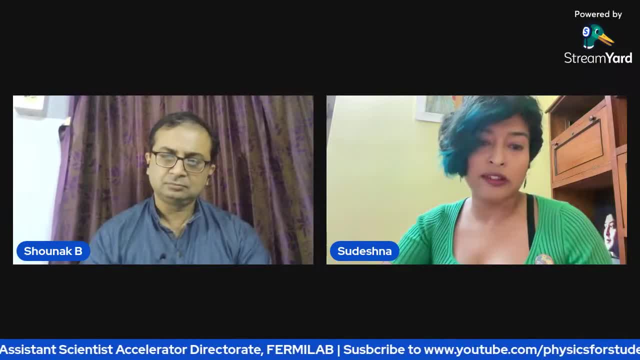 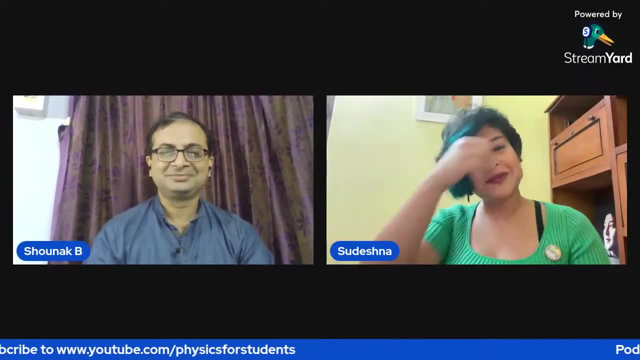 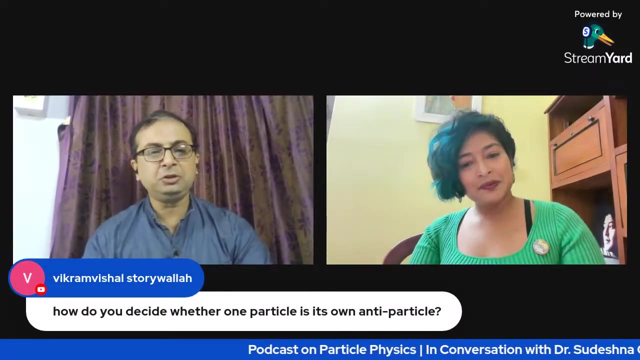 and then we talk to our theory colleagues and they come up with hypotheses and they say: okay, so this is the particle or this is the force which is causing this difference. simplistically, that's how it works. so we collaborate today, right? uh, this is another question coming up from vikram vishal: how do you decide whether one particle is its own anti-particle? 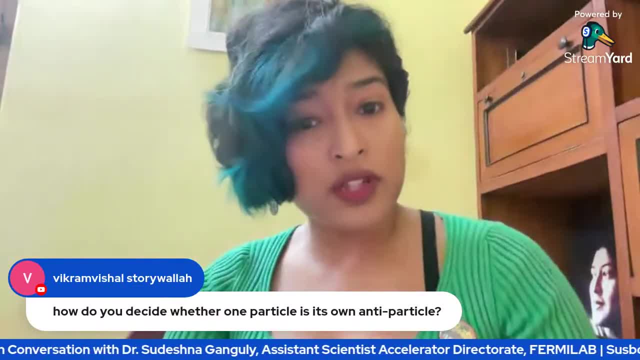 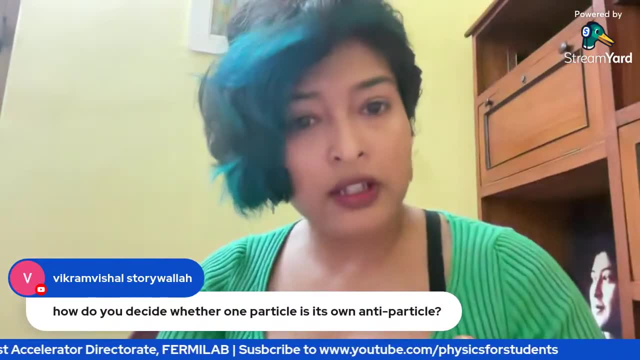 so so it. that has not been completely proved yet. so there is this hypothesis, this miorana hypothesis, and which, which says that if neutrinos are their own, entire neutrinos and many of the phenomenons could be easily explained. that's one hypothesis, that's still at the hypothesis level. 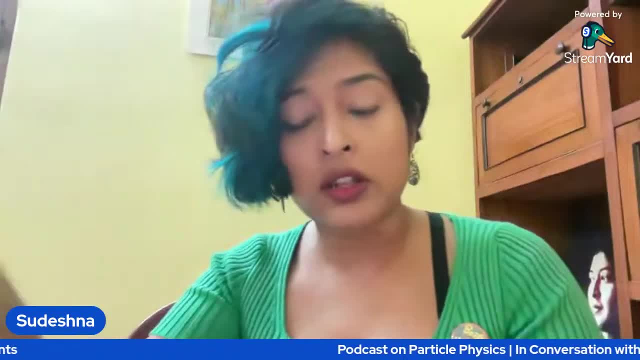 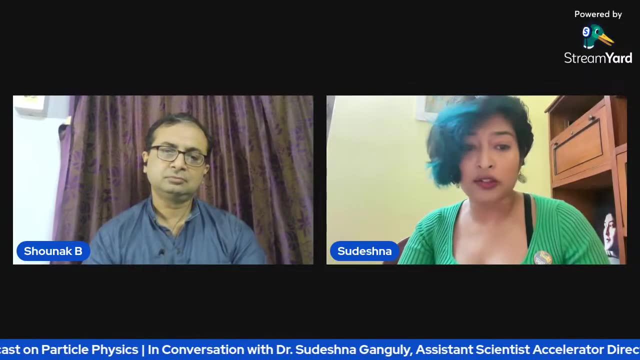 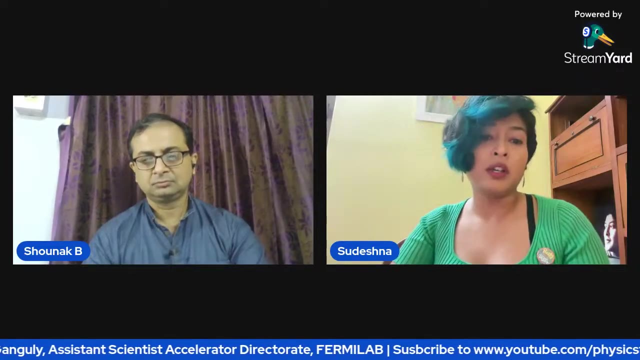 so you haven't got experimental proofs yet. so for that we would need future neutron experiments. the difficulty with this is neutrinos are so elusive they do not interact much right, so we have to pretty use very high intense beams so that we have many more neutrinos at a given amount of time. 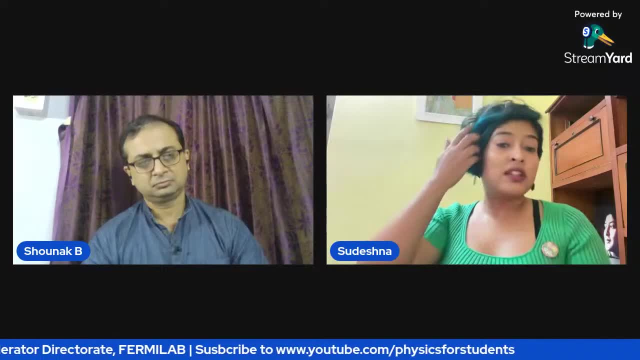 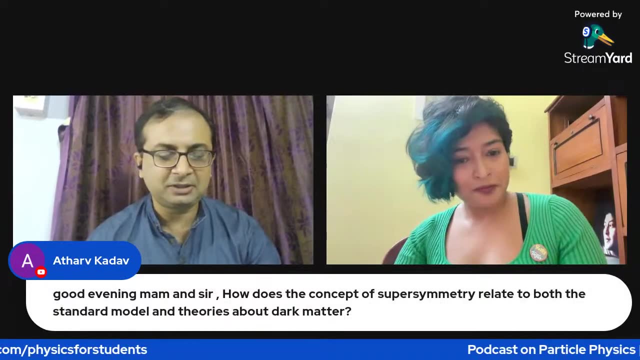 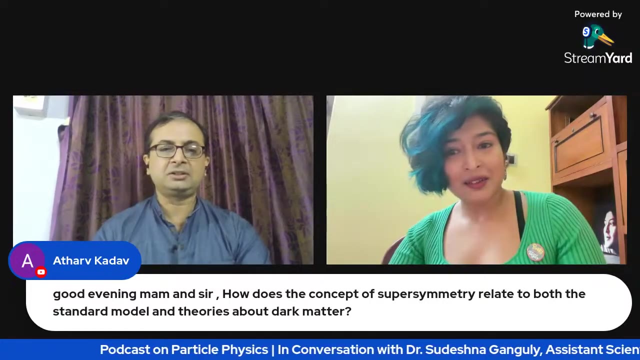 so that's why we need future neutron experiments like june. this is a hypothesis still, so we do not have experimental proof. okay, thank you. athar kadav has got a question. good evening, ma'am and sir. how does the concept of supersymmetry treats to both the standard model and theories about the 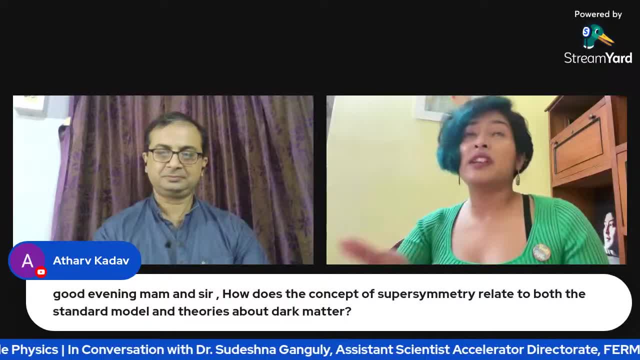 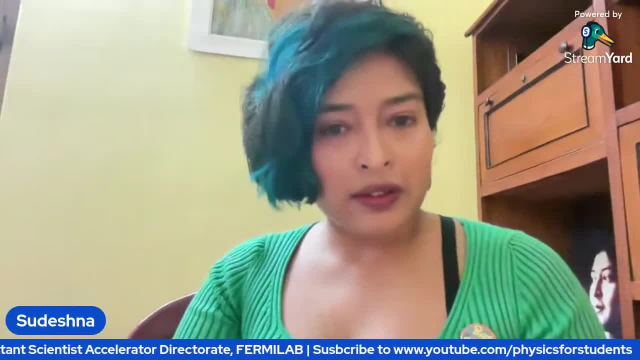 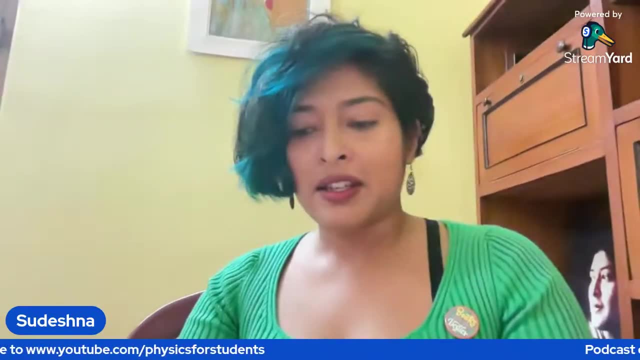 dark matter. well, yeah, so, um, supersymmetry: again, there was no proof of the supersymmetry, but it it is like. again, an analogy is: um what the theorists think that imagine a gem and different facets of the gem. so the theorists think that all these three forces that i talked about in standard 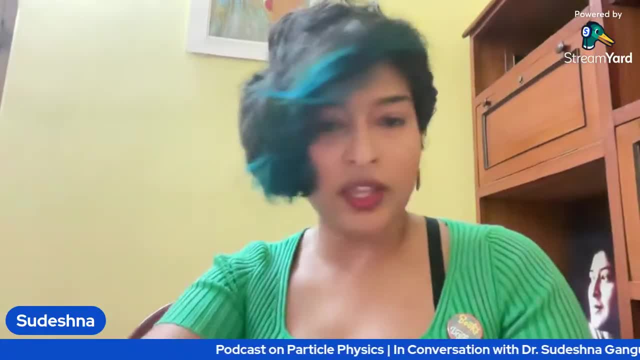 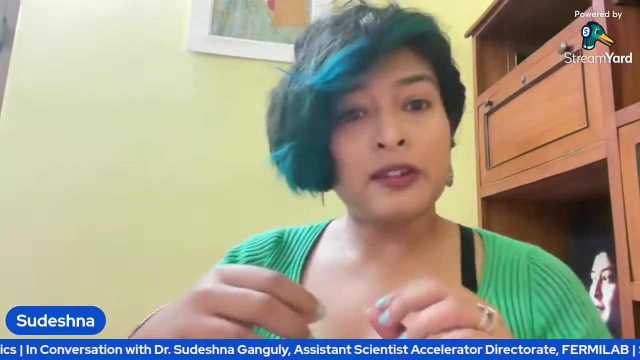 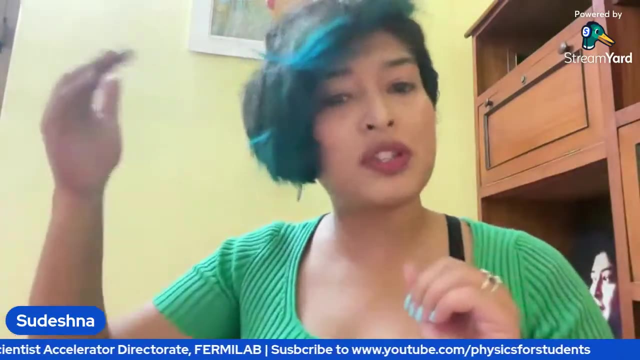 model, the electromagnetic um- weak and strong. so these are different facets of the same force, underlying force, right? so maybe at the energy level we are used to we see them as different forces. but if we can go to a much, much higher energy level, maybe they would appear as the same force. 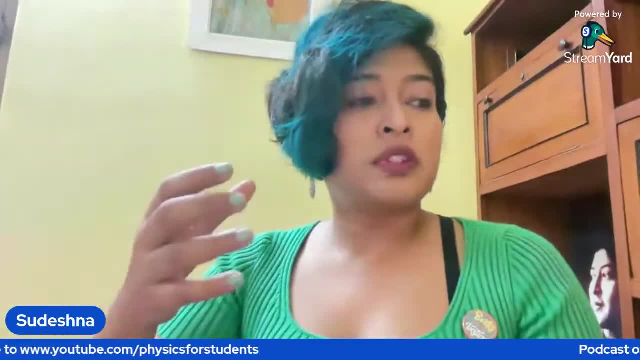 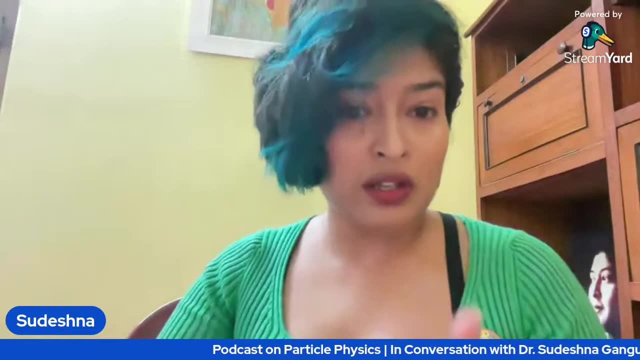 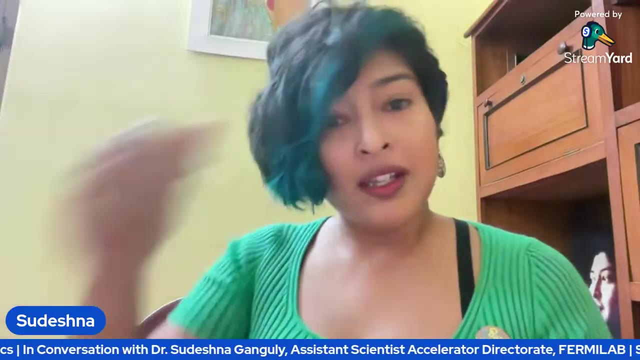 so that's the grand unification theory, right? so so the hypothesis right now is that standard model is only an approximation of a deeper underlying fundamental theory. but again, so so that's that's the question, then: how can we see it or how can we improve it? so so then the question is: are we? 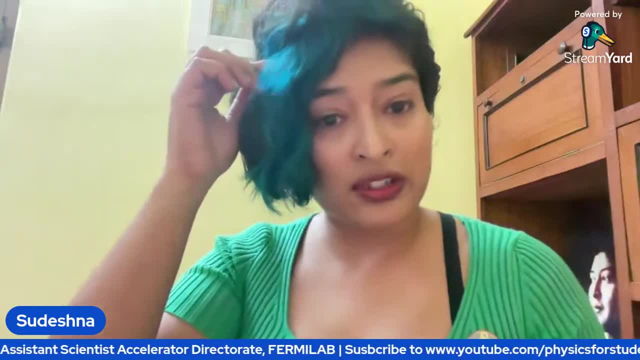 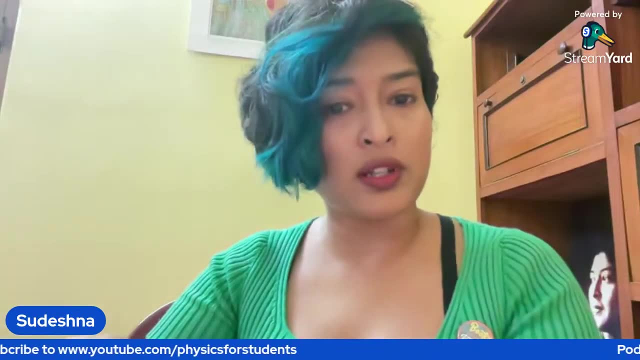 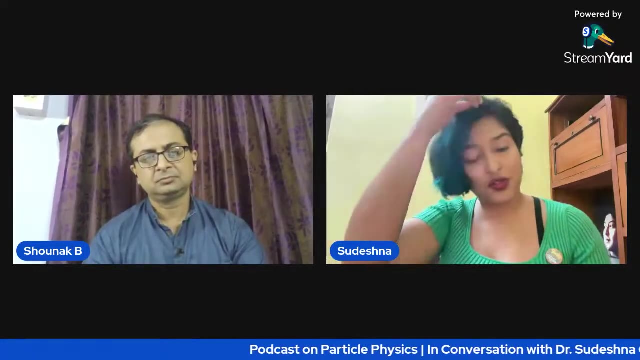 creating enough energy? are we creating enough high energy in cern? what if it's beyond what cern is creating? and that's when those indirect ways become important to find these answers. if we cannot go up in energy, it's super costly. it's not simple to just go up and up in energy. it's massive. 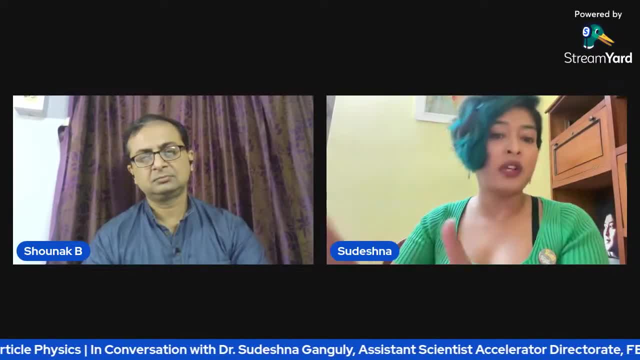 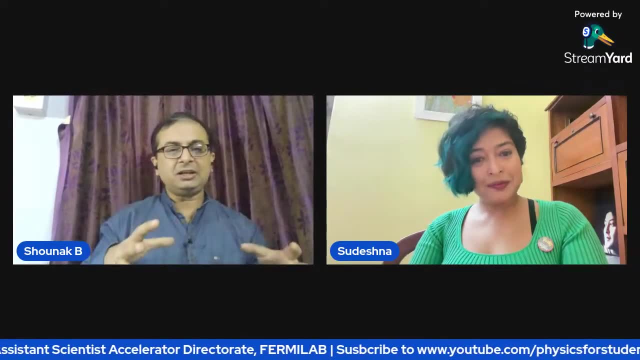 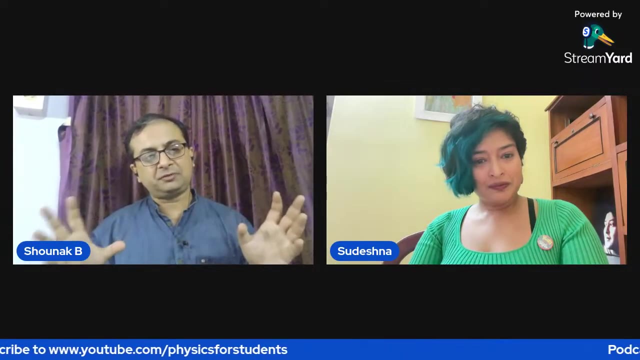 so then the other, other method, other avenue becomes important to find these answers right. thank you, doctor, for answering all this question now. cern and fermilab: i mean this might be a very idiotic question to you, but i think it's a very interesting question because these are two. i mean to say they are 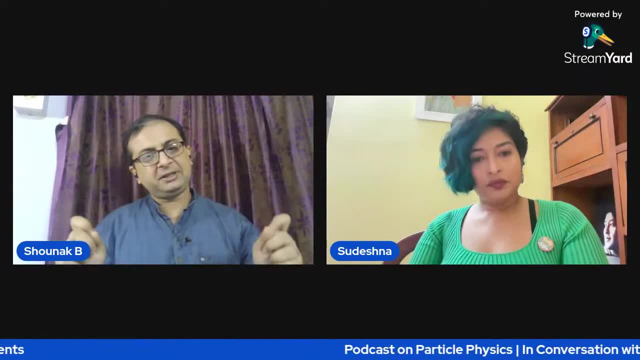 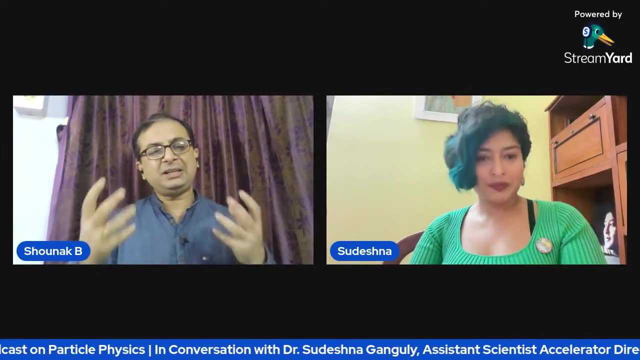 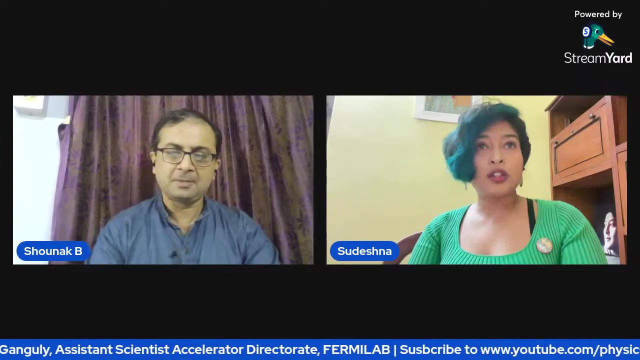 both from the government, one from us, one from geneva, switzerland. so the basic objective is the same: doing research in particle physics and look for new physics, look for new physics. so what is the difference? i mean to say what fermilab does and cern. i mean to say what are the areas fermilab. 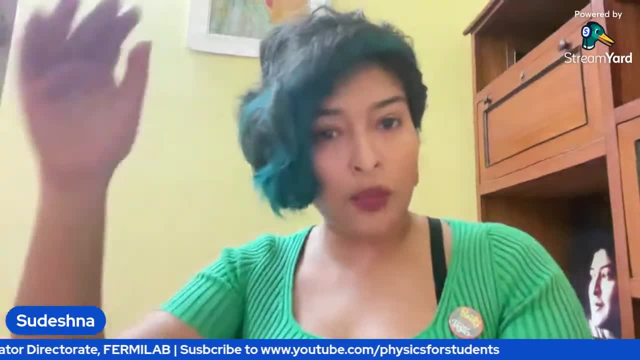 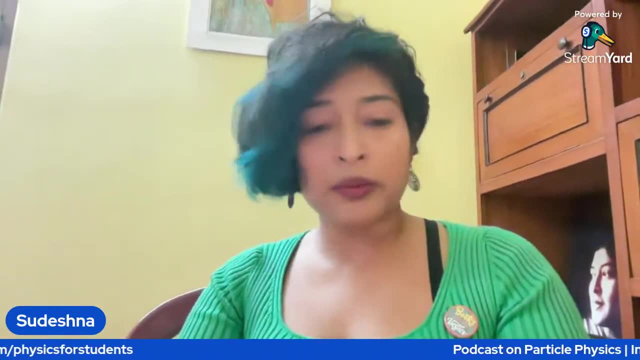 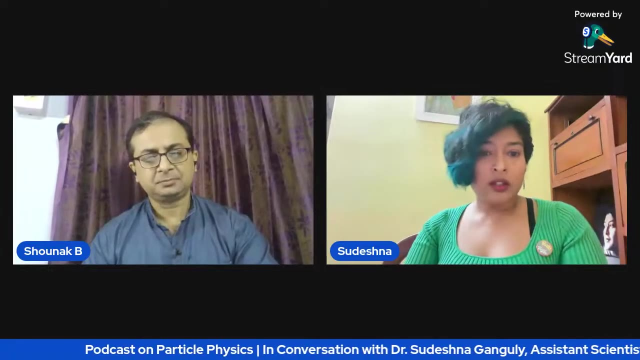 so cern does in, cern does energy frontier. so they are trying to go up and up in energy. so that was my analogy, uh, that they they saw his and if something new exists within the energy they're they're able to create, then it will just go bump in their data, they will see a peak and it will target new, new physics. 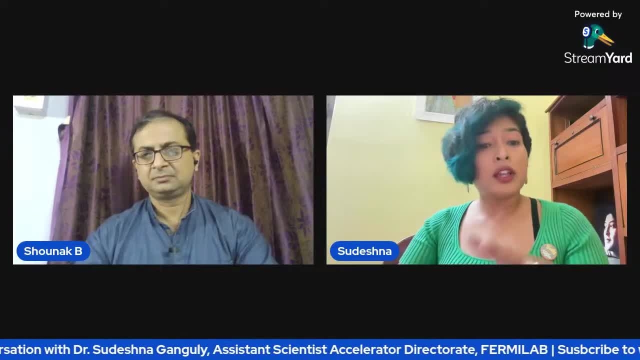 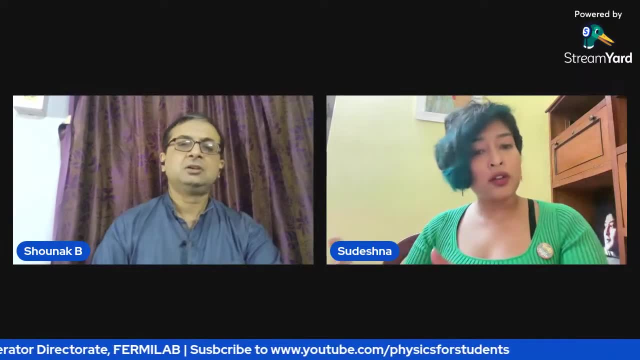 that's, that's their way: like colliding particles and creating, like trying to mimic big bang, like situation and creating massive energy. so that's their and and we are not trying to do that here in formula. we're not trying to go up in energy. instead, we are trying to create intense beam and 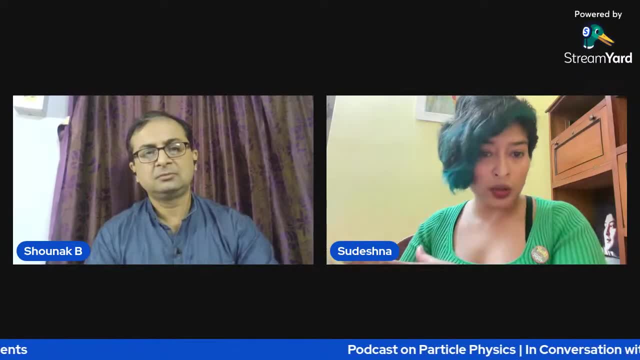 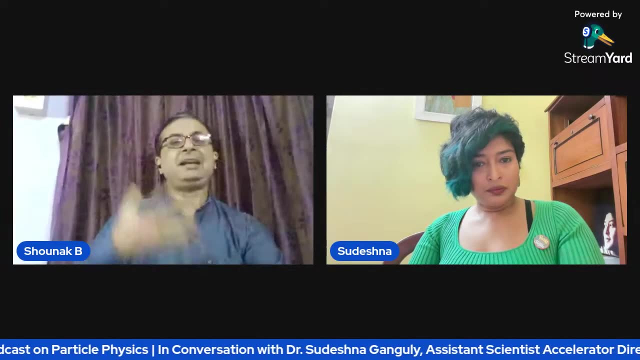 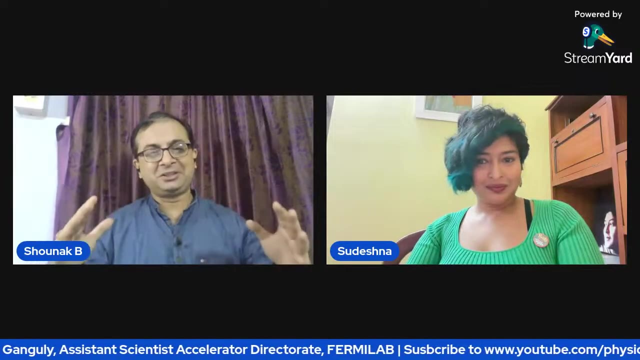 doing high precision measurement. so so we, we are doing intensity frontier or precision frontier. so when we come to producing very high energy, i mean to say, as you rightly told, i remember the book of money telling that- as you rightly told, that once everything merges at the same. 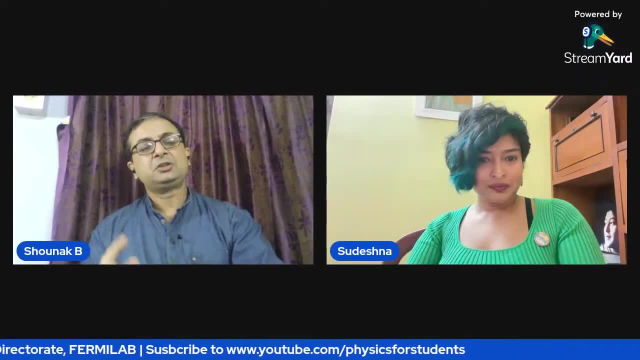 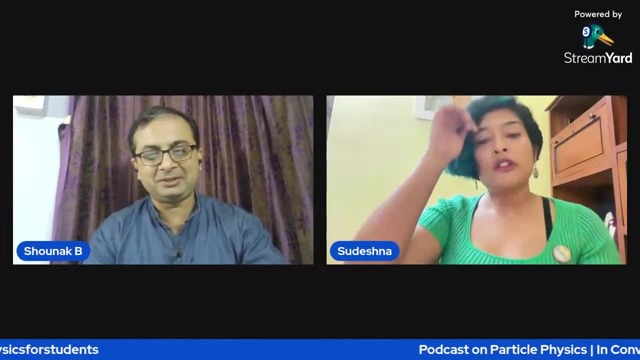 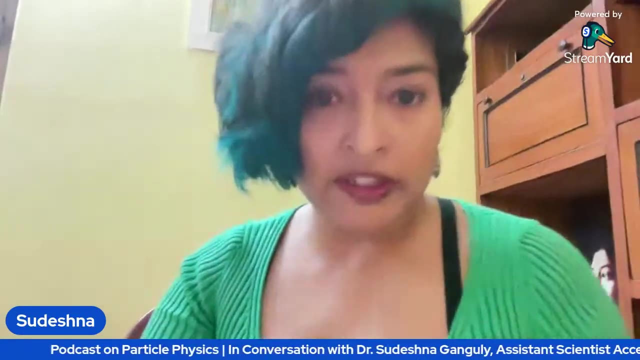 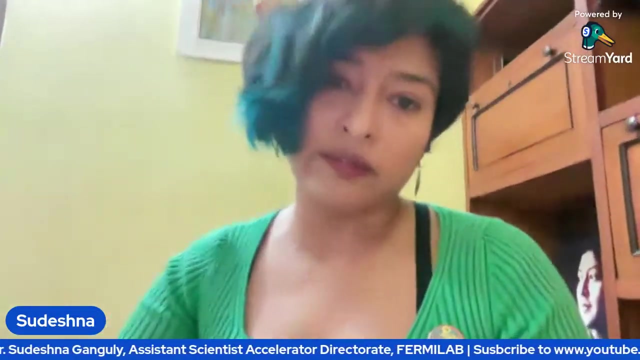 maybe this cosmic level, so we would be able to understand. so this production of high energy, how does it happen? i mean to say, what is the if you just tell us in few lines: yeah, so well. i mean, in particular, you know, like in future we're gonna try to think about how to train our 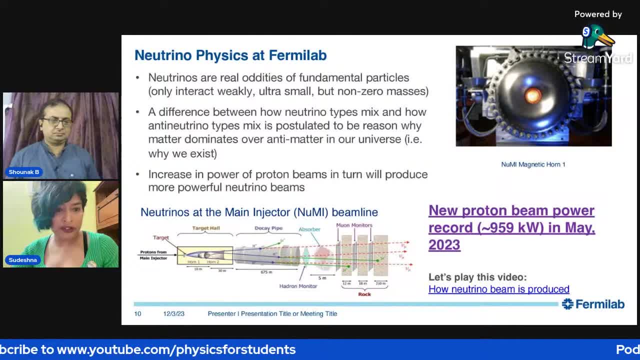 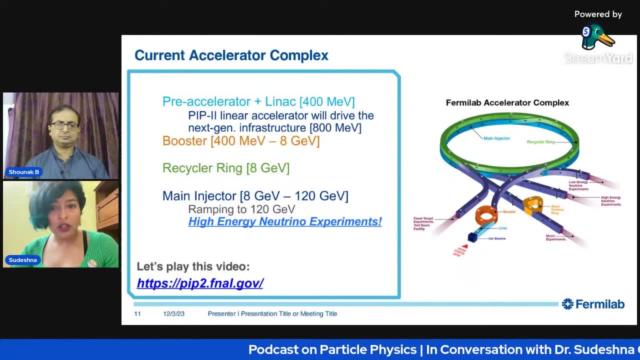 Grandma know how to vehically create the energy from the world. so we're going to see if, like if you could see where you could normally go right now, where you could do what you do at your own place, where you could see if we could create energy. if we create energy or just you know a country or 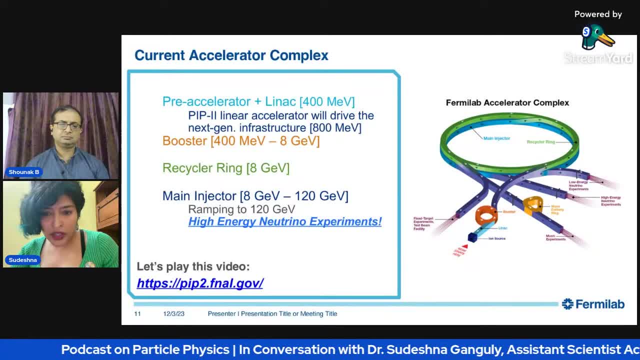 a country, you could create energy. so we're going to try to train our Grandma and do that. so, um, am i showing the right slide? yeah, so so you can see, um, we start with the source, a proton source, and then this is a linear accelerator. this is the linear part where we are just so, from here, 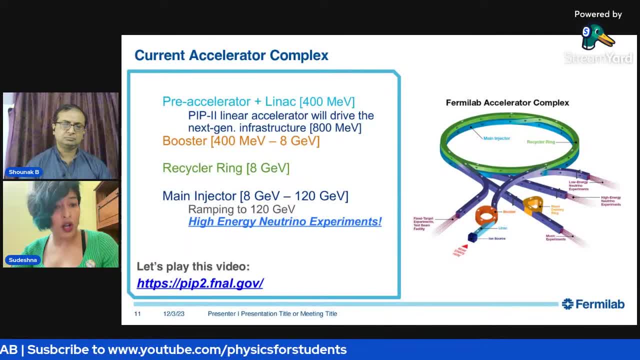 from the beginning. we increase the energy of the particle to 400 mav. then we send it to this ring. this is called the booster ring. so in this booster ring then the energy is ramped up to 8 gv. so now what comes out of this is 8 gv. then we send this 8 gv beam to this ring called recycler the green. 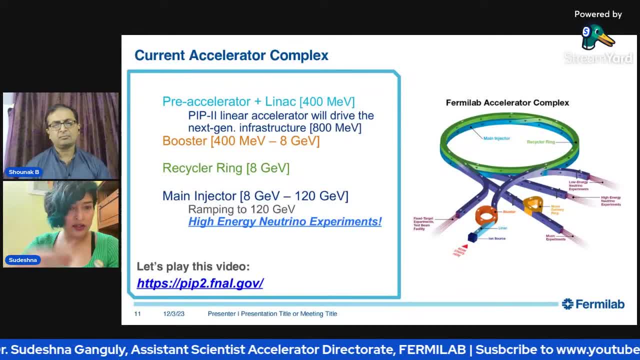 one on top and recycler is like a storage it's. it's collecting the the beam in bunches and creating batches, and then it sends the beam to the down ring, which is the main injector, and main injector then takes this 8 gv and then increases it to 120 gv. so what comes out of this? 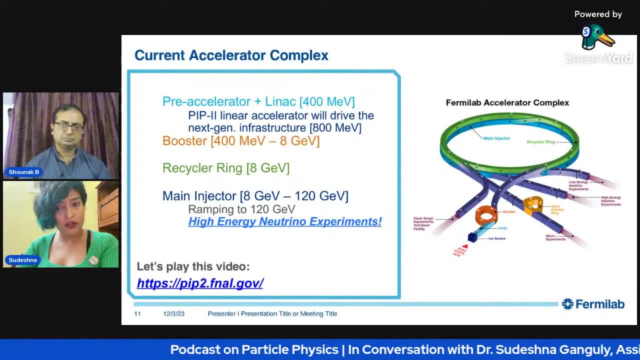 is 120 gv and we send that to the neutrinos. this goes to the neutrino beam line, right, and what comes out of this green that goes to the me on campus. so so, so that the accelerator complex is, we have the tuning facility so we can either produce 8 gv beam or we can 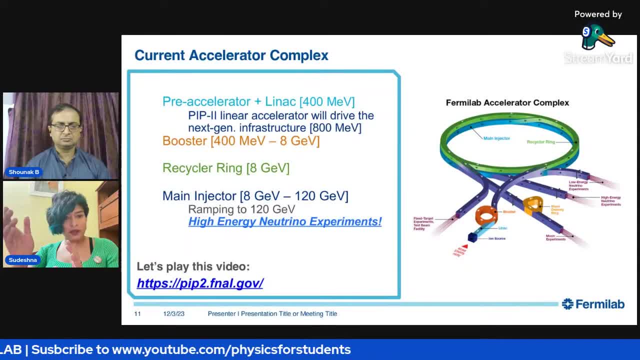 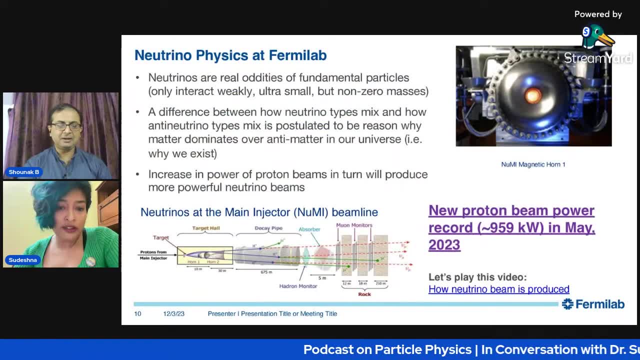 produce 120 gv beam, so cern also probably have like similar tuning. i don't have their right, so the complex here right, but but once you have the proton, then we have a target. and this is all the neutrino experiments. they follow the same way. you smash the protons onto target. then what comes out outside the interaction, the collision? 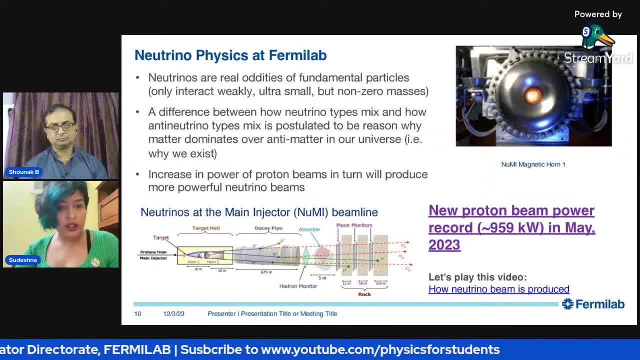 that those are pines, the secondary, these are pines made of quarks. so then we have huge magnetic focusing horns. they're shaped like horns, we call them horns. so they will select the positive pines and then they will send them down this decay pipe where the secondary pines are decaying to muons. 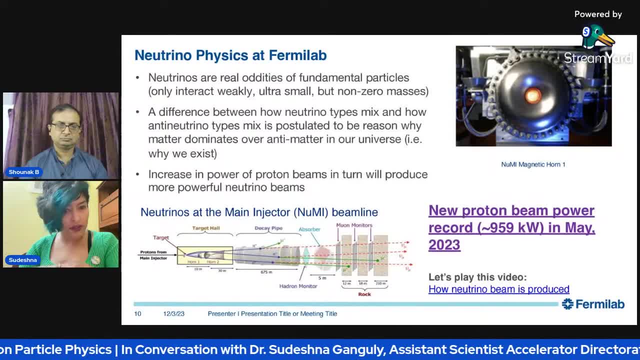 and neutrinos. so then we collect everything- these are the filters, we filter everything else except- and then we need to send the neutrinos down underground 700 miles to south dakota. and so so this is this is how basically it works, like okay, so the lab, i mean to say this acceleration of 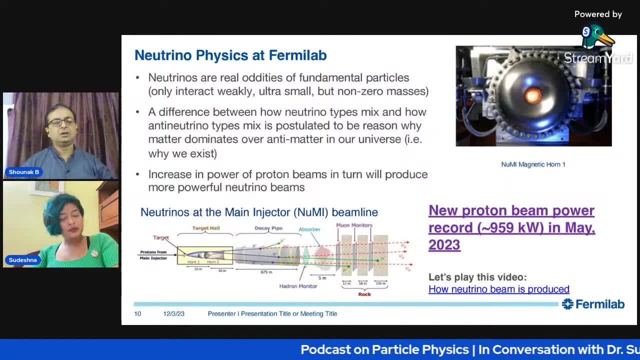 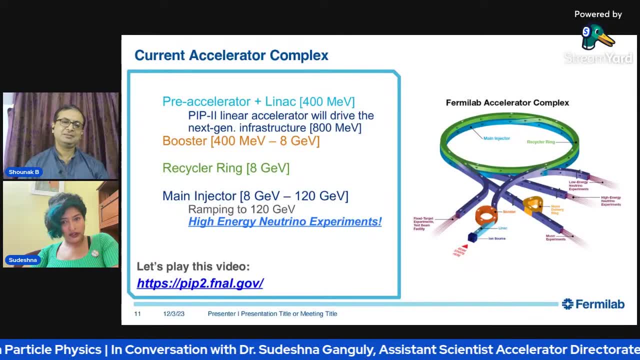 particles happens below the ground. yeah, okay, and how long it will be? this, this is under. this is above ground, but all these are underground. okay, this is in formula, campus. so if you are above on the plane or you're looking at your uber app, you will see this ring clearly on the map. 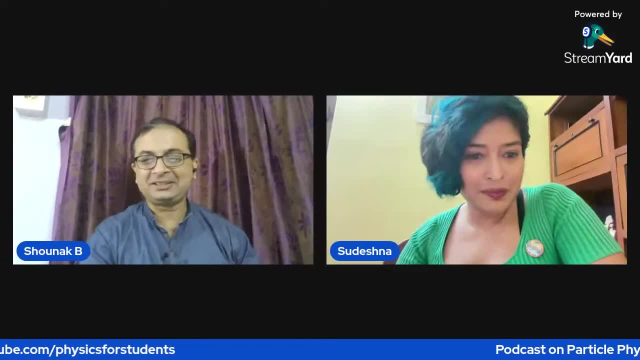 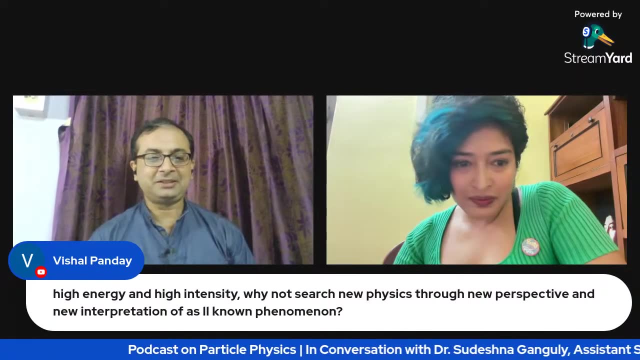 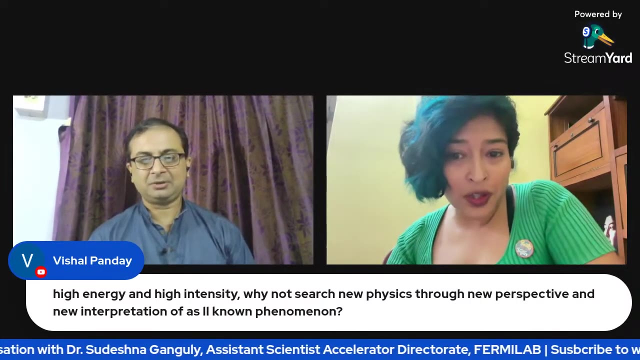 that's wonderful. that's wonderful. okay, i will take a few questions. uh, doctor, first, is that high energy and high intensity? why not search new physics through new perspectives and new interpretation as known phenomena, two known phenomena, okay, so so what are? so then my question is: what is this new perspective and new interpretation? yeah, do you mean? 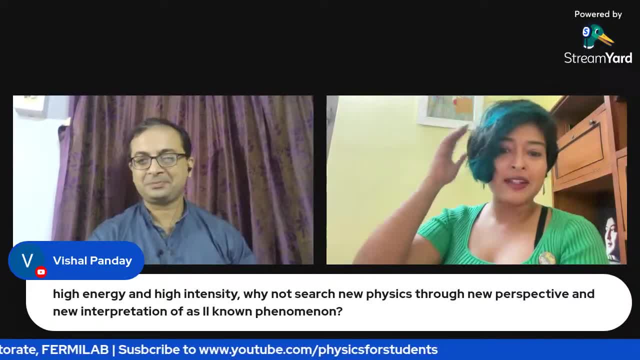 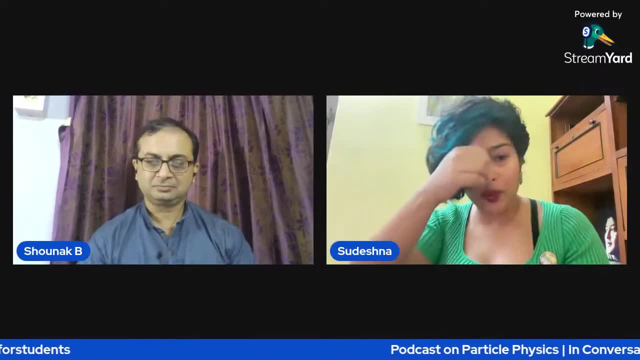 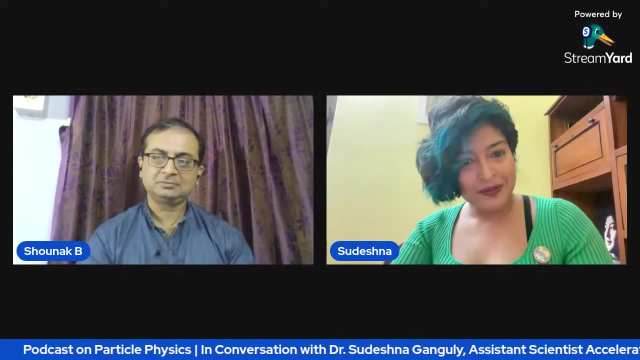 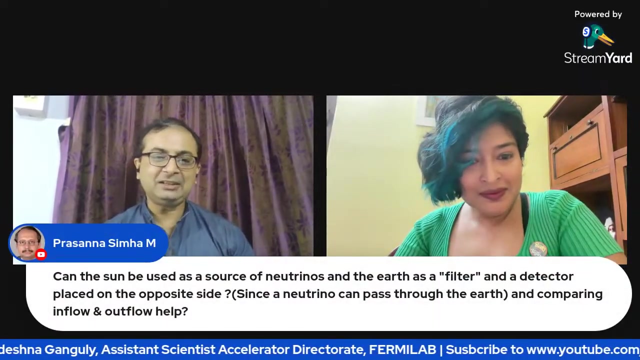 the theories. yeah, experimentalist, we will have to find either we'll have to do it experimentally, like actually palpably, either go high in energy or try to find indirect way what you are suggesting. maybe theorists can use different interpretations and provide us with different hypotheses. right, uh, prasanna sinha m the, our doctor, cardiac surgeon. he has got a question. can the sun be used? 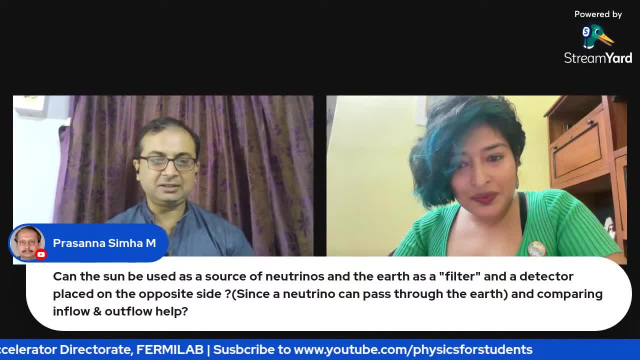 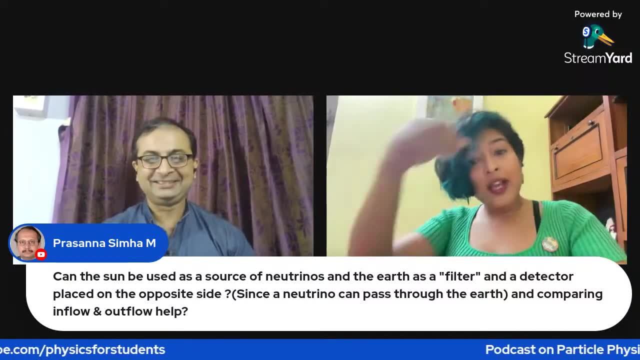 as a source of neutrinos and the earth as a filter and a detector placed on the opposite side, since a neutrino cannot pass through the earth, and comparing inflow and outflow health. so so, yeah, so, so there are atmospheric neutrino signs as well. there are some labs, um, i don't remember. 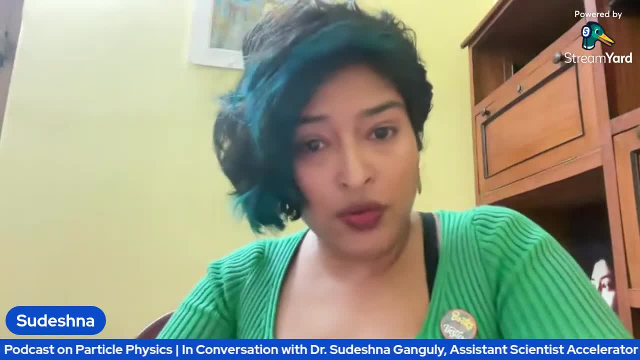 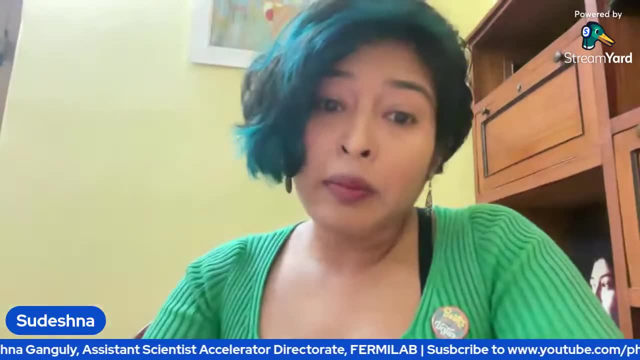 exactly the name. uh, they do study atmospheric neutrino. where we are studying what we're studying is in a, in a controlled manner, we're creating neutrinos, but yeah, but like we, millions of neutrinos are passing through us every second actually, but we don't see them because they don't. 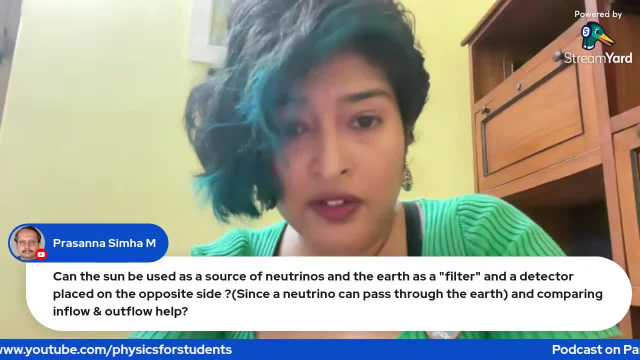 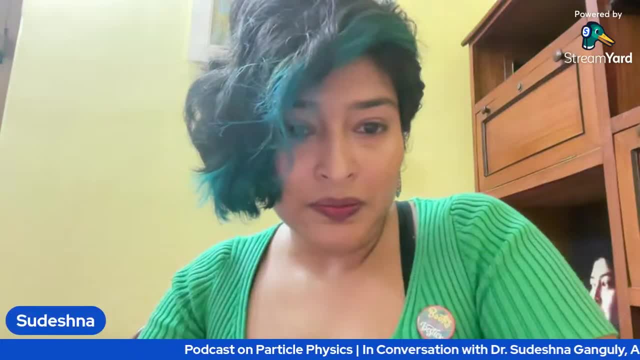 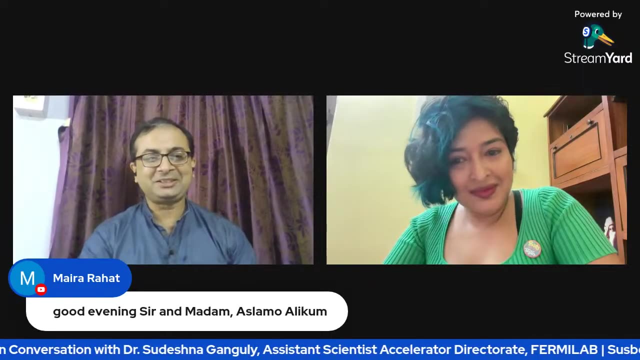 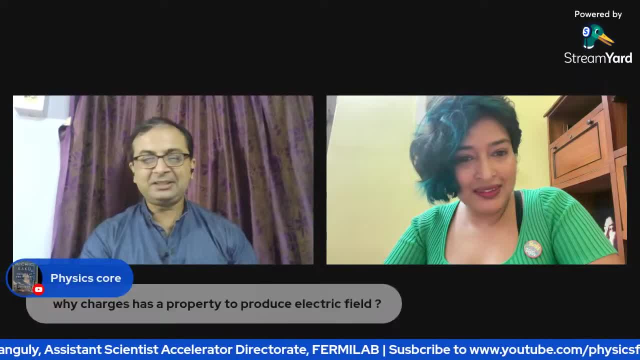 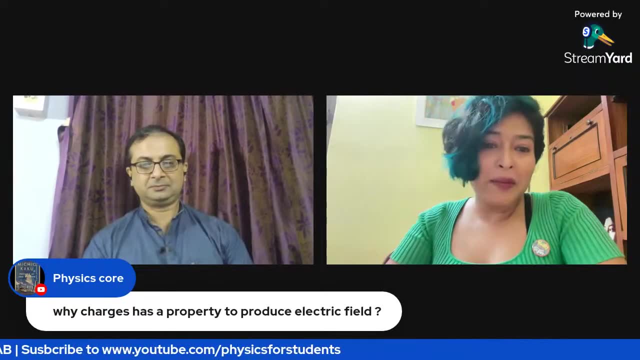 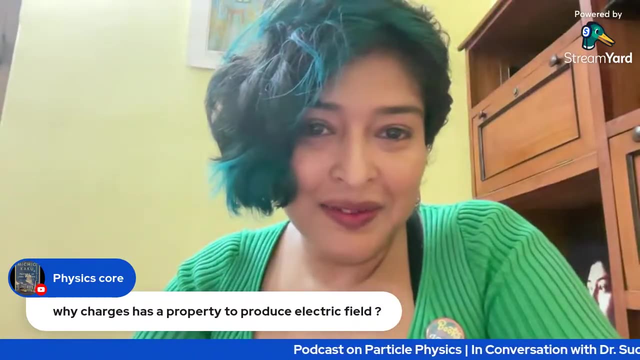 assalamu alaikum, welcome. uh, mahira. uh, physics core have got a question: why charges has property to produce electric field. well, yeah, i mean again, these are fundamental properties. that's how they are built. yeah, i'm, it'll be. really don't have that kind of a why. 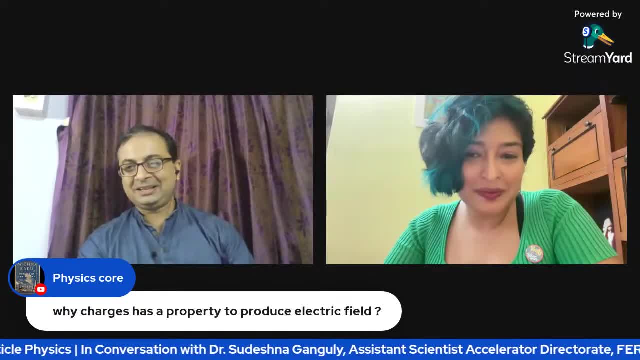 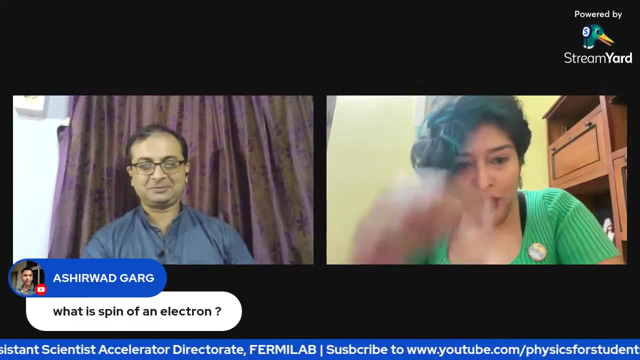 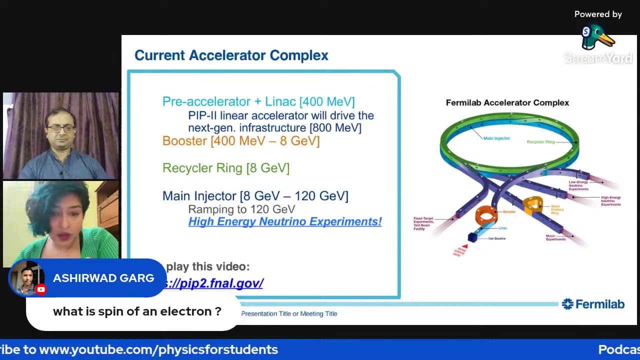 until we dig down further into the details. yeah now, this is from ashir vadgad. i think this is a good question: what is spin of an electron? so for screen? i do actually have some nice um cartoons on my slide, okay, even though it's spin of me once. but it'll answer the same question. 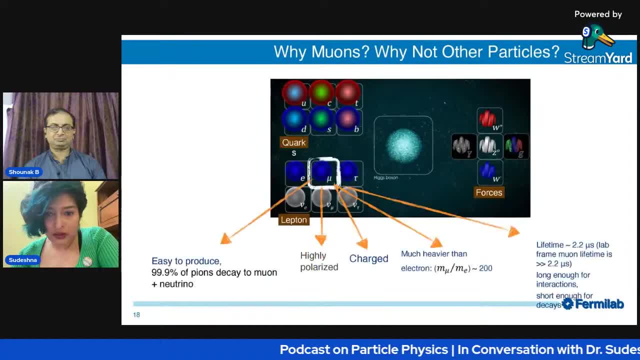 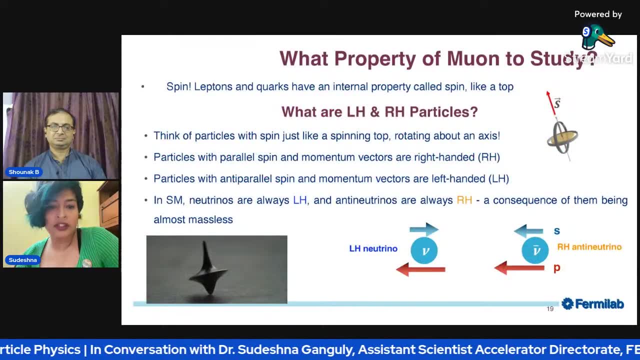 uh, i will skip all those, all those. yeah, so i wanted to talk a little bit about spin anyway, but oh, sorry, this is a pdf so the animations will not work, but that's fine. so so i i mentioned leptons already. leptons and quarks are fundamental uh particles, so they have this fundamental property. like charge. spin is also. 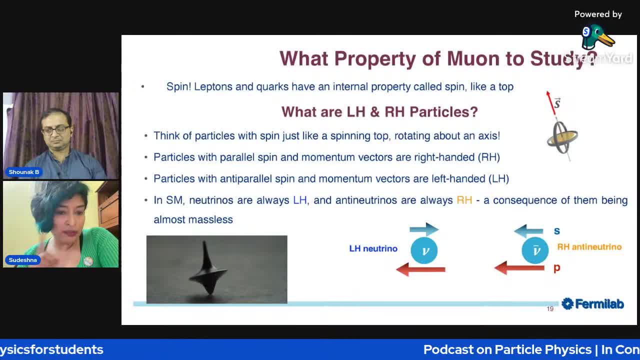 fundamental property of this leptons. so imagine a spinning top. it's, it's pretty much like that. that just a spinning top, like in this picture, right? so? so that's what i wrote here. just think of a particle. as, with spin, an electron is a lepton. so that answers the question. so think of a particle. 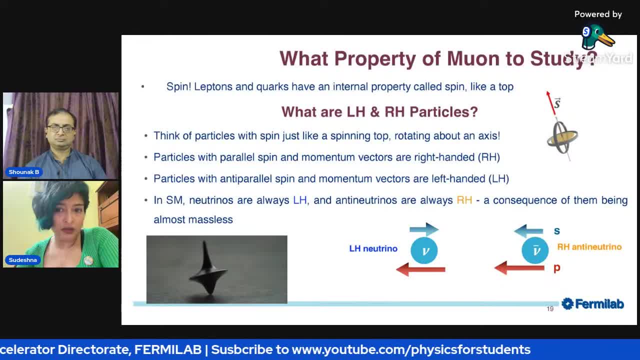 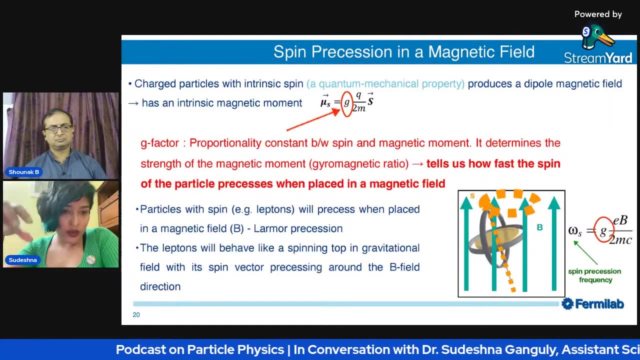 with spin, just like a regular spinning top rotating around an axis, as shown in this picture right. so i don't have to go to all this left-handed, right-handed. so again, this is a basic property and what happens when you place a particle with spin with in an area with external magnetic field. 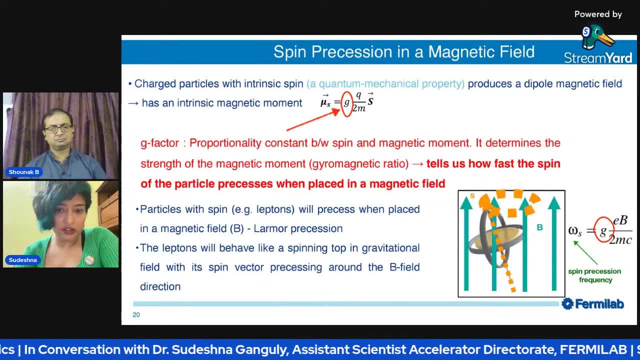 so. so the spin rotates, processes with respect to the external magnetic field and and that gives rise to this magnetic moment, and that's the whole physics of g minus two, basically. so spin is a good segue, because that's what we try to do in g minus two. we measure how. 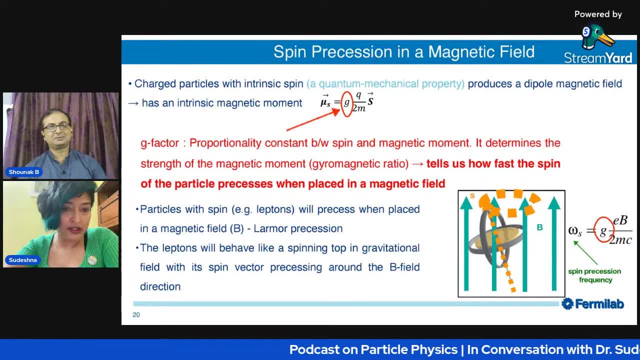 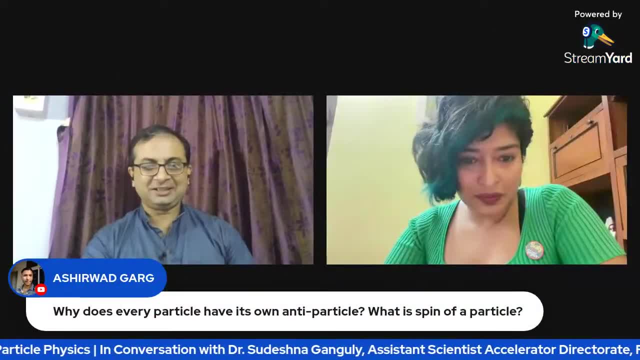 fast the spin is processing when we place it. Tagenia a magnetic field. Right, Okay, we have another question. I'm just removing your slide. Let me know when you want to show it. Why does every particle have its own anti-particle? 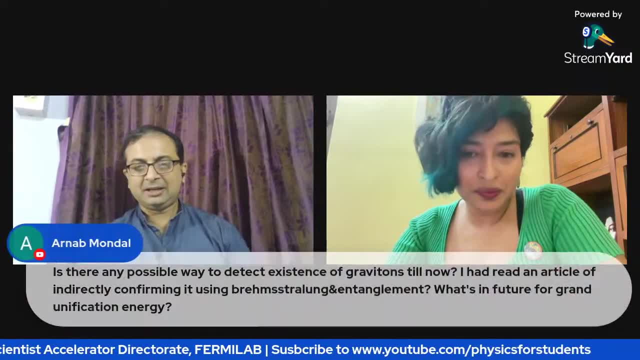 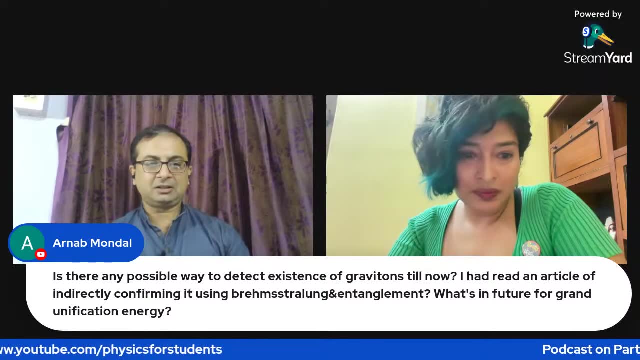 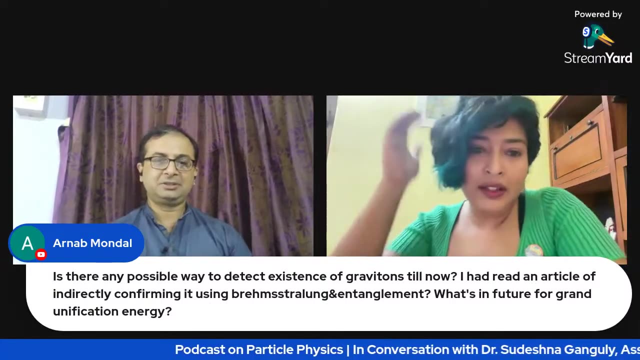 I'm so sorry. I think we have taken this question earlier. Yeah, Okay, So this is a new question. Is there any way, possible way, to detect existence of gravitons? till now I read an article of indirectly confirming it using a Brahm Strongland and entangled. Yeah Well, I mean. 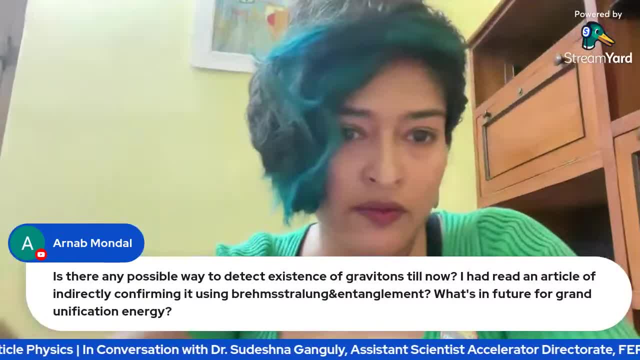 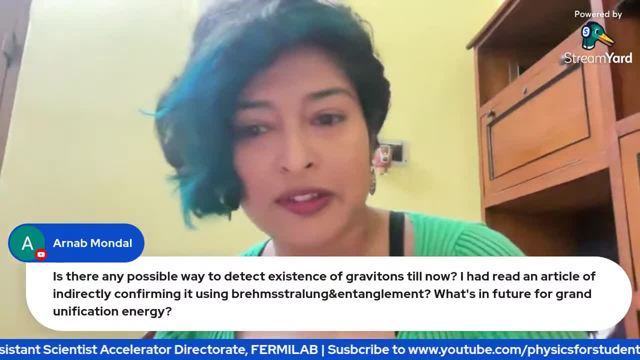 I cannot comment on gravitons. I know that there are like active experiments going on. I'm not part of that. But what is the future of grand unification theory? Yeah, we all want to see that. We all want to see GUTs satisfied. So there are like many, many experiments that are 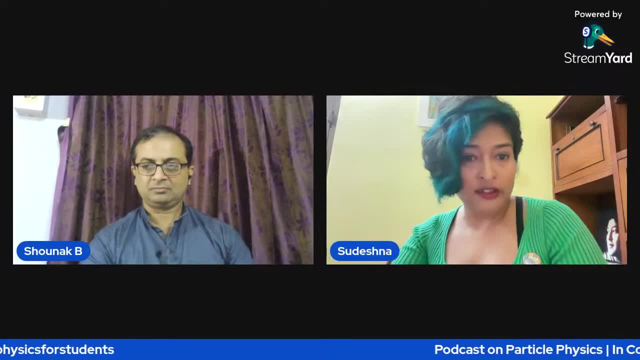 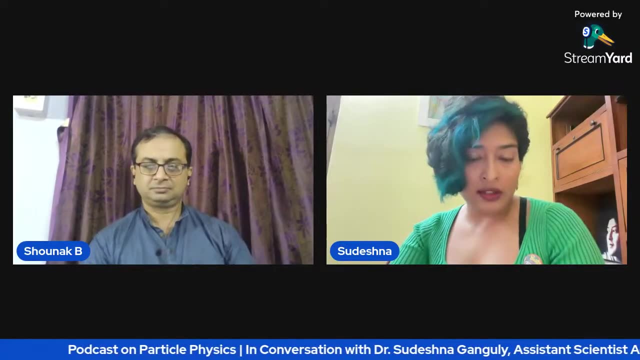 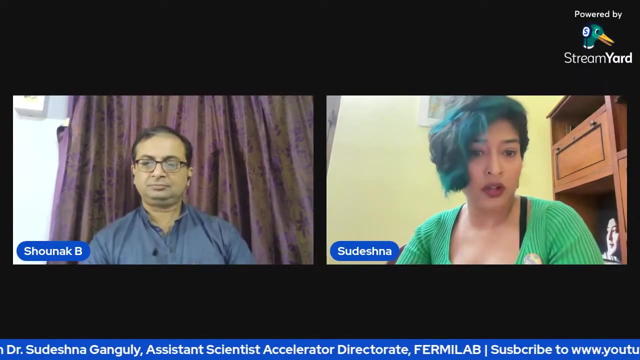 ongoing right now, For example, proton decay searches standard model tells us so it's not possible, but the gut hypothesis that they could decay in a very, very long time scale. so that's one example, like active research is going on in proton decay searches, neutrino science overall. so that would give us a very good handle, you know, with upcoming 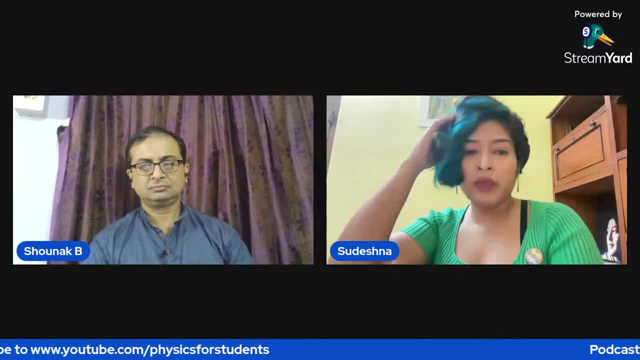 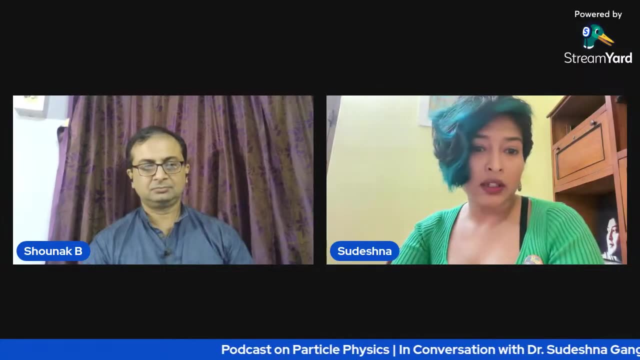 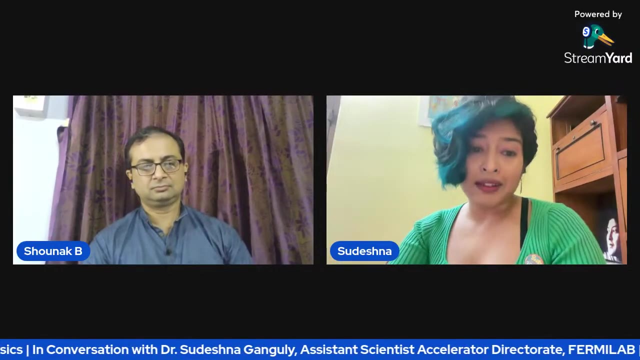 dune experiment, neutron oscillation experiment and many other different duty parameters could be uh verified or or satisfied like whatever theory is predicting um any. any like intensity frontier experiment would help answer gut questions. but again, at this stage this is still a hypothesis. we do not have conclusive evidence from experiments. but these are extremely difficult. 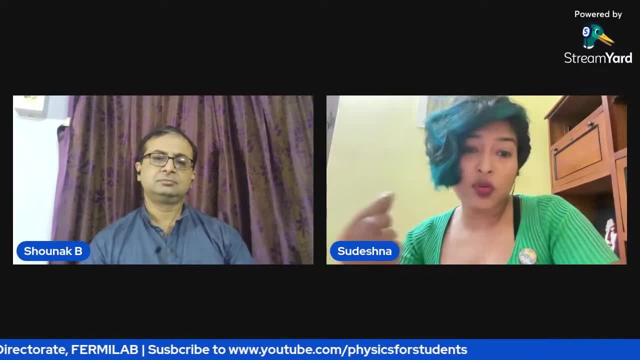 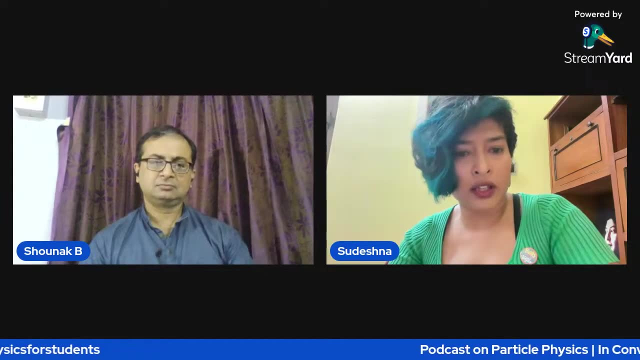 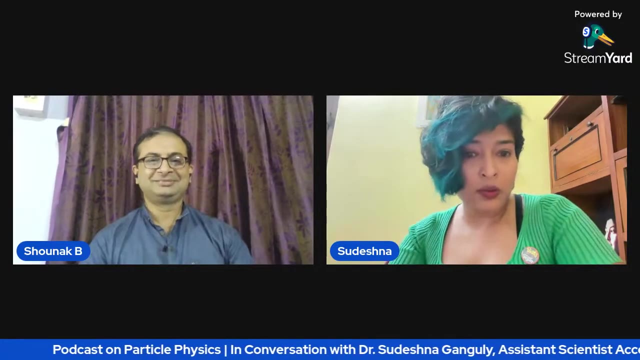 experiments extremely difficult, like for g minus two is just one, one parameter value we're trying to measure, and that requires so much hardware, so much operations and analysis and calculations. so these are not simple. so i'm hopeful. i'm hopeful, maybe in 40 years we'll have more evidence. 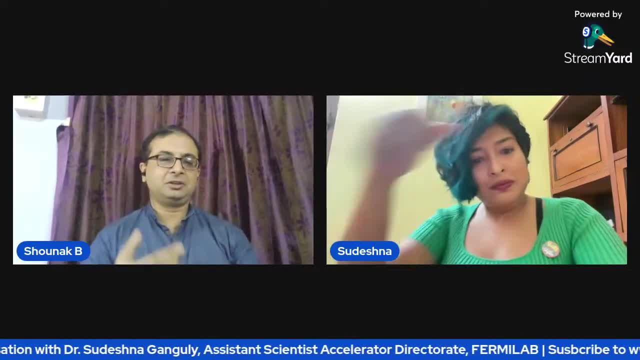 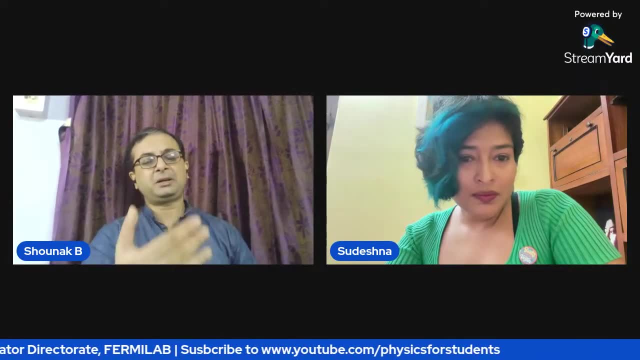 right before i go to the next question: uh, your, uh, this statement that you told that these experiments are difficult. i mean to say as a career aspirant, for example, somebody who wants to become a particle physicist and maybe work with or under with you in the vermi lab. we all know. 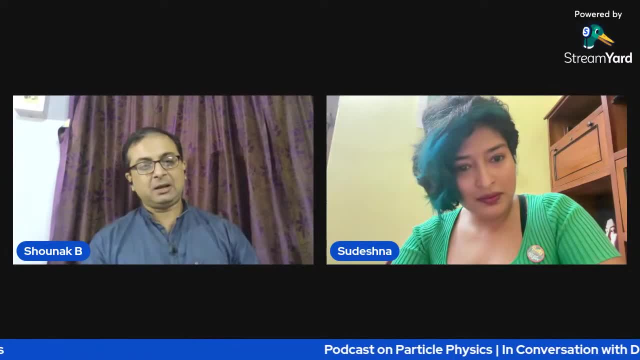 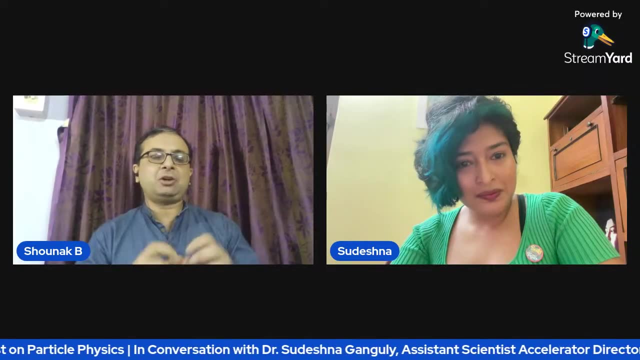 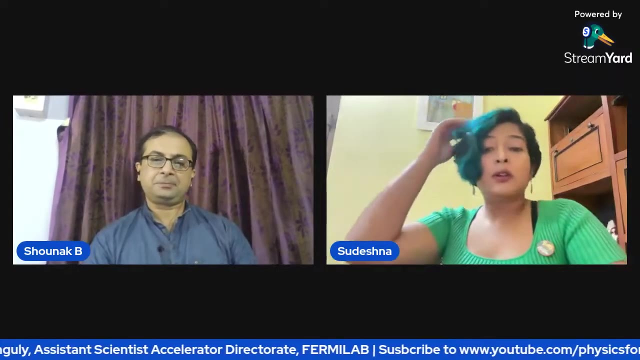 that physics is dominated primarily by mathematics, but especially for particle physics, acceleration, or the type of work that you do, what is, uh, i would say, what is the type of mathematics that someone has to be, you know, very good at, it's okay, so. so, if you are, if you are trying to do, 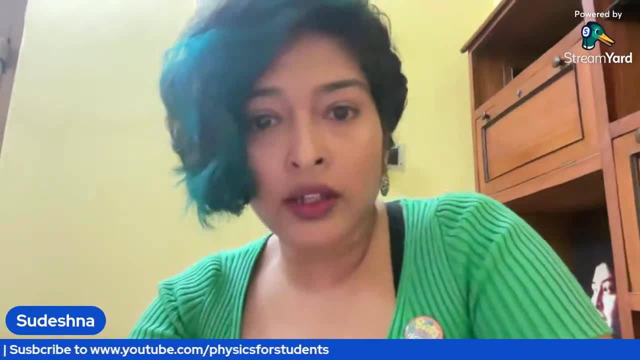 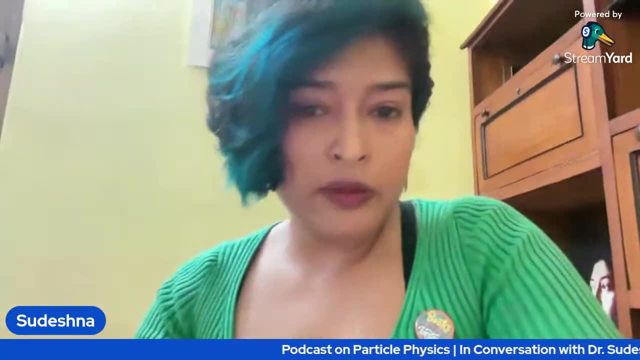 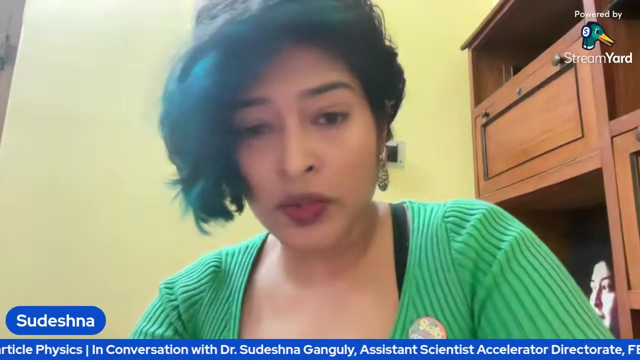 if you're trying to go to theory, if you're trying to become a theorist, then you would have to do many more mathematical calculations. you have to quantum field theory, uh, in as an experimentalist, our day-to-day work. so it contains uh, three different areas. hardware will have to be able to build very sophisticated hardware instrumentations. 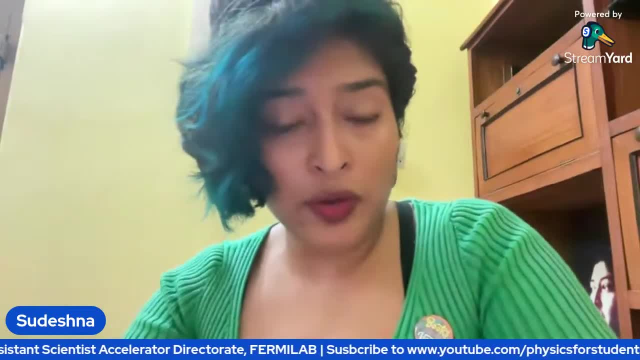 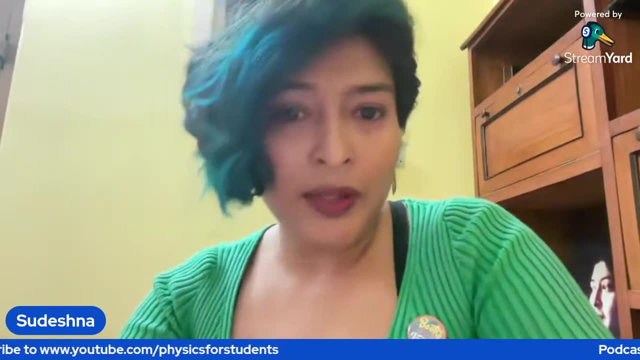 machineries, because all these will have to work before you can collect data. otherwise you have no data. if you know, if you have no data you cannot analyze anything right. and then if you don't analyze anything, you don't have an experimental result. so you cannot compare that with theoretical. 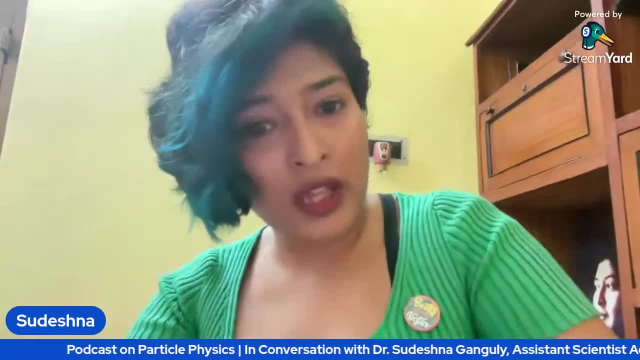 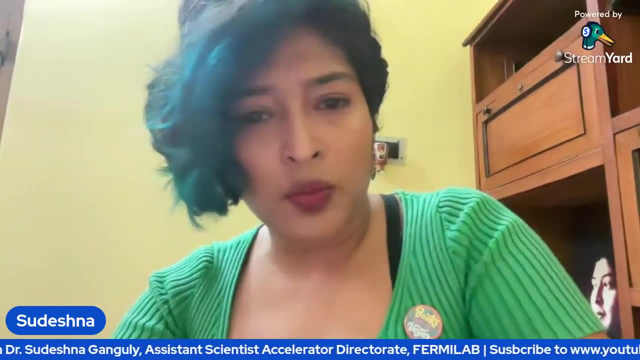 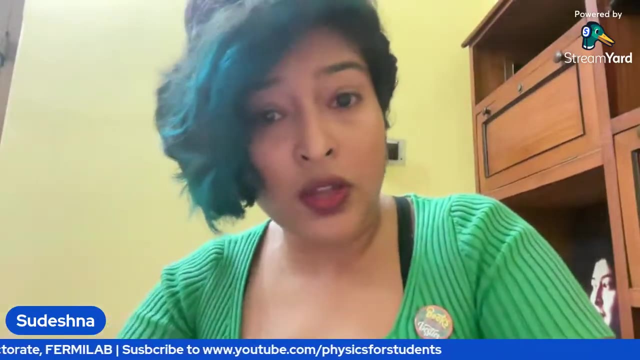 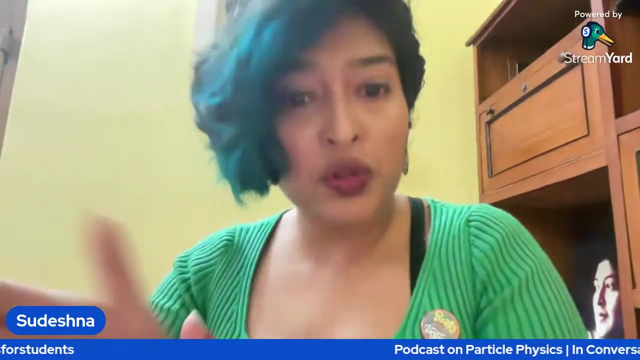 prediction. so the hardware is extremely important. so that's one part. so now we have machines, so you build machines. you have to operate them. so operations is extremely important and it's super difficult. operations means day-to-day running of all these very, very complicated machines together. so there are many, many groups of experts so we'll have to work with everyone together and make smooth. 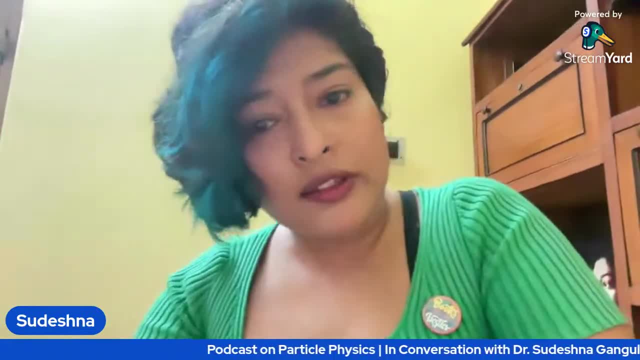 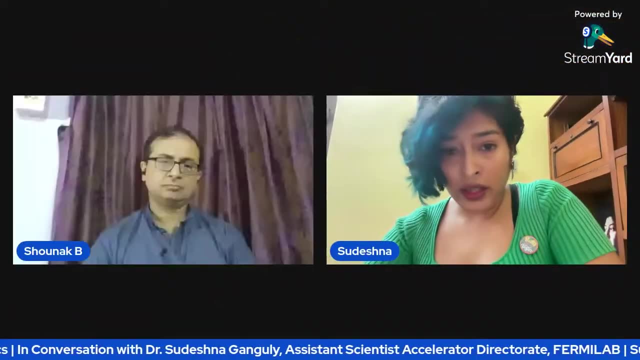 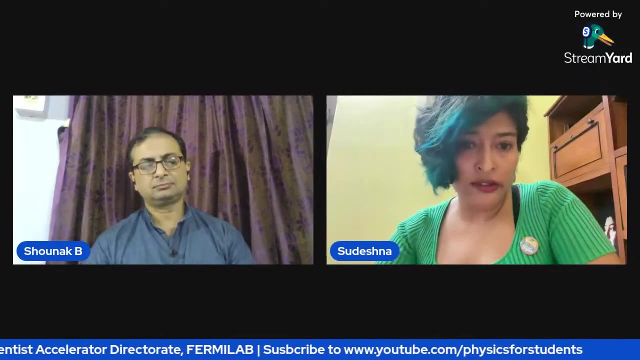 running of this machine. so that's operations and then analysis. so all these different detectors are collecting different data and for that again, you're not going to do like handwritten mathematics, you have to write code. so you'll have to be very, very familiar with the latest coding languages. 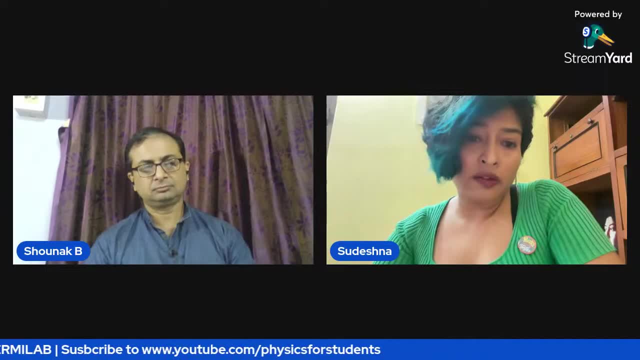 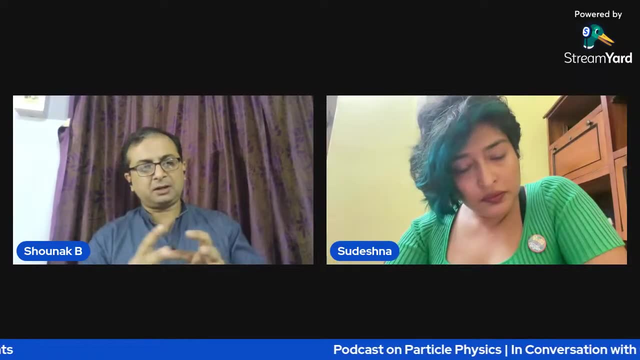 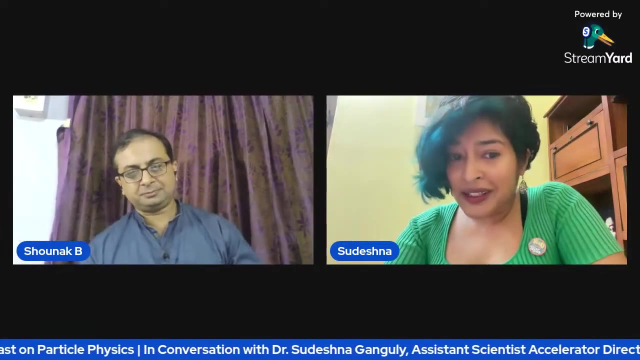 softwares, etc. so, and, and that takes a lot of sophisticated calculations, uh, coding basically. okay, that means hardware, that means, uh, your part and those you're working with the colleagues. they have to be more into designing of machines rather than doing everything in all three, okay. so on g minus two. i started doing analysis. 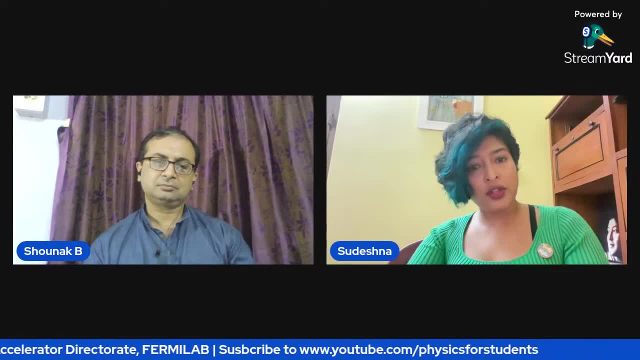 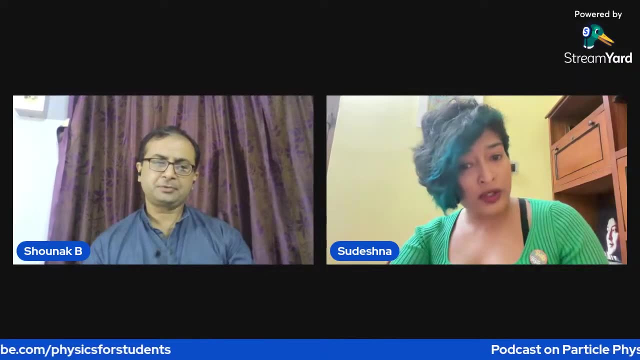 this where i developed the muon loss detection algorithm. i developed an algorithm which other people are now using in the collaboration, so so that was that's how i started. worked on the data acquisition software. so that software part. then i worked on hardware. i worked on the electrostatic. 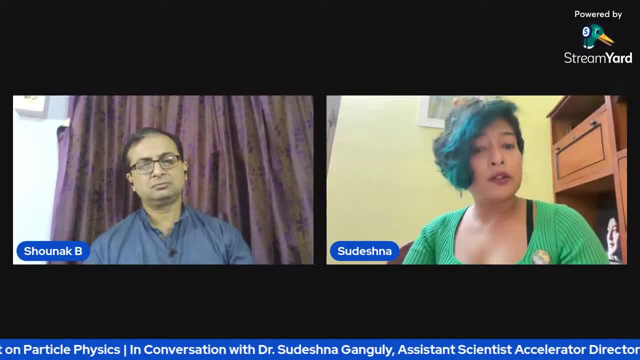 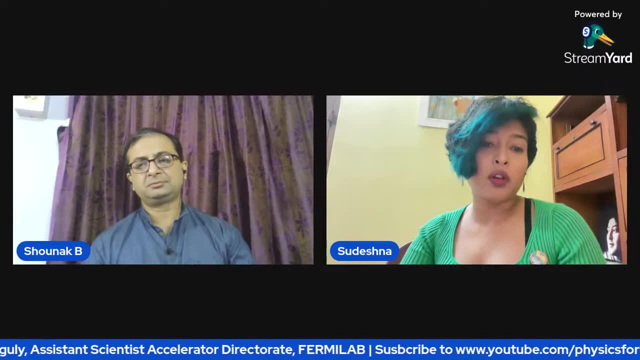 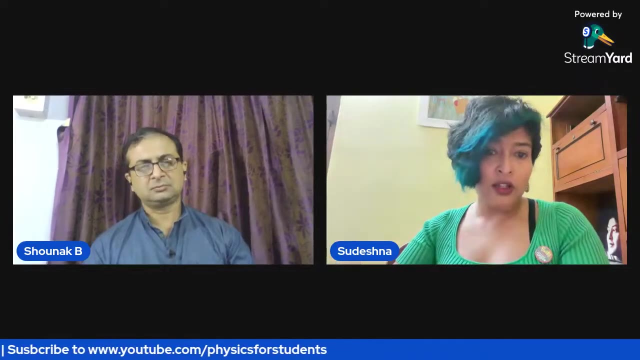 quadruples for the g-minus, to experiment these systems. and then i also became run coordinator where i was operation of like, operating the whole experiment, and then i became a run coordinator of the accelerator, the whole campus where my duty was to run all the accelerators. i just showed you all the machines running all. 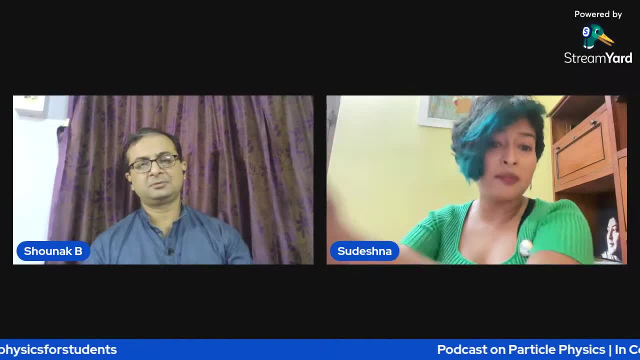 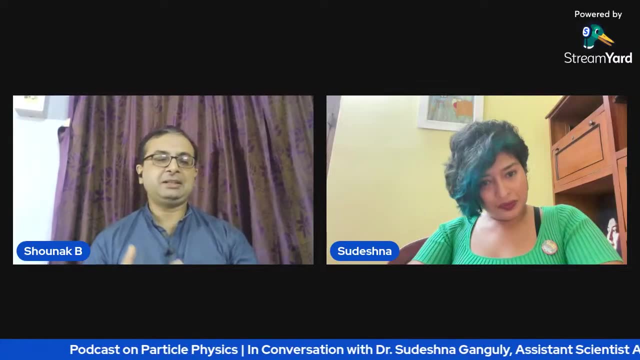 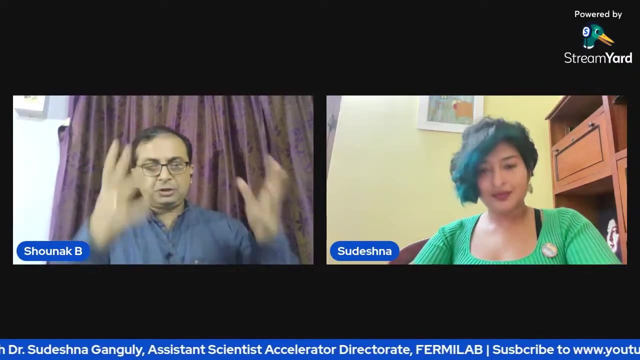 the machines smoothly, then you're making sure that you're giving beam to the downstream users, otherwise nothing is going to work right. so that means, uh, my, the basic intention of my question is that purely mathematical or pure mathematics doesn't exist. it is more of a instrument. 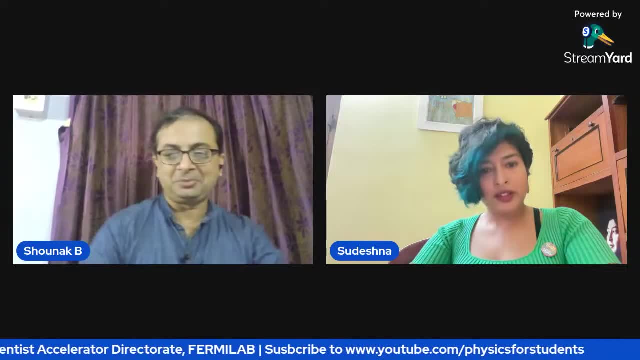 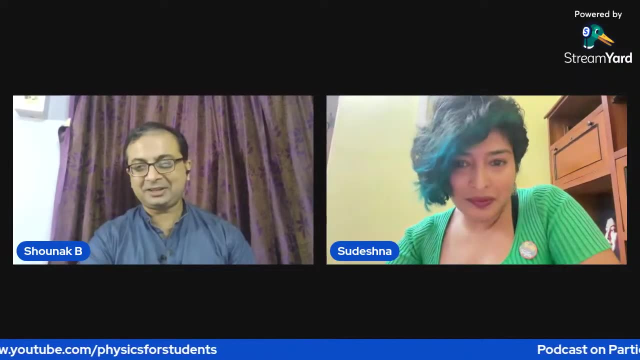 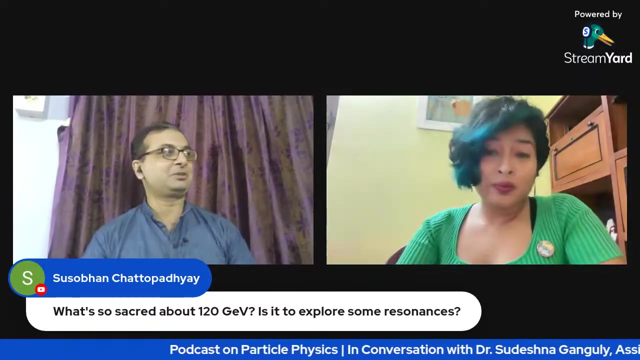 wires and things which are happening. okay, yes, and coding, a lot of coding as well. coding, yeah, okay. one interesting question before i go to the second question. author is asking what is so sacred about 120 gev? is it explore some resonances? so 120 gv that was built. 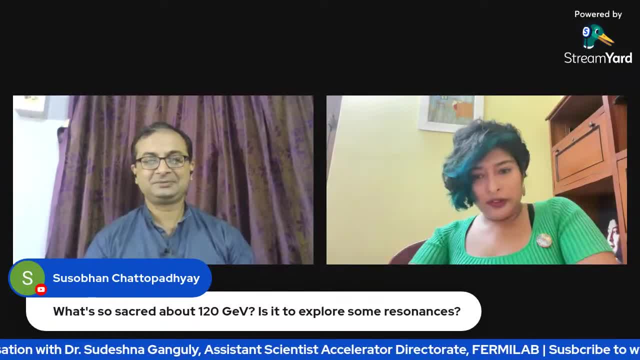 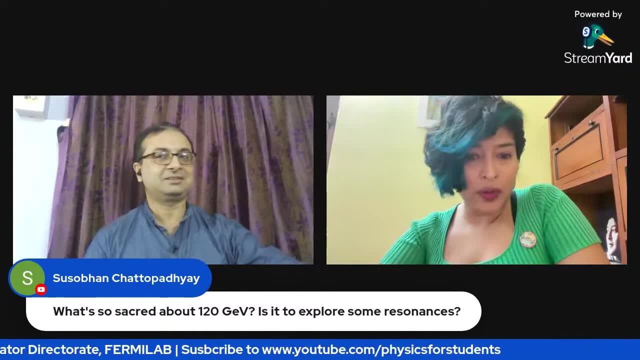 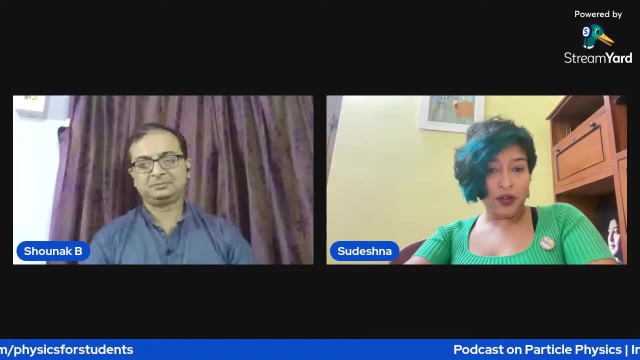 for a new me, the neutrino main injector. so so, whatever the range- uh, the neutrino solution range they wanted to look at, for that we would have to start with 120 gb proton beam and and, luckily, the for lbn. if so, that was my design for new me science. we needed 120 gv and that was within the 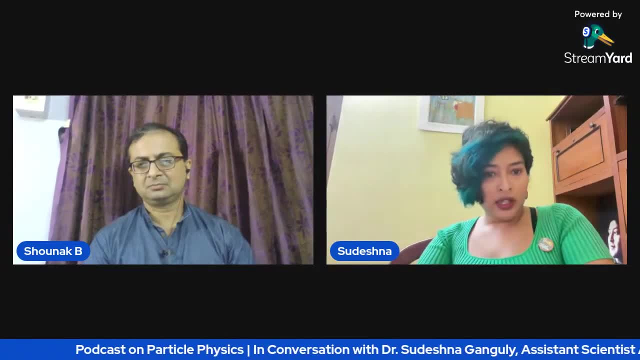 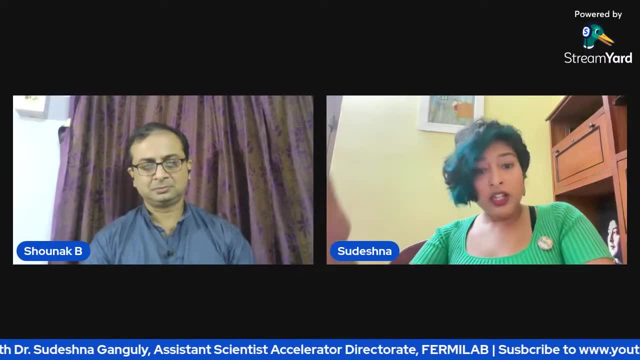 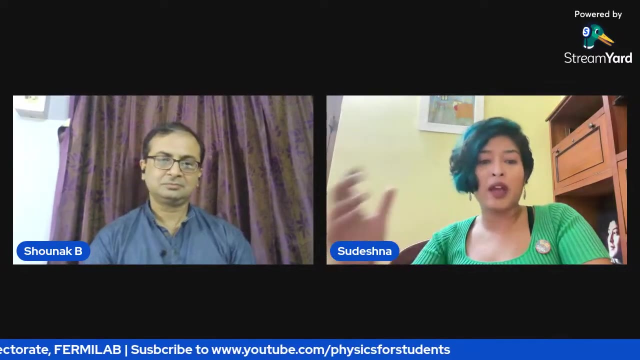 reach capacity of the technology at that time when new me was built. and now for lbnf, we're going to use the same beam because we don't want to investing to go up in beam is a lot more investment, so that's like that's unimaginably large number. so so for lb, and if that's why we're lucky, we're. 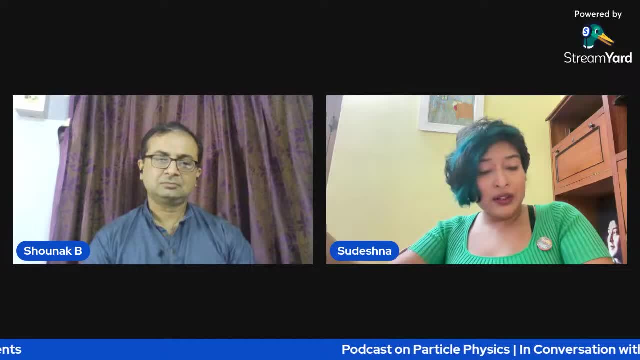 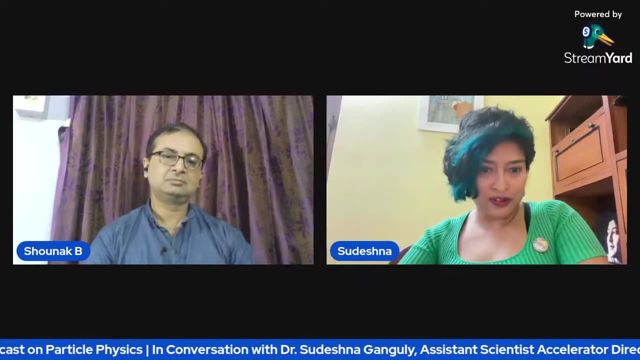 going to use the same beam. we're going to use the same beam. we're going to use the same beam. we're 120 gb beam, but we're in increasing intensity or increasing beam power. we're creating more proton beam. that way. you were trying to create more neutrinos, you know, but that was by design. 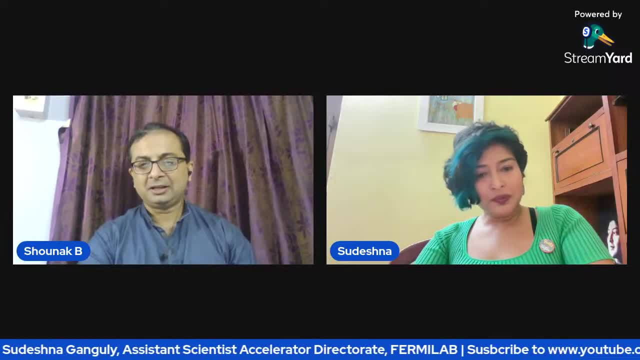 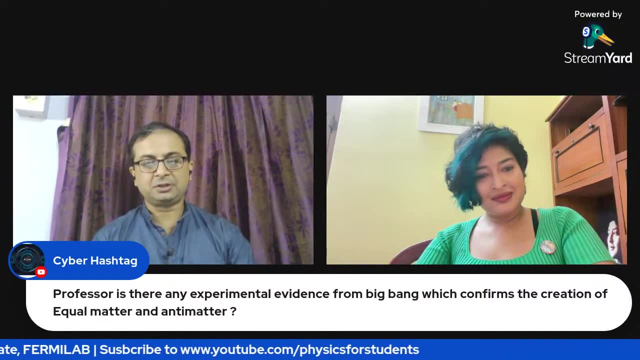 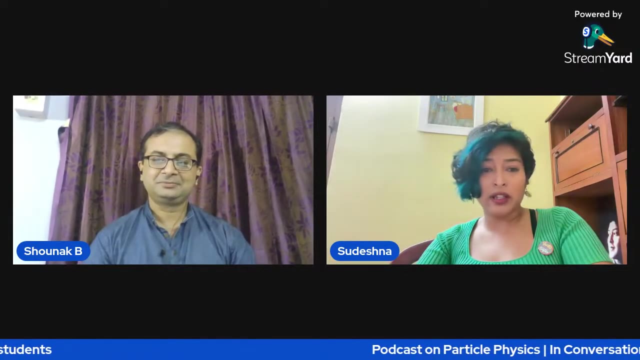 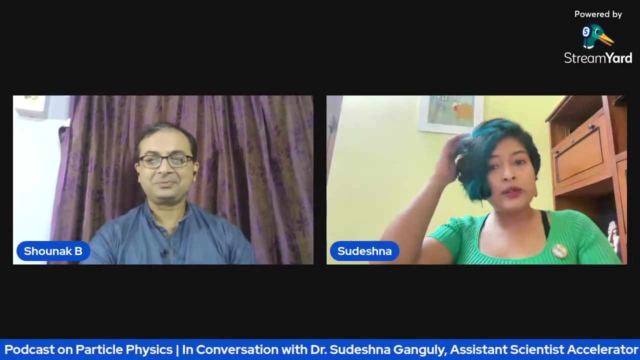 basically for new me: okay, okay, okay. cyber hashtag got. what a question, professor. is there any experimental evidence from big bang which confirms the creation of equal matter and antimatter? no, equal matter, antimatter. shouldn't have happened, then we wouldn't be here. then we wouldn't be here, but but we. the point is, we don't know why there is more matter than 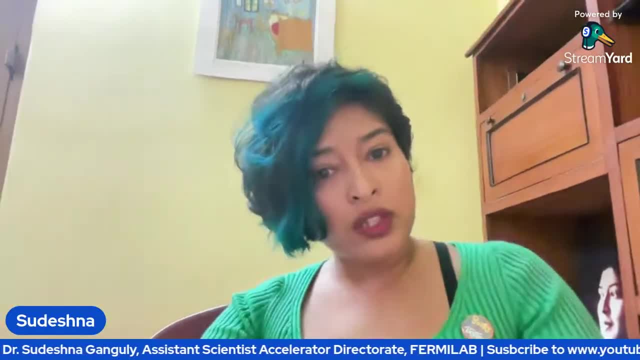 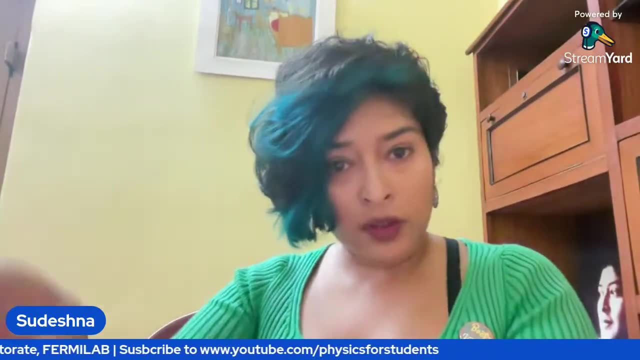 antimatter. it's still not understood, and that's why we need all these experiments: to look for physics beyond standard model, because maybe by by looking at the results from all these new experiments, we would be able to put the dots, connect the dots and understand something better. 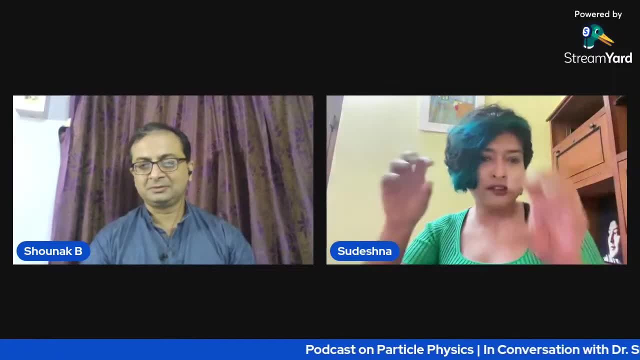 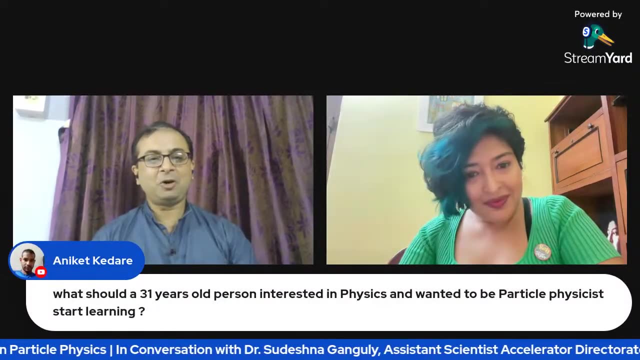 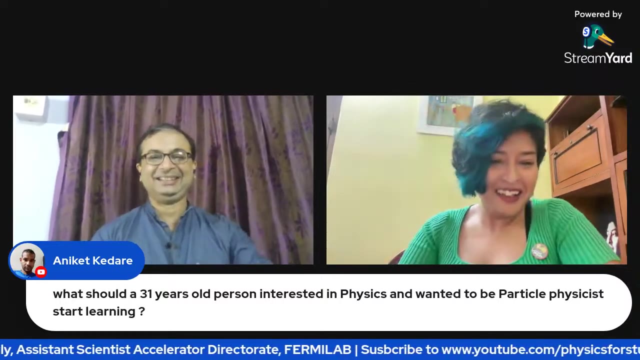 you know, it's like this jigsaw puzzle and there are so many pieces missing, yet you- yeah, aniket has got a very interesting question. what should a 31 year old person interested in physics and wanted to be a particle physicist start learning? what you should start learning? 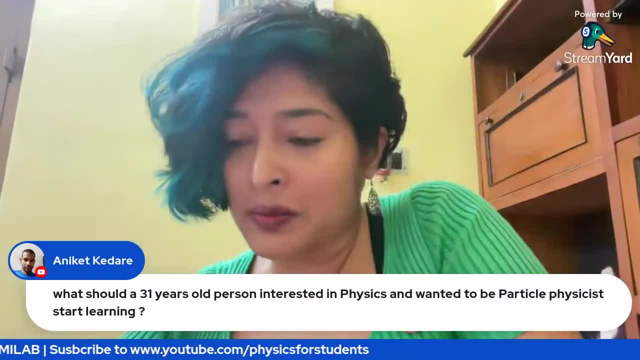 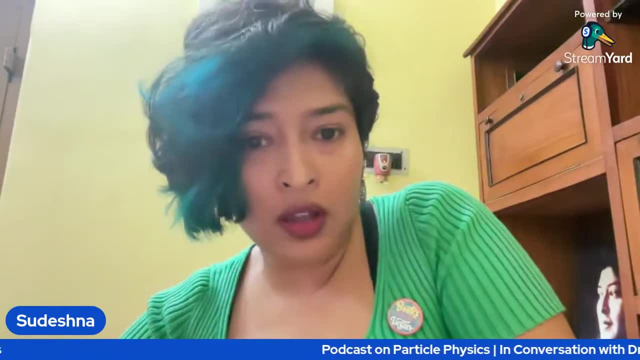 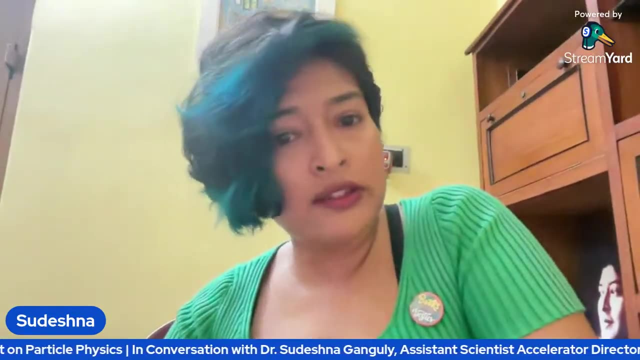 well, i mean, oh yeah, there is a very good um resource actually on youtube. um, if you're interested, formula is don lincoln. he posts a lot of videos, uh, on formula physics, like what we do the most british raisers, just like sohbhan and other astronauts do, since amps are extremely 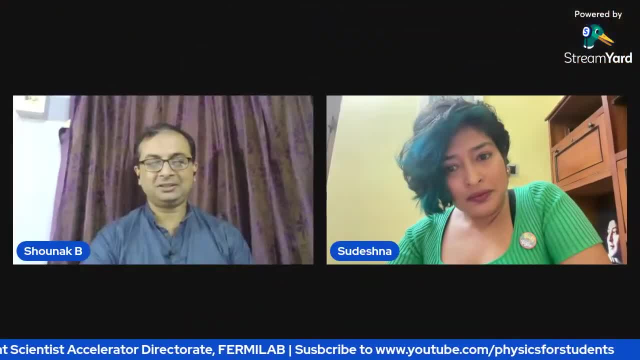 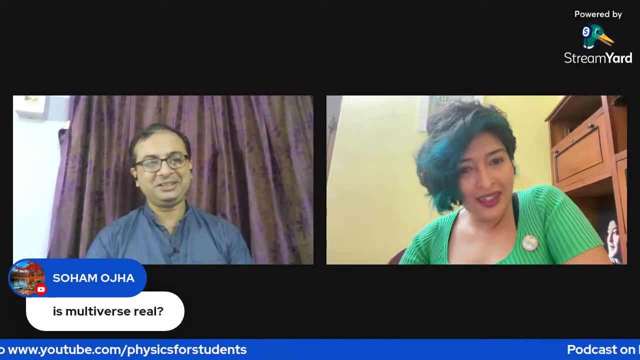 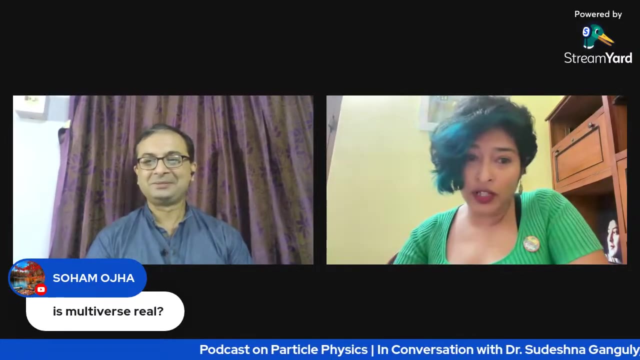 entertaining and easily accessible so you could start watching those videos. actually, yeah, uh, one question from sohum oja. i don't know whether he will take it or not. is multiverse real? i cannot answer that. i i wish it is, i want it to be, but i i cannot vouch for it. 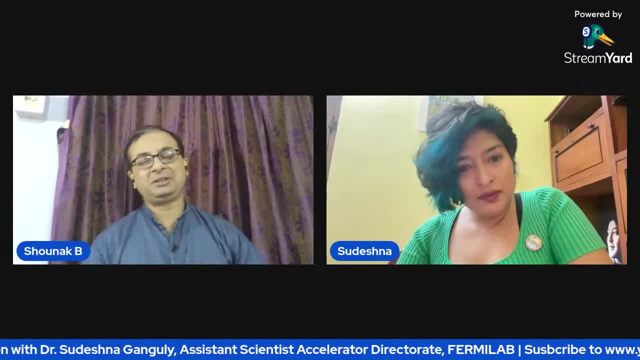 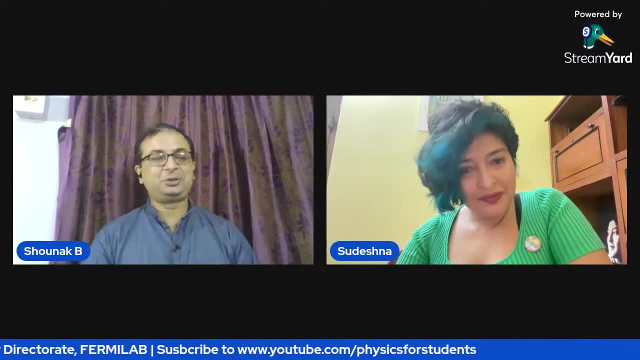 what i would like to know a little bit from you. this is have been the way the first time when i contacted you- is that when you walk inside your fermilab- i mean to say if you can take us a virtual tour- how do you start your day, what you do and what exactly are things around? so i first, when 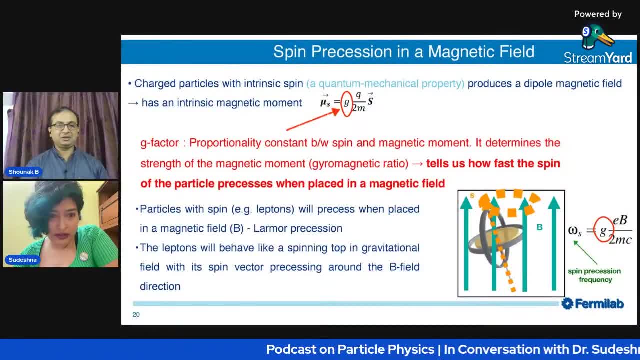 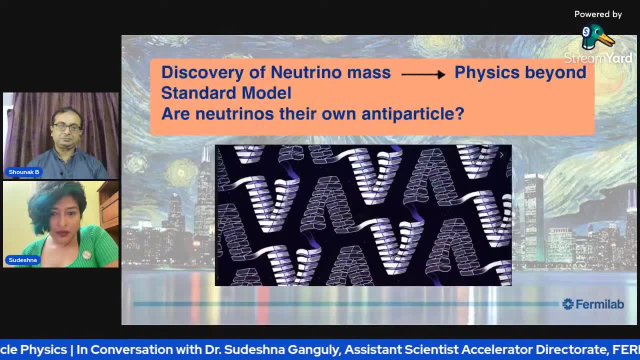 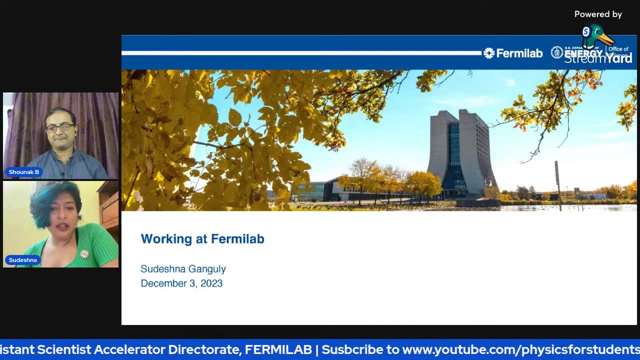 i go there. can you show me my slides? yeah, so i go to this building straight on my first slide. where did it go? almost there here. yeah, so we come from this side, walk down this path. this is called wilson hall, so this is just where all our offices are and our cafeteria: big atrium on the first floor. 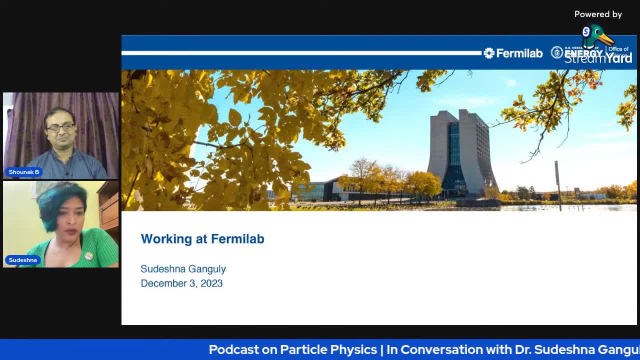 so we just go there, grab our coffee um, sit down, chat with our colleagues a little bit and then we scatter to our offices. but the actual experimental halls are scattered all over the area. you can see like tiny buildings here, like the outline of the building, that's. that's the 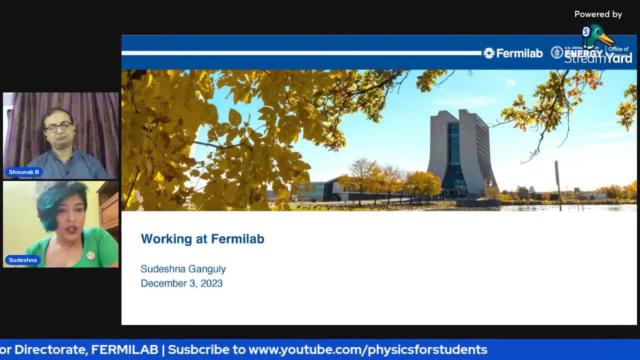 experimental hall of muon g minus two. so then, so actual experimental halls are above ground and they are located in different locations. the enclosures which contain the accelerators, they are underground and they are like strict, stringent, uh security rules to access those. we cannot just like go in there because it's radioactive and it's highly hot, so we cannot just go in there. 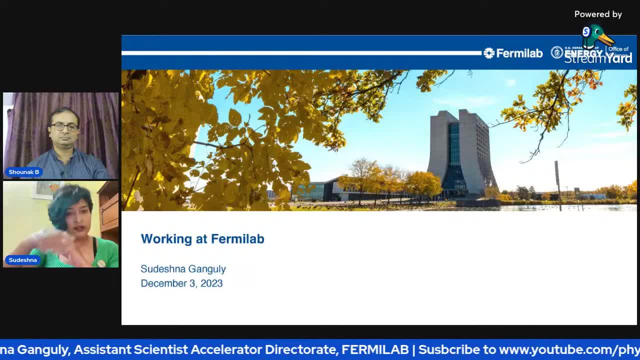 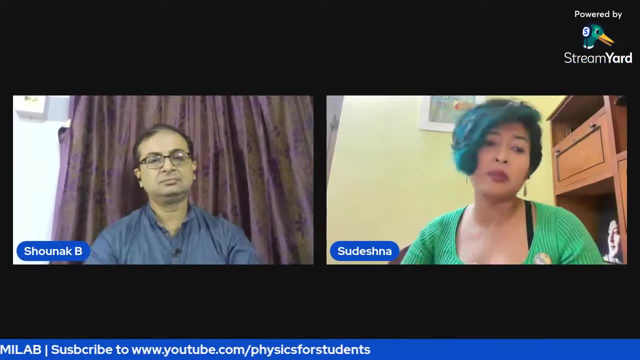 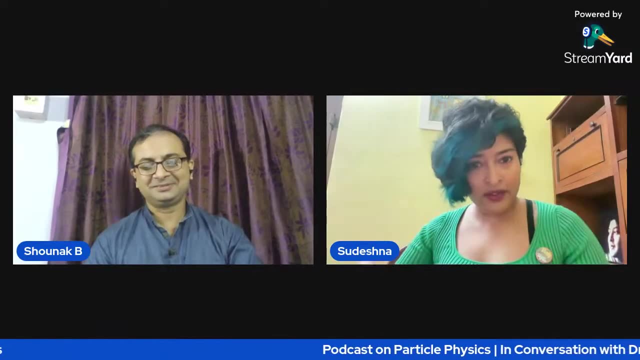 but above ground halls are in different areas and then then we have access points to this underground accelerator and during summer shutdown we make access and that's super exciting. so we have to like, take keys and follow all these procedures, wear hard hat, take our safety tools and then searchlight etc. and then 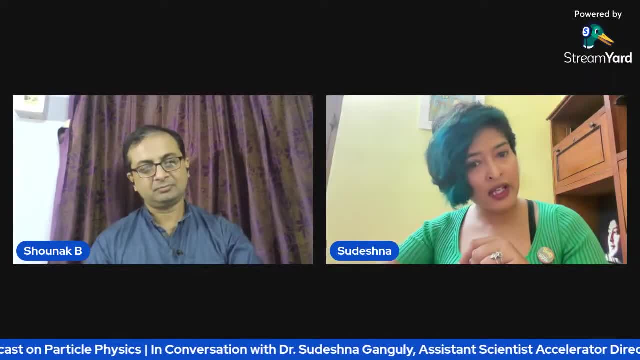 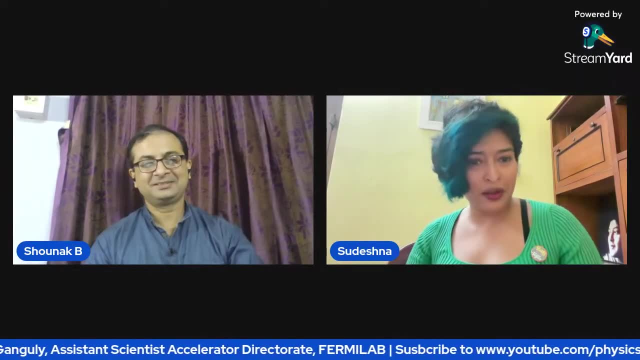 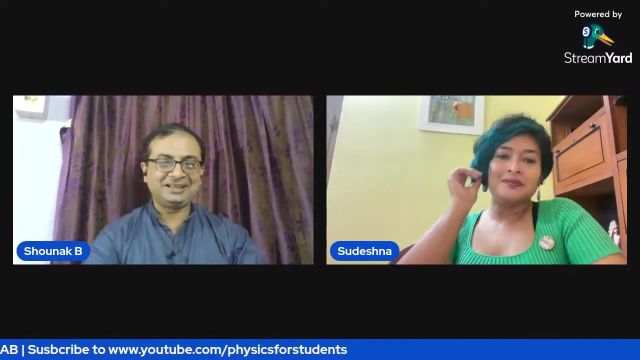 we'll take an elevator underground, like eight floors down and dark tunnels. we'll walk down there, we'll work on some machines, take some measurements etc. and then climb up. so super exciting. we do that in summer when beam is not running. okay, that's great. i mean to say 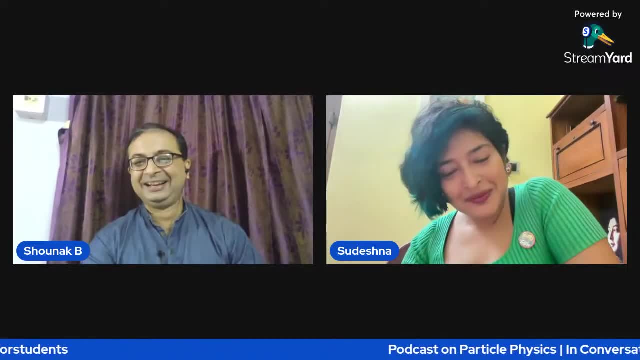 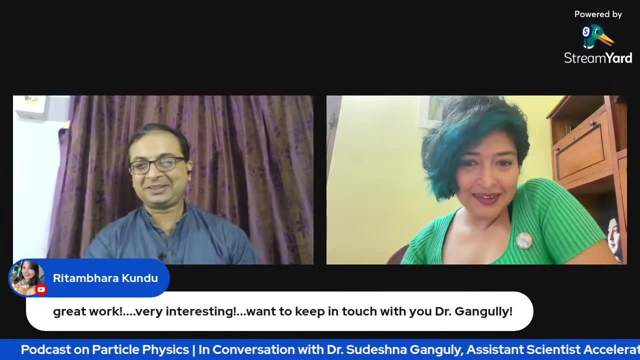 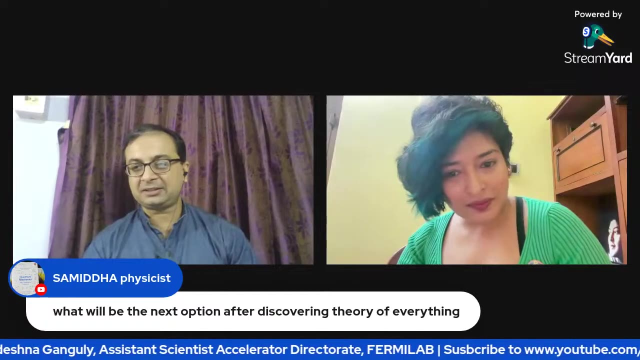 you made a virtual walkthrough to that. okay, uh, uh, uh. ritam bharat kundu is telling great work, very interesting. want to keep it in touch with you, dr ganguly. okay, there's one question is that? uh, what will be the next option, samitha is asking, after discovering theory of everything. well, i mean. 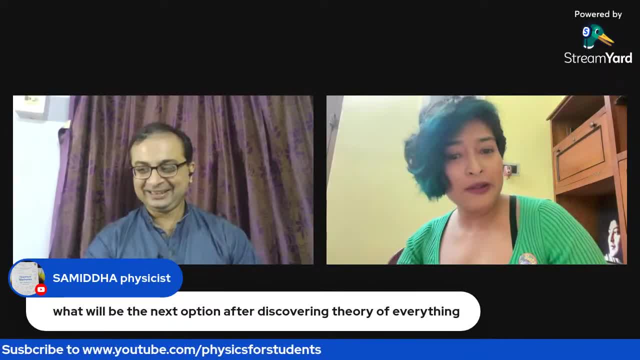 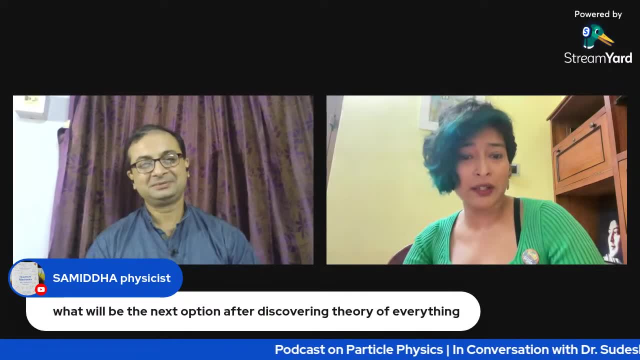 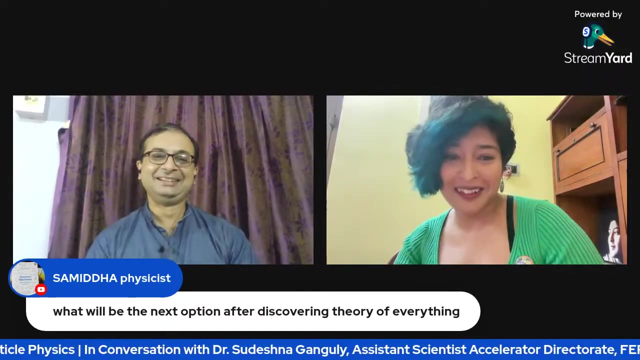 i don't think that's gonna happen anytime soon, but suppose we understand everything, then i guess we will rule the universe. who knows, if we understand everything, then we will have immense power. i, i, i am scared of that. probably that will not be a very good thing, absolutely, uh, actually. 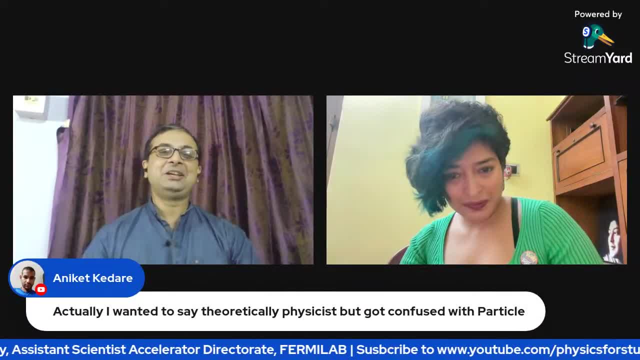 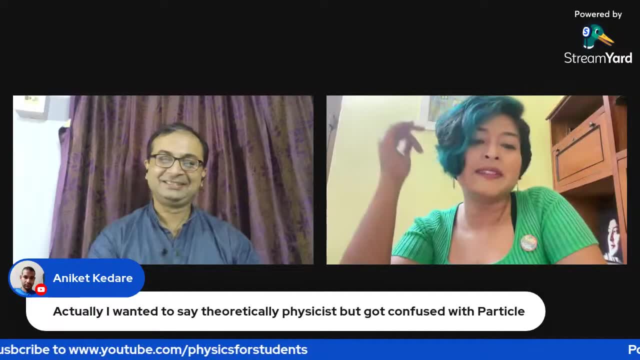 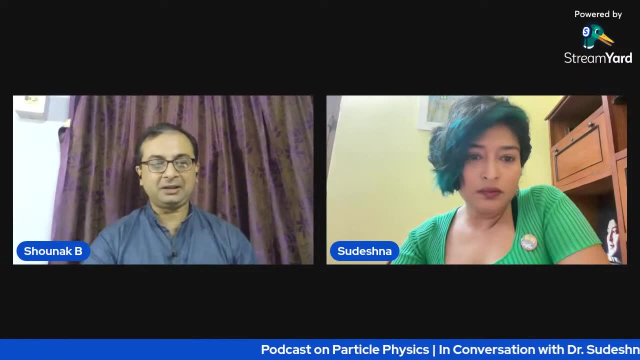 aniket wants to convey this message to you. actually wanted to say theoretically physicist, but got confused with particles. yeah, yeah, so i, i assume that's what you're saying, that's what you're meant. yeah, right, uh, dr ganguly. uh, the moon g2 experiment. what exactly that you're doing? i will. 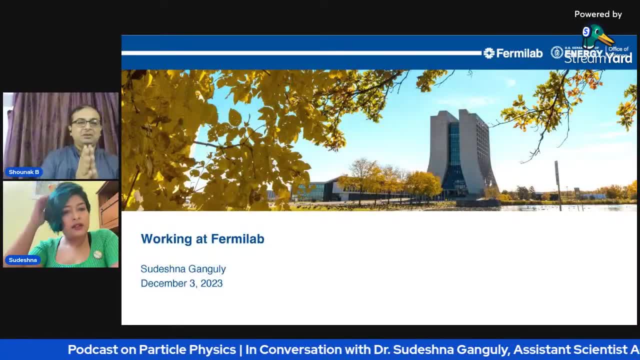 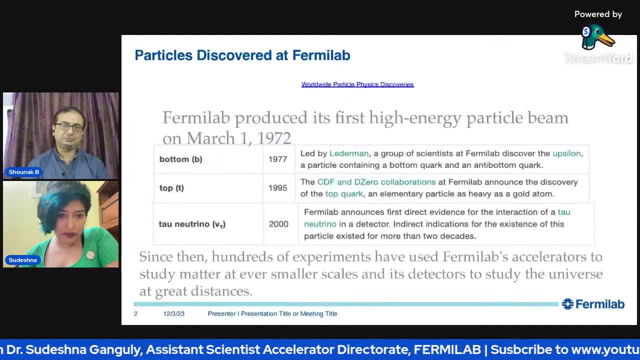 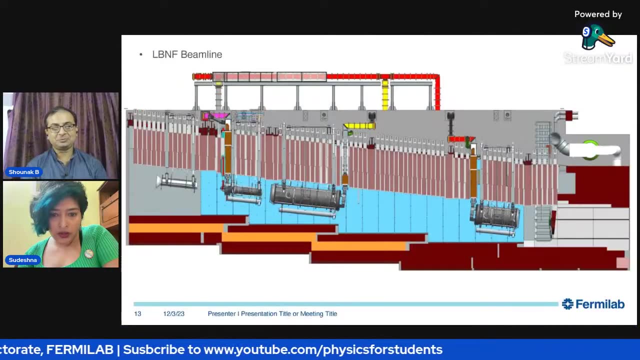 just put on this slide. yeah, we would like to know exactly what this more g2 is trying to prove and what are your words right? and then i wanted to show some pictures as well. i have, like, some really fun pictures of the actual experimental hall, our beloved g-2 ring, so let me go there. 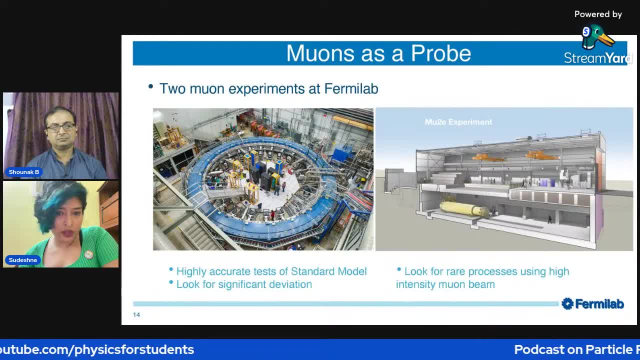 yeah, so so these are the two neon experiments. this is a picture of our actual ring um with, taken with the drone from up, and we worked in here on this uh area, on this platform, many, many summers, like many hours um, amazing work, uh. so this is my friend. 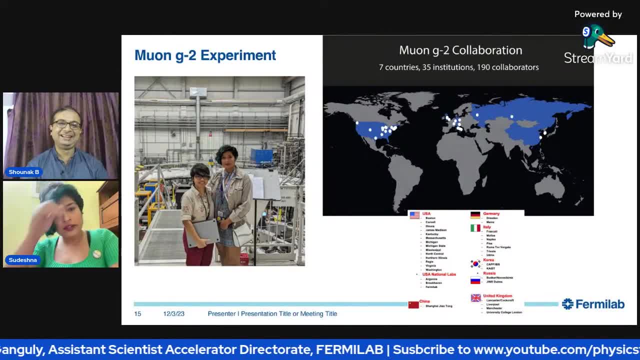 magna. she was also bengali, so we worked together on this experiment. this is our experiment. so we walk down the staircase and go down, and then we work inside the ring. and this, the ring that i'm referring to, the ring that's actually the magnet, a superconducting. 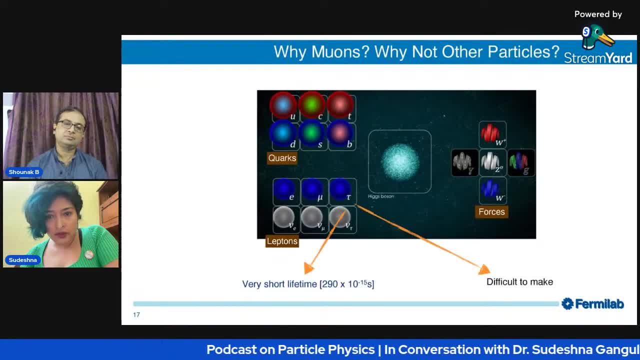 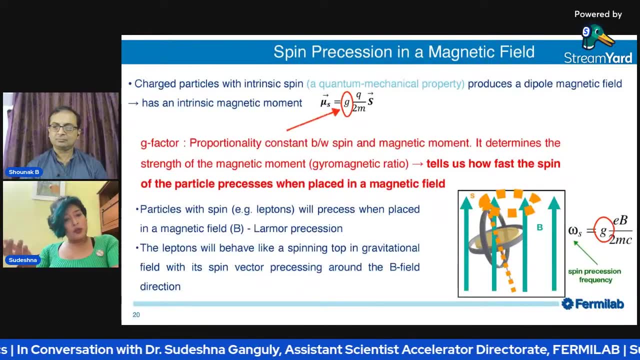 magnet, you know, and that stores the muons. so i will just briefly tell you what we do in the experiment. okay, we we try to measure the name g. g comes from here. so the question about spin, that was a very good question, uh, so so g quantity is related to the spin and it tells us 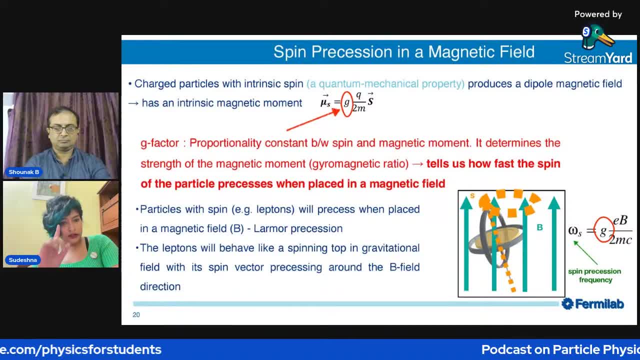 this g factor tells us how fast the spin. the spin is processing around the axis of the magnetic field. so we have an external magnetic field, we put a spinning top and then the spinning top is precessing around the, the, the direction of the magnetic field, right. and then g factor tells us: 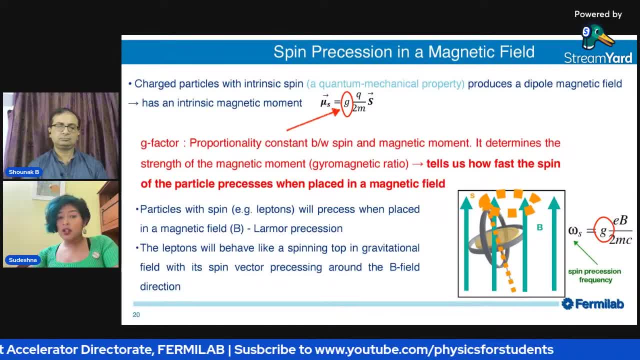 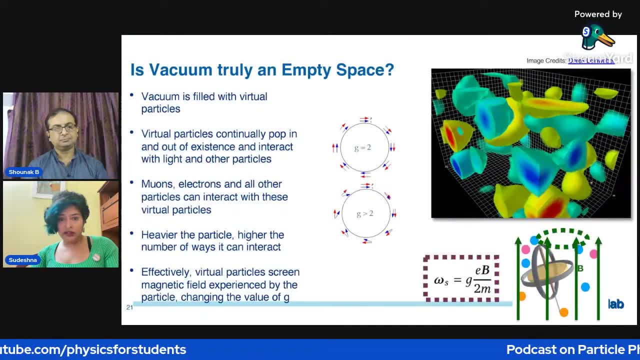 how fast that happens, right, okay, so now if quantum mechanics did not exist, then direct said g will be exactly equals two. if quantum mechanics did not exist, so this would be the case when the spin and the momentum will be locked in, it will not precess. so g is not exactly close to. so the spin is processing as it goes around the ring. it's. 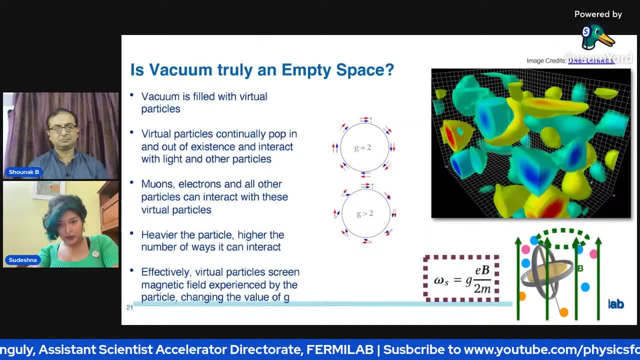 precessing, so. so i can't play the um animation here, but i can just explain briefly. so when we think of vacuum, is it truly empty? no, it's not truly empty, so it is filled with virtual particles. they're coming in and out of existence due to quantum mechanics. it's like a soup of virtual 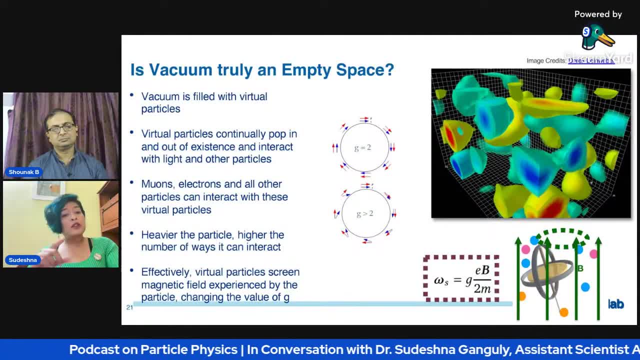 particles. it's just continuous fluctuations, right? so if some virtual particles exist in in soup that is coming to existence, interact with the muons and and screen the muons in a way like a spin, that its g factor changes, right, and this virtual particle is something that is not. 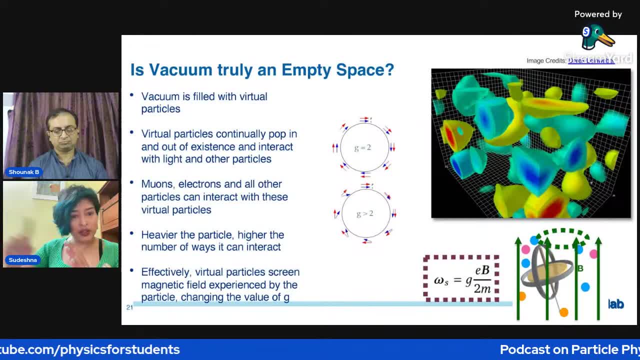 detected yet that's not known yet. so then the theory. what theory predicts how g will be different than two? theory cannot predict that, because theory doesn't know this new virtual particle, right? so theory predicts that g minus two will be x, but this virtual particle comes into play. 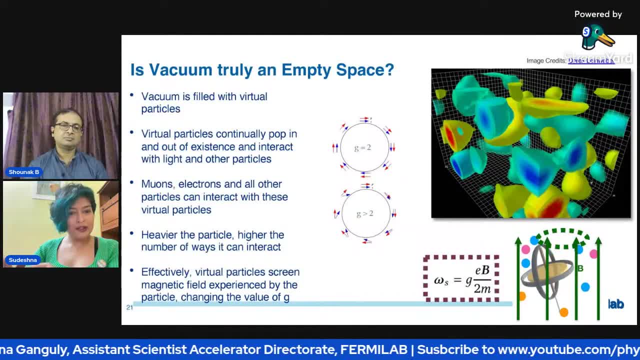 and says: oh no, g minus two will be x plus delta x. so this delta x is the interesting part. so if we see the delta x, then that tells us: oh, there is some new physics, maybe a new particle, new force or interaction that's causing the g minus 2 value to differ from what theory tells us. right, that's. 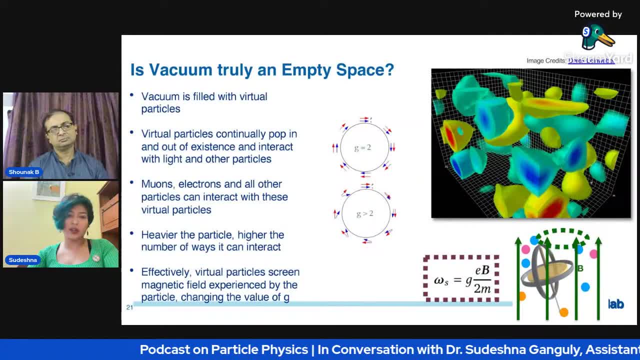 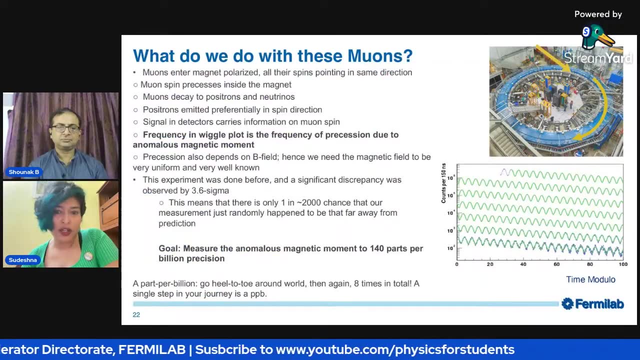 what is interesting. so we just try to measure this quantity, g minus 2, and hence the name of the experiment, and, and, and we try to show that this measured value is different than what theory tells us what it should be. standard model, right? so so that's the basic uh principle, and this is in few years time, i mean to. 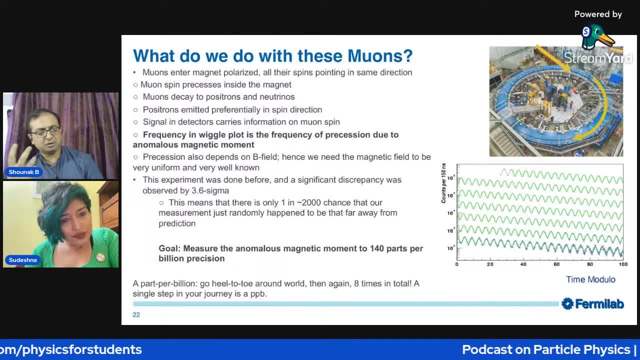 say: what you think is that we will? are we going to replace- because there are a lot of problems that are coming up- i mean just the limitations for standard model? it will. it will get, uh, improvised into something new. yeah, i mean, as we learn more, it will be more, more, more additions. 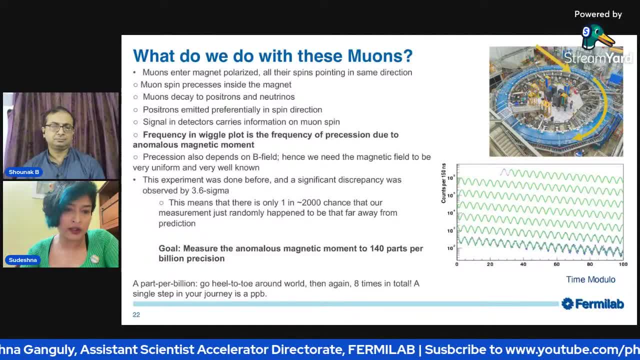 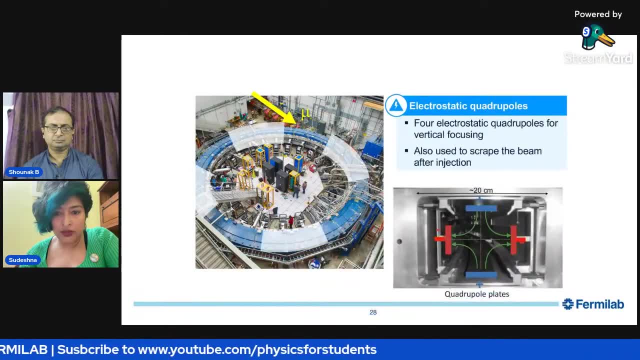 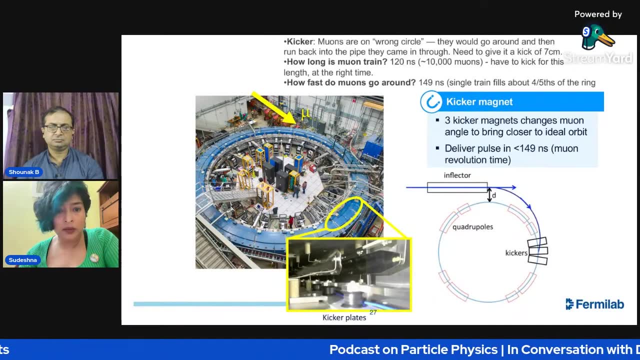 just would be: uh, attached to the standard model, like higgs was added, so we just need to have more proof. so so, briefly, i will just show the result of the g minus 2 experiment. so these are our rings and, like i said, we're just trying to measure one quantity but see like the complexity of all. 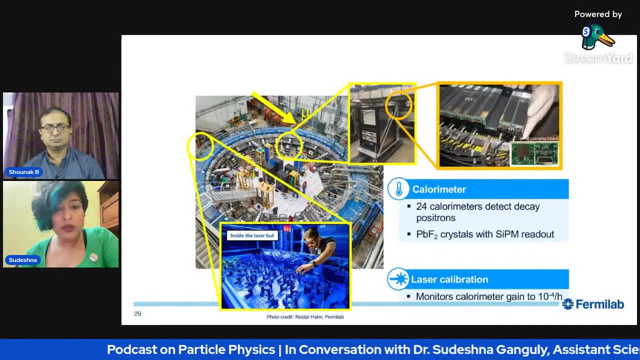 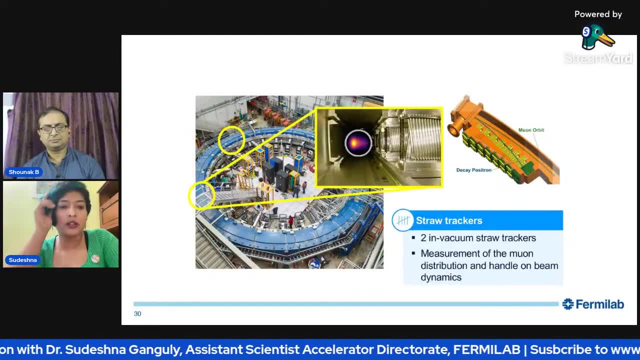 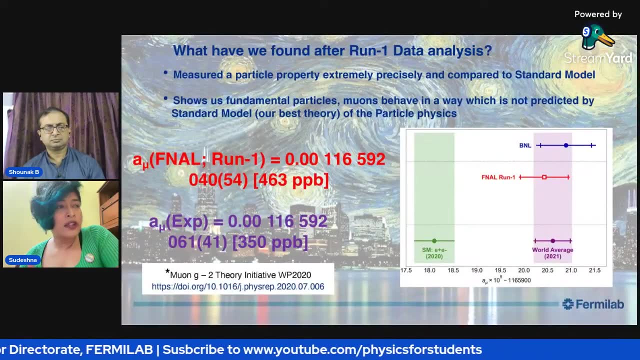 the machines, all the detectors for different purposes, and so we had many, many subgroups to work on each specific um like detector system, and that's a lot of work and not just hardware analysis operations, etc. right, okay, so so run one result. this was that happened in 2021, when we analyzed the run one data and published the data. 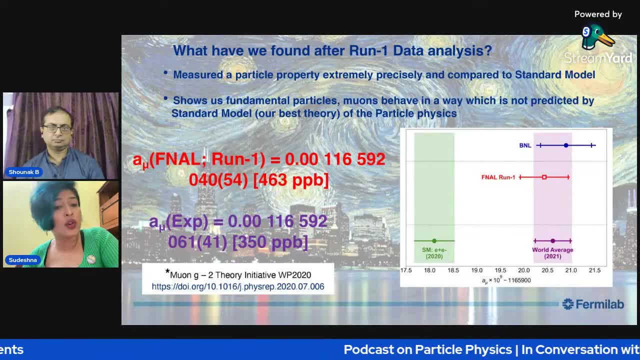 so what it tells us? this was the theory prediction in 2020 standard model. so theory tells us: the g minus 2 value, this amu quantity should be here, but our experiment showed it here and we had a prior experiment 20 years back. our senior colleagues worked on that. 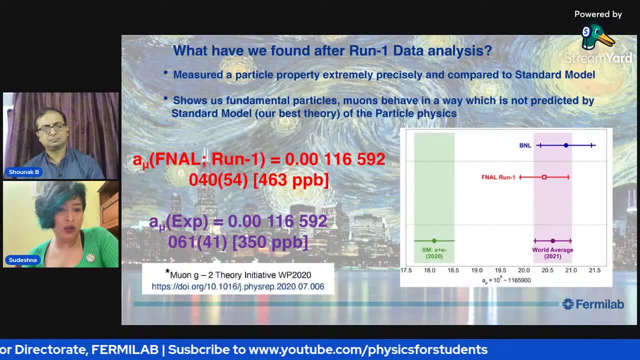 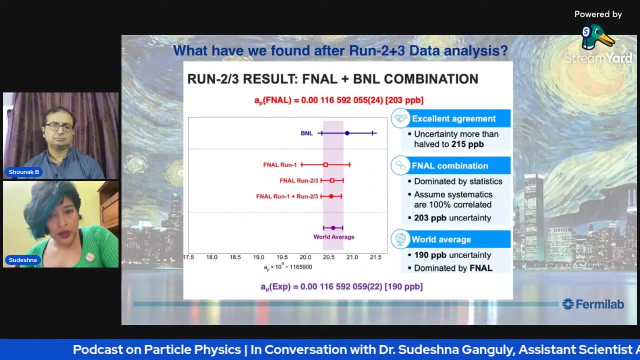 bnl brookhaven so they were also here. so combined those two, the experimental result here and theory tells us it's here. so it was 4.2 sigma this gap, and that was exciting, given that the theory prediction back then was here right now, currently with the run two, three. 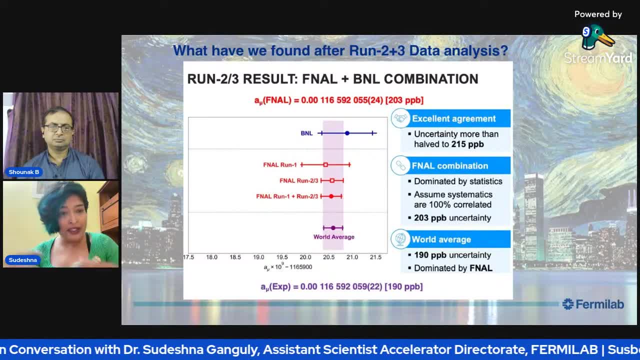 measurement, what we show we have done much better by adding more statistics. by adding more statistics to reducing the error. right, if we add more data, your error will reduce. so by adding more statistics we have reduced the error bar. you can see this has reduced. so right now we have the world. 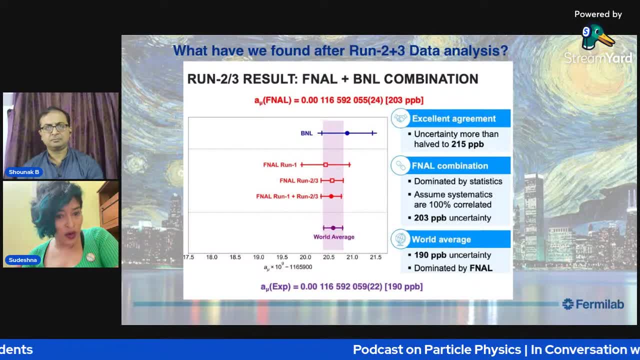 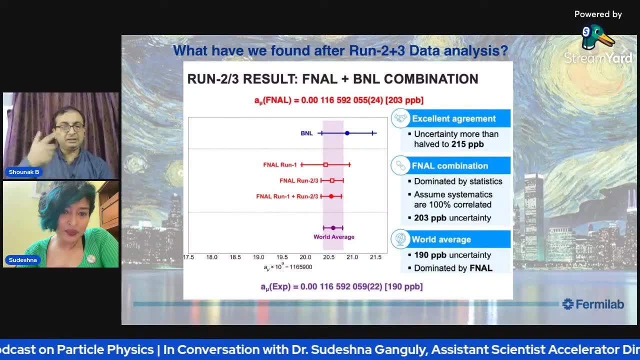 best average measured g minus 2 value so far as of now, and we are waiting for our theory colleagues to update the results. you are running how many times? so we have run six. we have collected data for six accelerator cycles- six years, basically. so we started in 2018, yeah, and then we just ended. 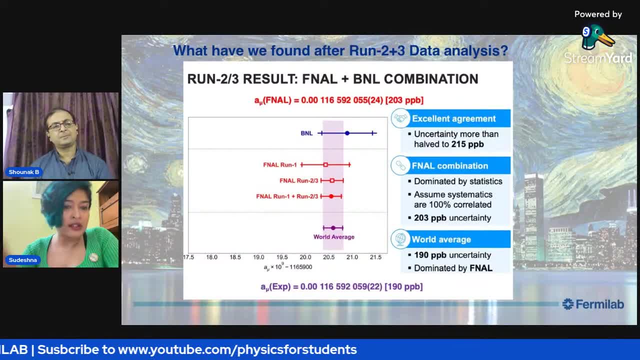 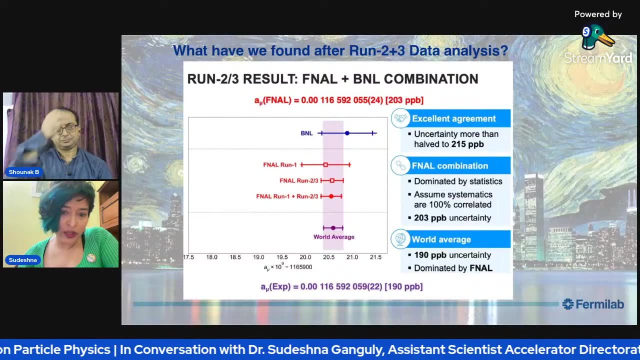 this year. so okay, so each year is one data run set. so so so far we have um analyzed up to 20, 20 data, roughly 20, 20.. so we have like three more runs to four, five, six to analyze, but we just three runs right now. we are dominating the world average. this is 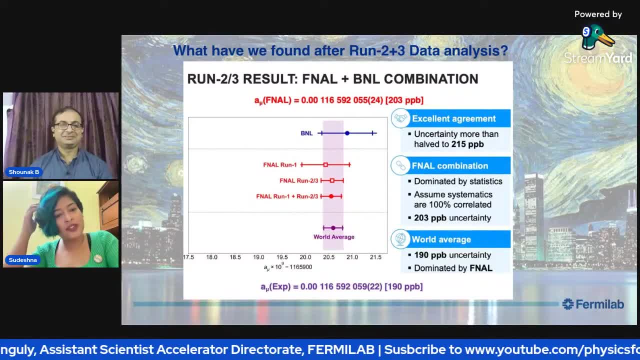 where the experimental result sits, and so we're extremely proud when this result came out, and the world is proud of you, dr ganguly, because you, you're there, you're going to take the great things. a very important question. if you don't mind, i will remove this, coming up from fatma. 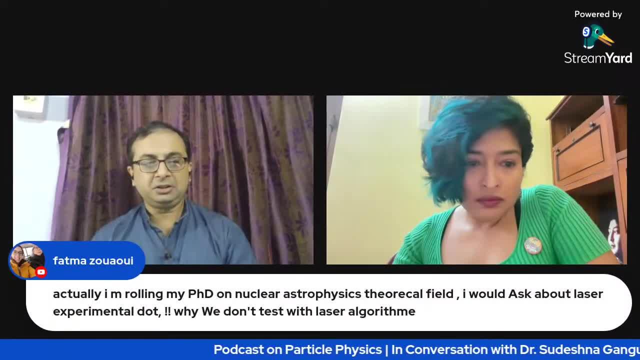 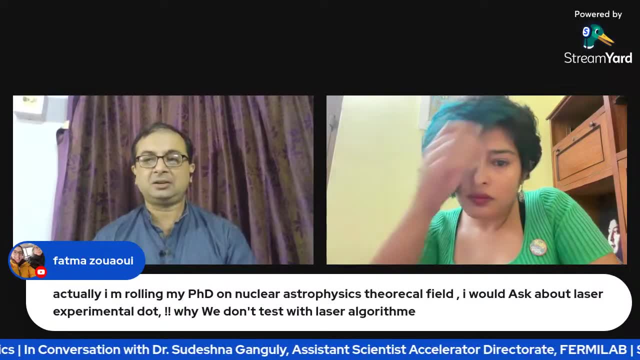 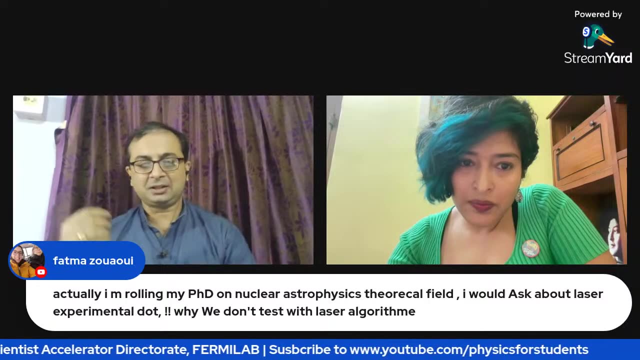 uh, zawawi, actually i'm rolling a phd on nuclear astrophysics theoretical field. i would ask about laser experiment, dot. uh, why we don't test with laser algorithms. so what, what exactly do you want to test? yeah, i think, fatma, if you're listening us. uh, dr ganguly is asking if you can put it a little. 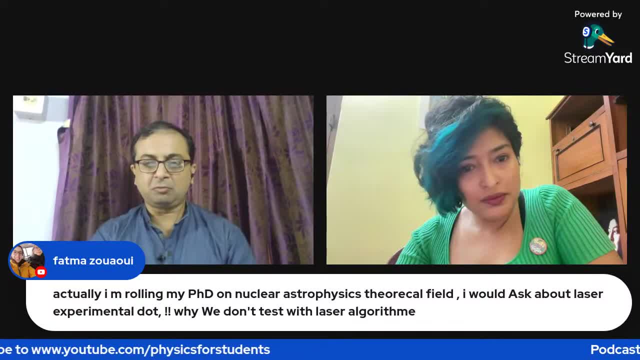 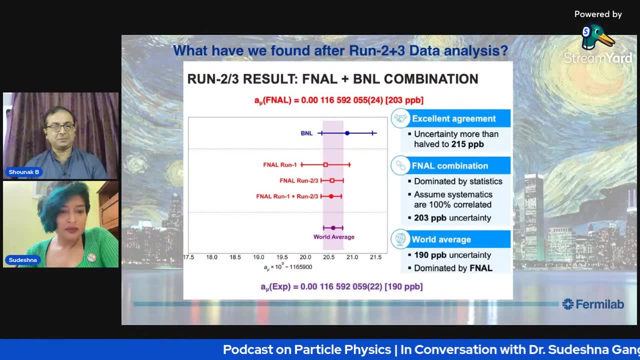 bit more. i think that would be much. she wants to know what actually you want to take. if you can put in the chat box, i will quickly get to it. yeah, so what you were explaining. i'm sorry to interfere. no, yeah, that's. that's totally fine. i was just saying so. this is where we stand with g. 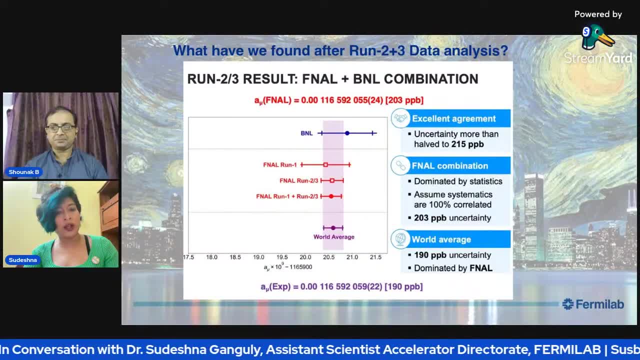 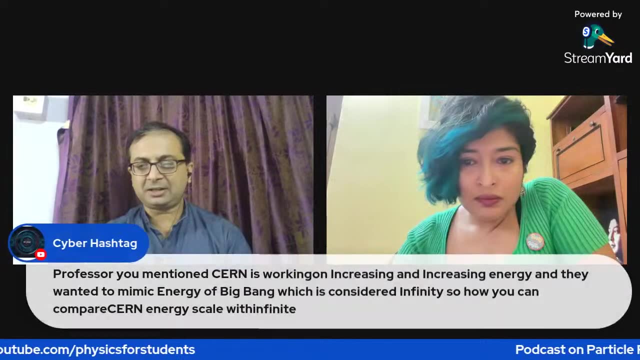 minus two right now, and we are waiting for our theory colleagues to update their calculation as well, and then we will see where we stand in terms of the discrepancy. okay, the discrepancy is interesting because that tells us they're probably new physics. uh, there's a question from cyber hashtag coming up. a professor you mentioned, cern, is working on. 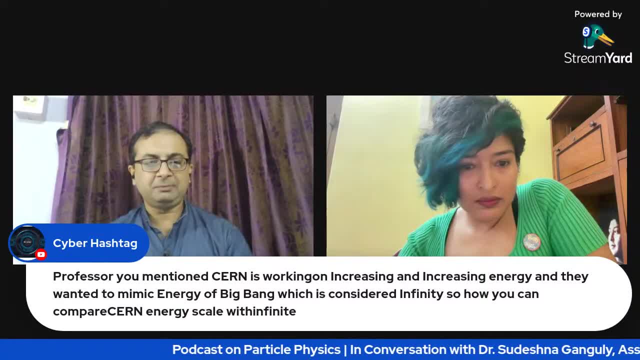 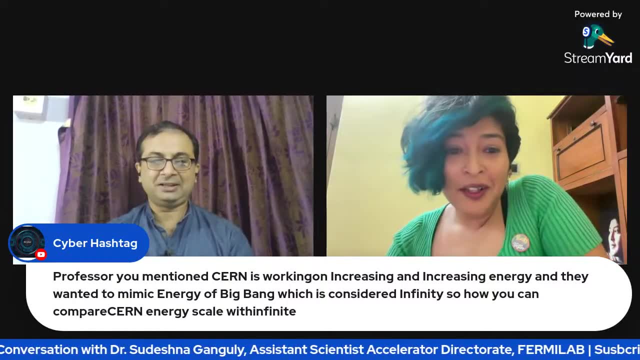 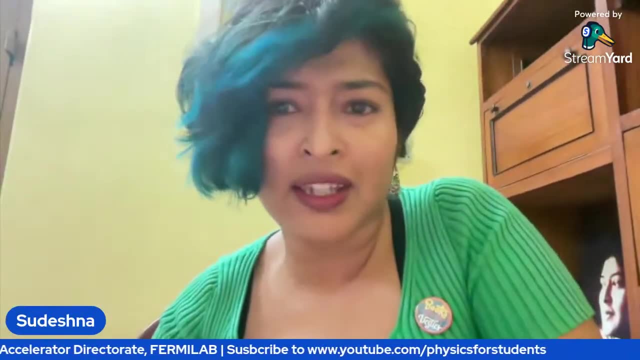 increasing and increasing energy and they want to mimic energy of big bang, which is considered. so how can you compare cern energy scale with infinite? well, cern, i don't think cern- has the ability to mimic infinity. they, they are, they have, they are creating a lot of energy. i think they are. 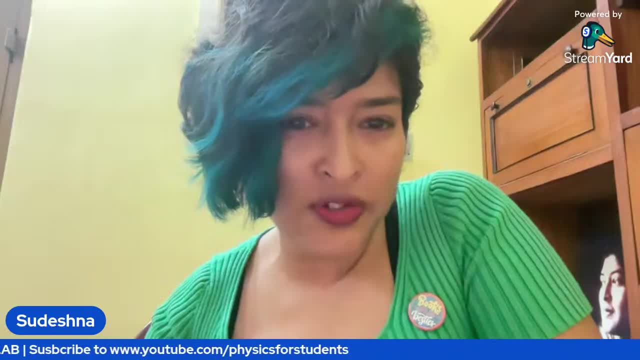 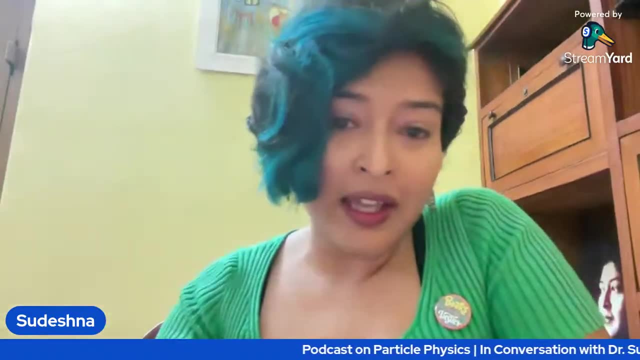 in the uh tv range right now, most likely 6.8 tv or something. that's a lot of energy. so so what i said? they are trying to mimic something like what happened in early universe. like when you smash very high energy particles, you create new particles, soups of new particles. 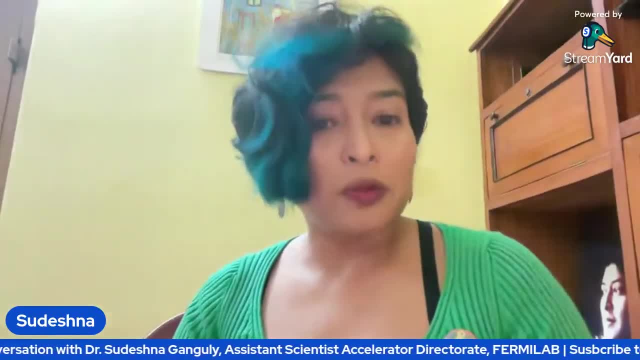 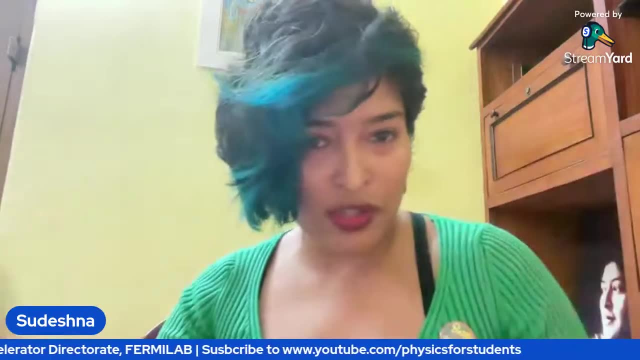 and they knew, studied the properties of those particles. so by by big bang i meant those initial state when you were smashing protons into protons and creating many more new particles and studying those. so so that's what they're trying to do, but the amount of energy they have 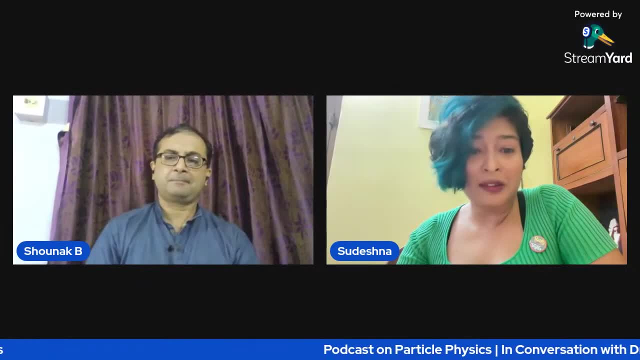 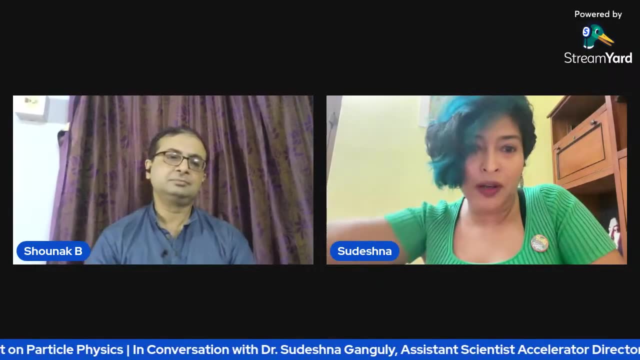 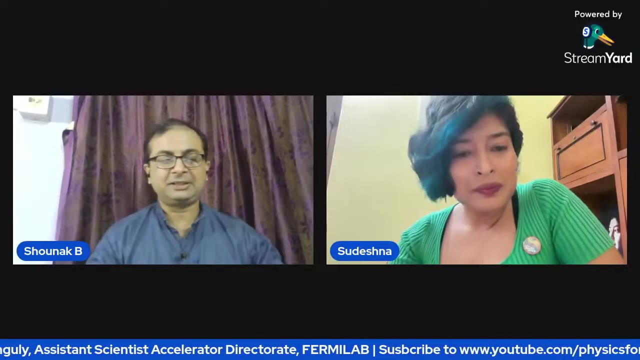 reached. that's immense, um, and so that's already immense. but but then the question is, what if this new physics is beyond their reach? it could be just lying above and it's not humanly possible to that much energy in a laboratory setup. yeah, i will go to shubham's question before that's uh. 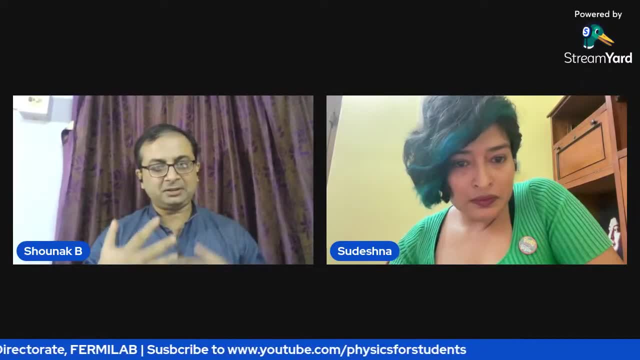 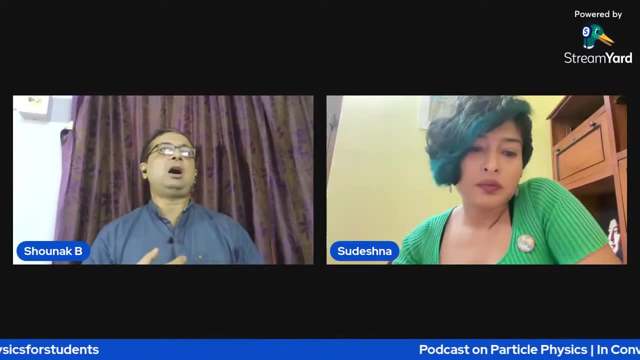 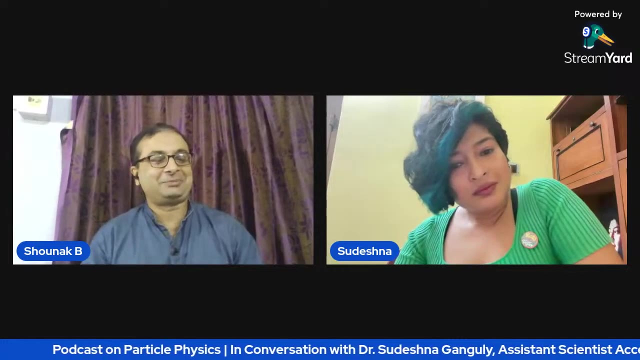 dr ganguly. one question is that this colliding of particles which came to my mind, it includes a huge amount of fund. i mean to say finance and money. uh, yeah, i i want to understand on a very basic level, what is this? i might- i don't know whether i'm being to explain- what is the cost. 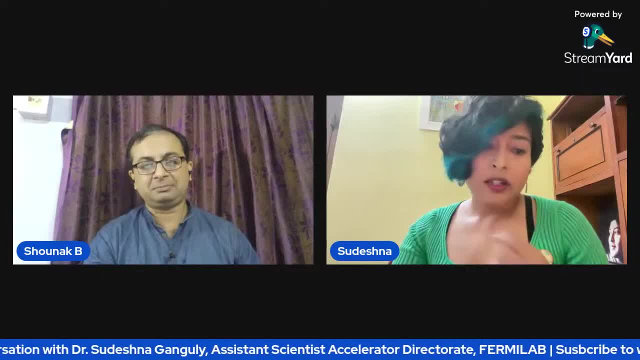 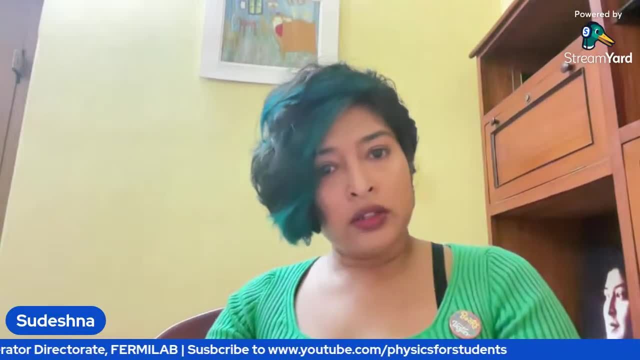 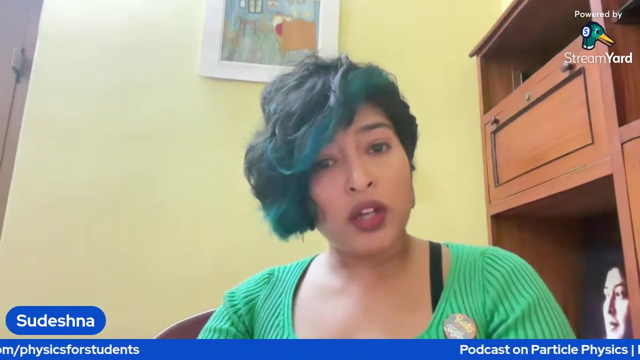 and how is the cost involved? and approximately? yeah, i cannot talk about cern, but for family i can totally like give you an idea. uh, because i was the accelerator run coordinator, which means i was in charge of running all the machines that i show right. so, um, to run. so if we, if we do not run the 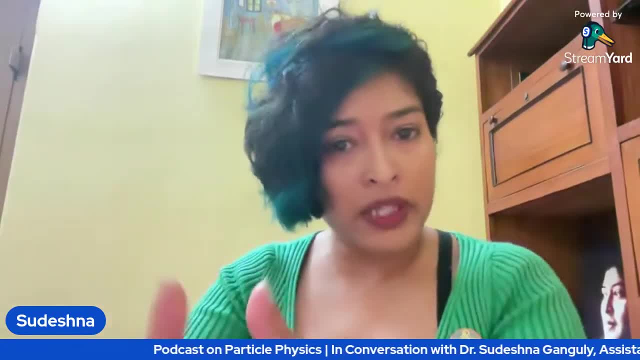 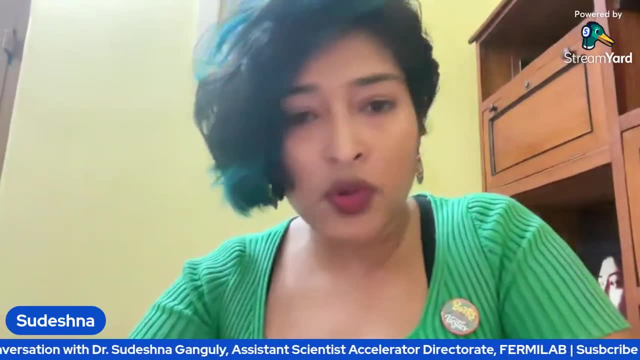 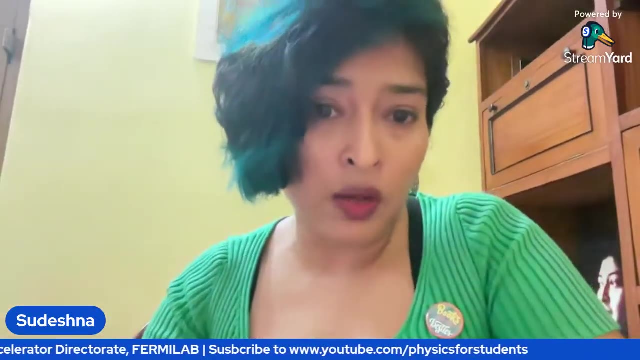 machines, and if we do not, we are not able to provide beam to the end users, say, for one hour. that would cost about million dollars. so our first priority is to keep running the machines and deliver beam. to just keep running machines and not deliver means meaning you're wasting million dollars per hour, you know. so it's that level. 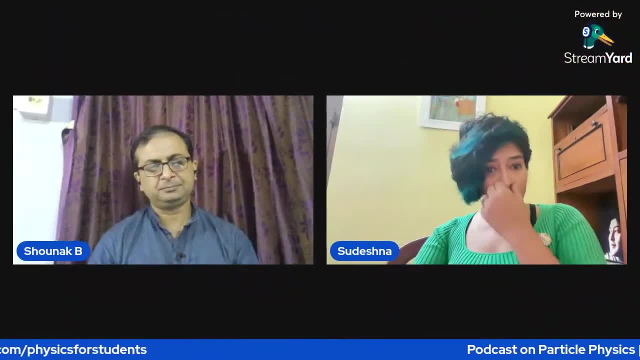 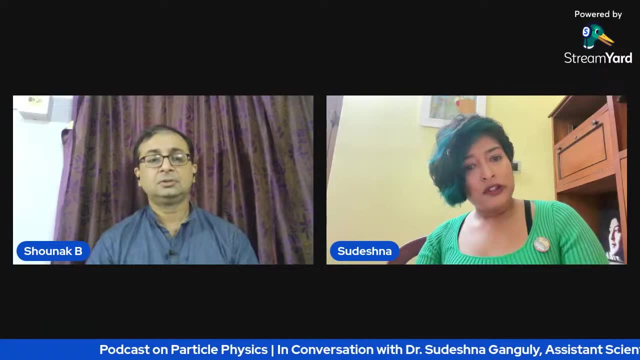 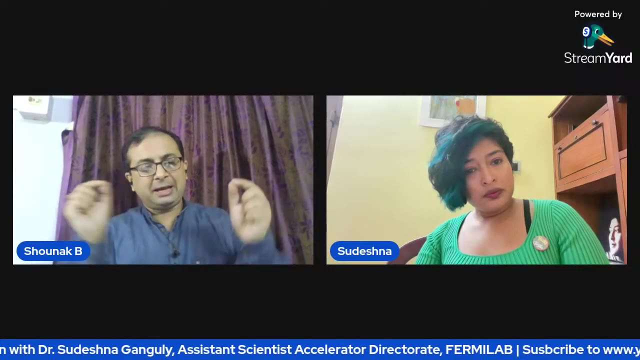 so you can imagine like building those machines. so g minus 2 is a very small, small experiment. but even that small size experiment requires approximately 50 million or so. so dune is a billion dollar experiment. there'll be a beam line and doom and when we are, you know, emitting particles, so that 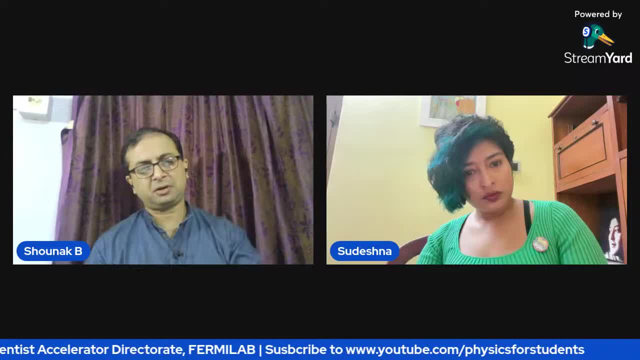 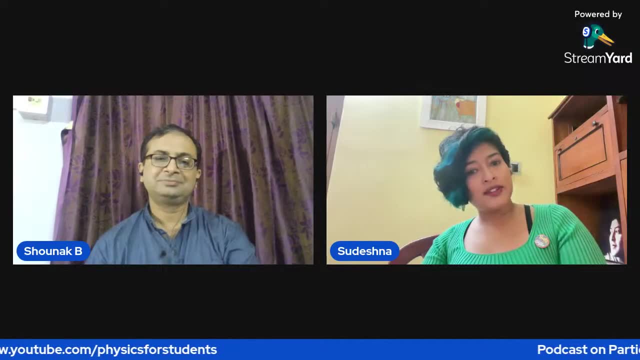 they go ahead in the tunnel and collide. does that also include a lot of cost? yeah, yeah, because yeah. so when we physicists, we typically don't think about practical things, to be honest. but now that i'm working in the beam line, i see what you have to think about, um. 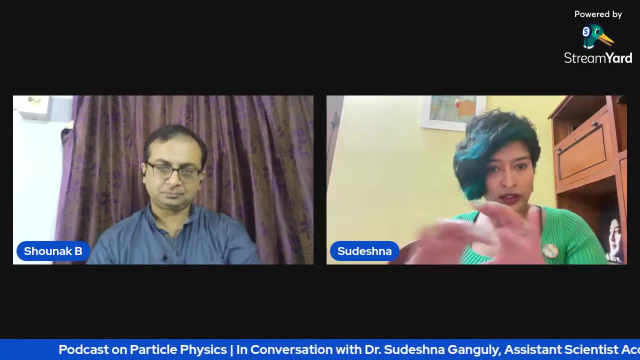 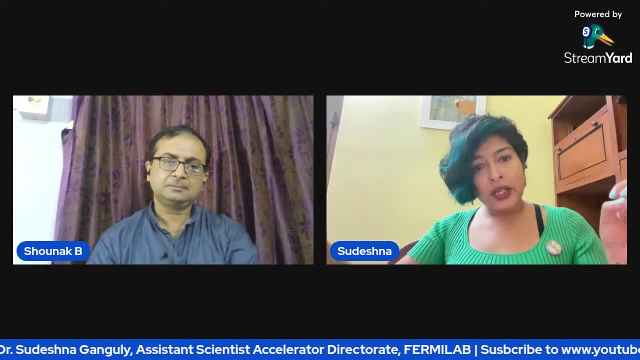 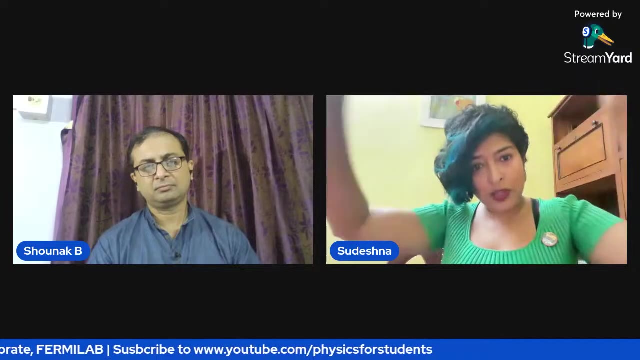 so? so suppose you have this magnetic horn, this focusing horns. these are like focusing charge particles. these are huge, enormous machines, so you will have to have structures to hold them. then you will have to have steels to shield them around so that radiation doesn't come out. you'll have to charge it, so you'll have to have strip lines. 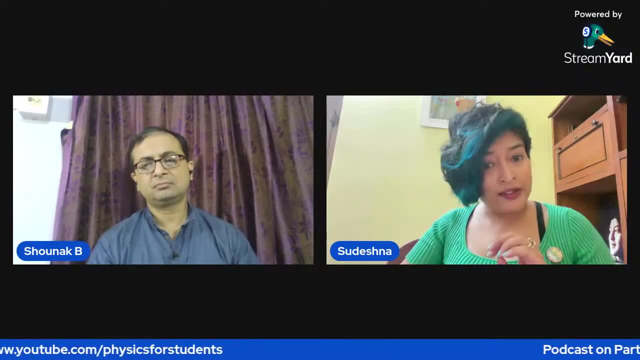 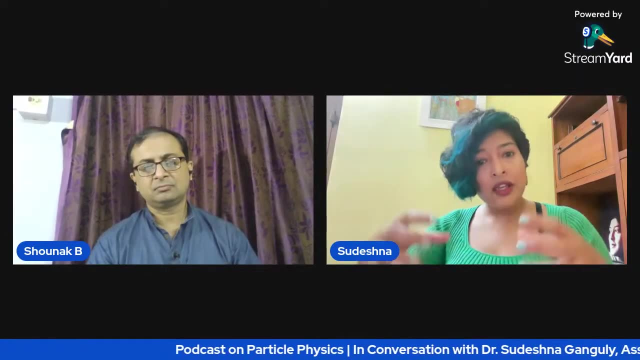 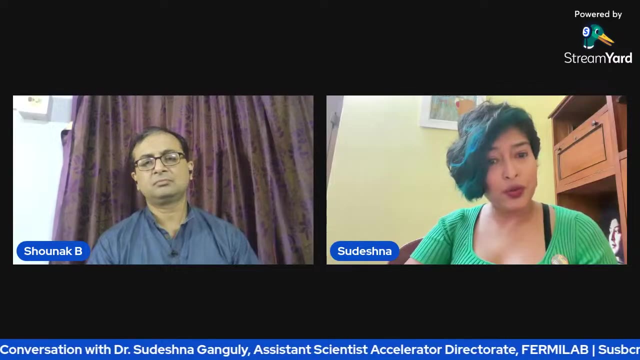 you'll have to have huge cables, cooling gas. so cooling is super important, otherwise they're gonna not going to survive. so cooling gas, just a tiny graphite target, that would take a case, a cooling system, something to hold. it cascades. so when something is hot, what do you do? you cannot just take each radioactive material, so you'll have to have coffins to call. 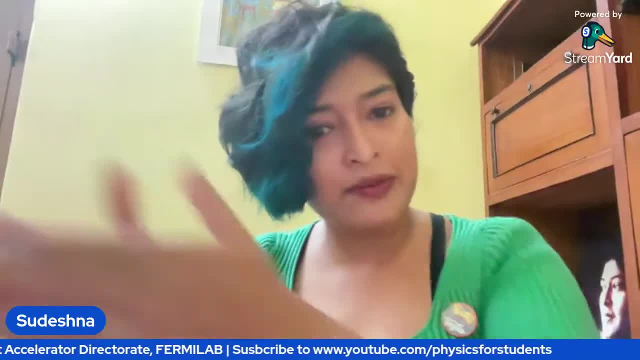 them, coffins, and you'll have to have facility to store them, to take them to the facility. so when we do to store them, so we'll take them to the facility, so it will have to have capacity to take them to the facility, so to the facility. so it's like the just the day-to-day practicality of handling these machines is immense. 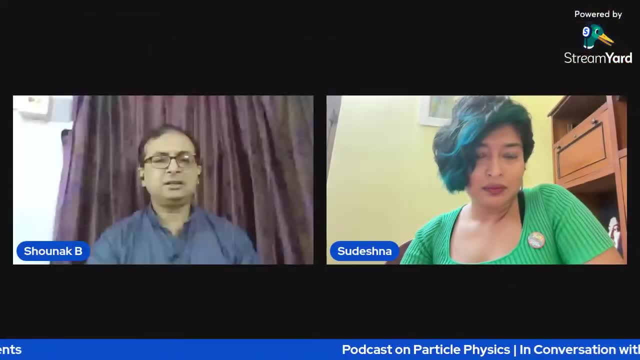 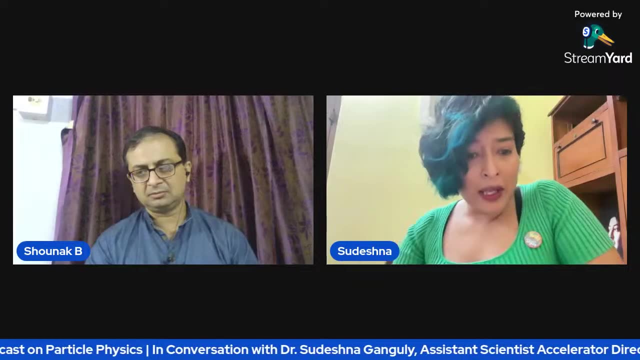 and costs a lot of money, and these machines are actually made on the lab or they come from somewhere and they get assembled. most of them are made at the lab. so right now, our engineers are actually welding the horns, they're, they're creating and they then they create spares as 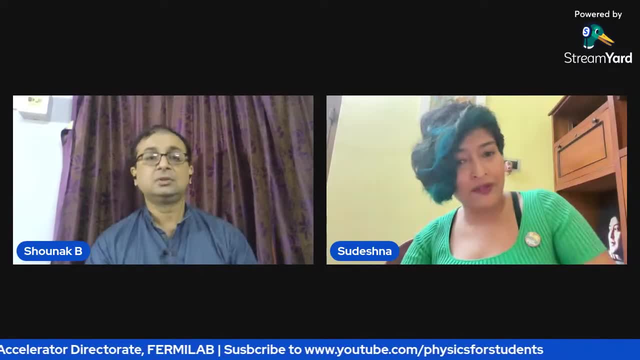 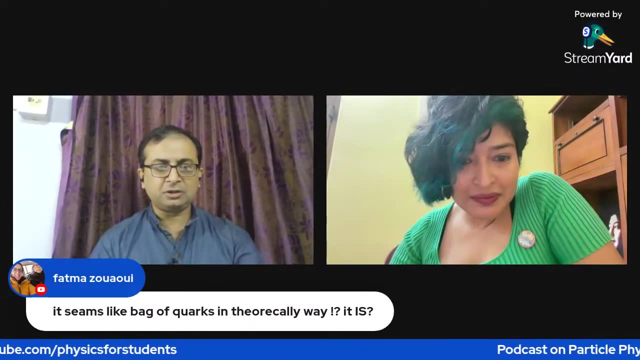 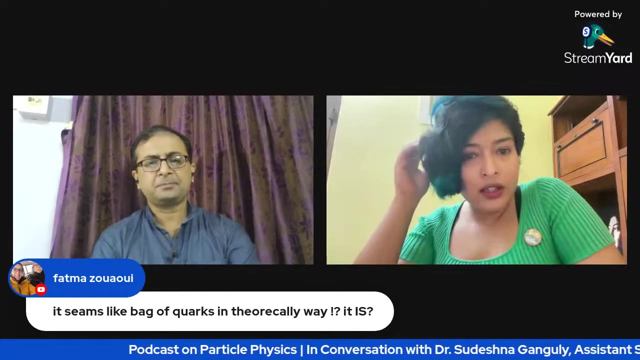 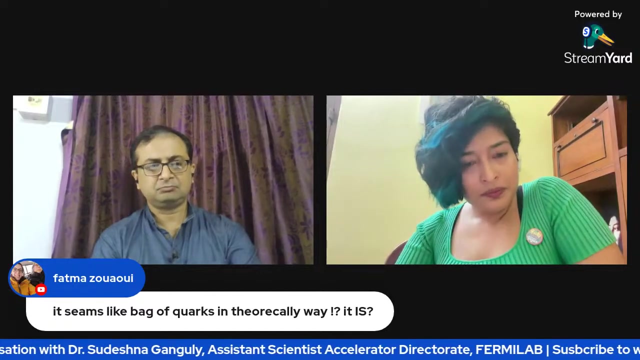 well, you cannot just create one huge machine. you have to create spares in case they fail. okay, fatma has got the answer. it seems like bag of quarks. in theoretical way it is. yeah, you can call it a bag of quarks. um, like another particle, like the mesons or variants, they're a bag of quarks. yeah, okay. 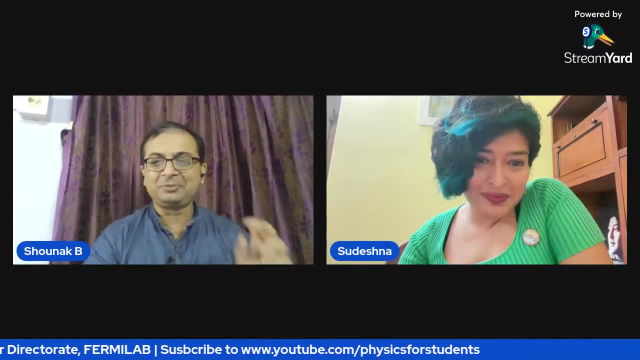 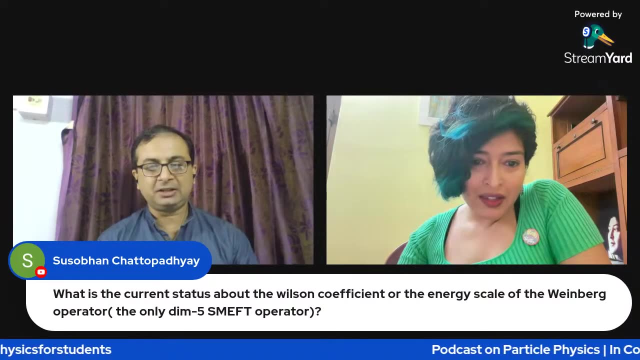 yeah, we are almost an hour but uh, i would take few minutes time, doctor, to take few minutes more questions. uh. so someone is asking what is the current status about the wilson coefficient of the energy scale of the weinberg operator i i cannot answer that this is not my field. but 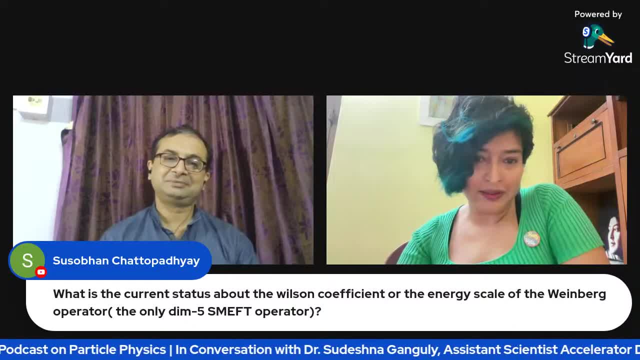 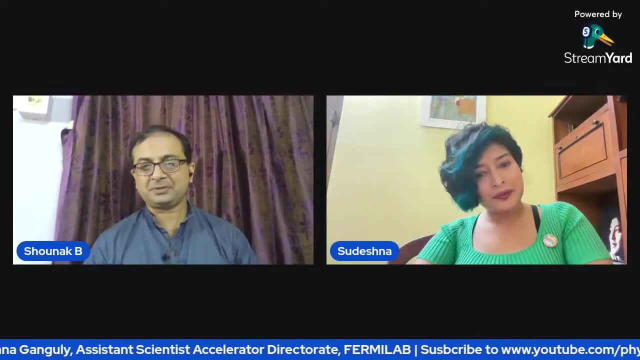 if you are interested, i can hook you up with someone who is working on that. sure, and i would request to get in touch with dr ganguly. absolutely, if you share my email id, yeah, doctor, if you can just put it in the chat box or if you want, exactly, i will do that. 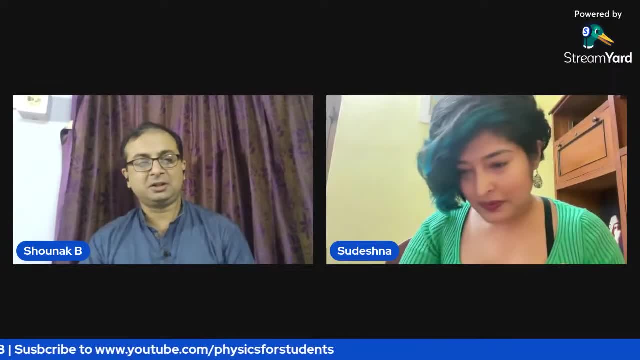 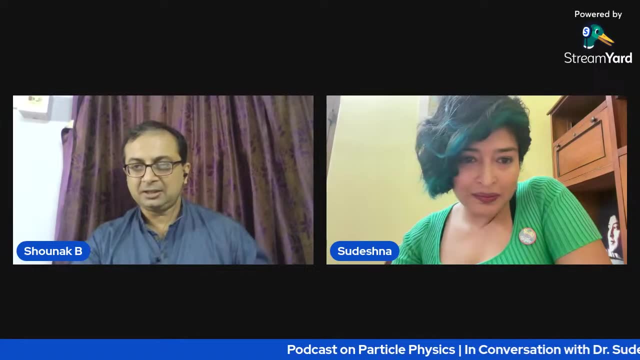 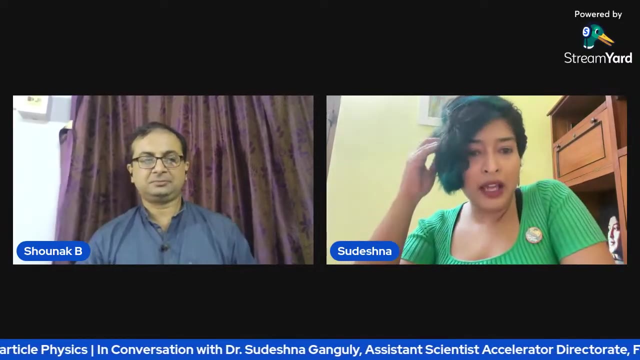 flash it over the screen. so this is dr ganguly's- uh you know, uh- email id, uh, and i would request all of you to you know, just to look into that. just a second. let me just put it in the chat box so that it is available for everyone, and then my slide decks it. 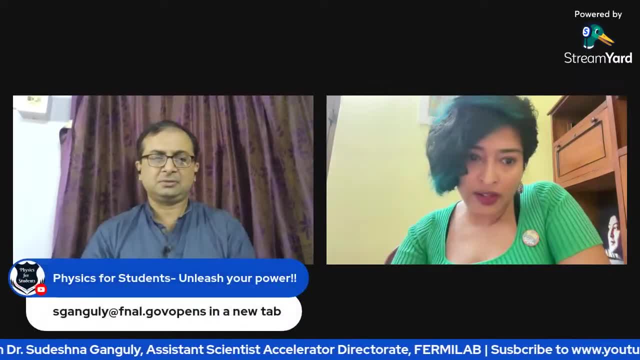 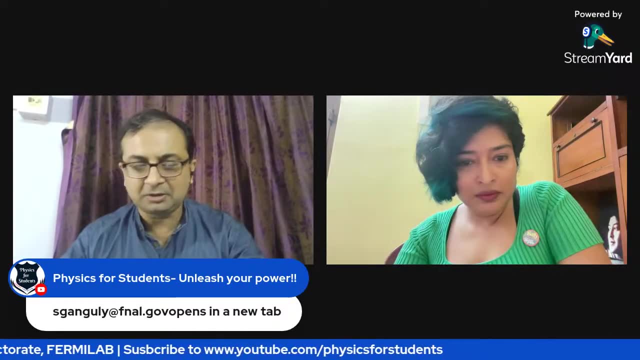 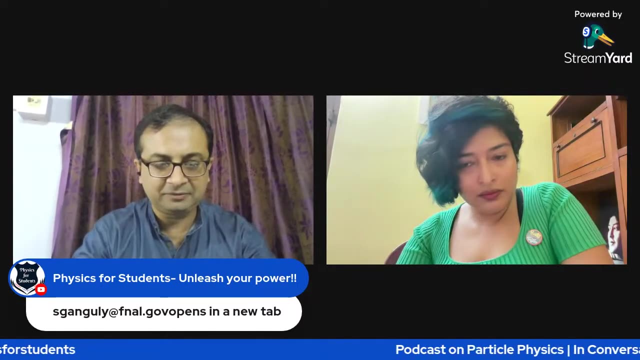 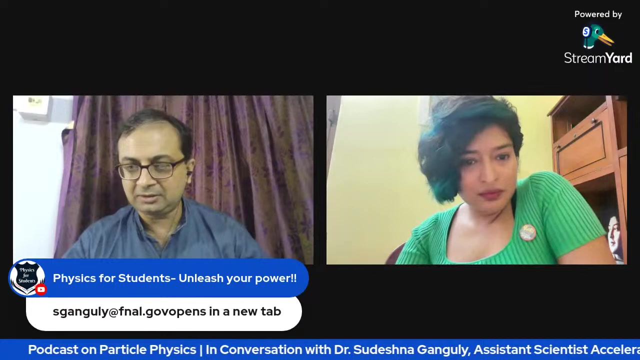 has a lot of links, uh, related to formula. if people are interested, that might be interesting. yeah, so you can just ignore the other part. yeah, let me put it across. so it is s g a n g u l y at the red: f n a l dot g o v. i will put it on a fresh page so that, uh, it comes in the visible. 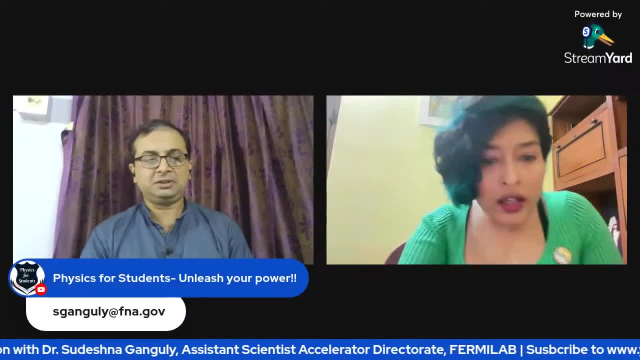 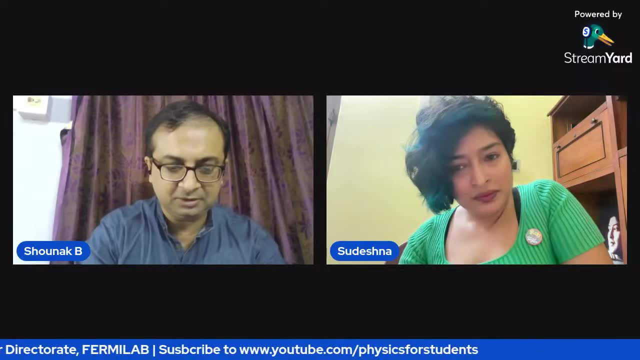 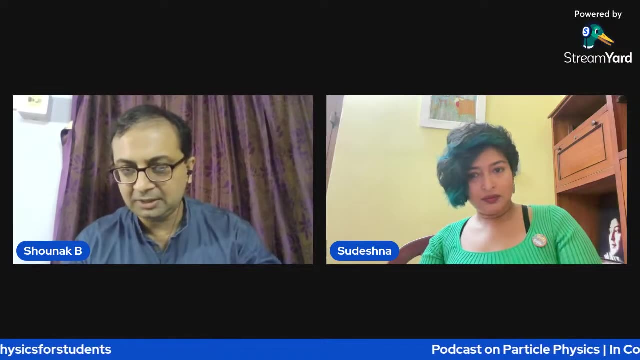 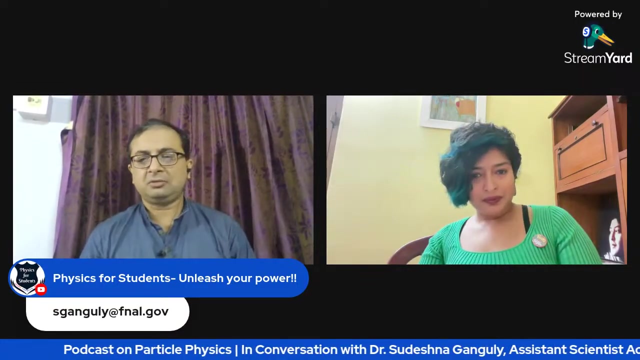 not this one, this one, yeah, so this is dr ganguly's email. i, i'm so sorry. yeah, yeah, yeah, and you, i think this is is the one. yeah, right, so this is dr ganguly's email id. uh, officially, any one of you is willing to contact her can contact for, uh, education purpose, for, etc. that is the purpose of physics. 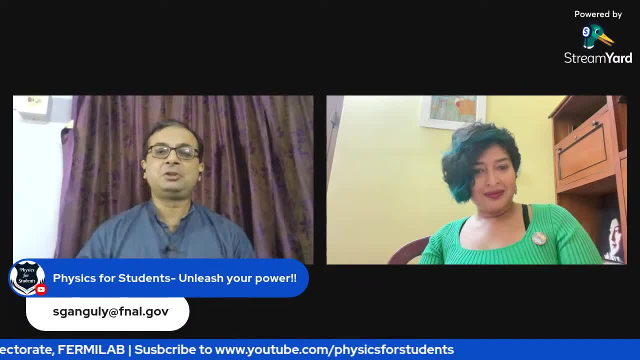 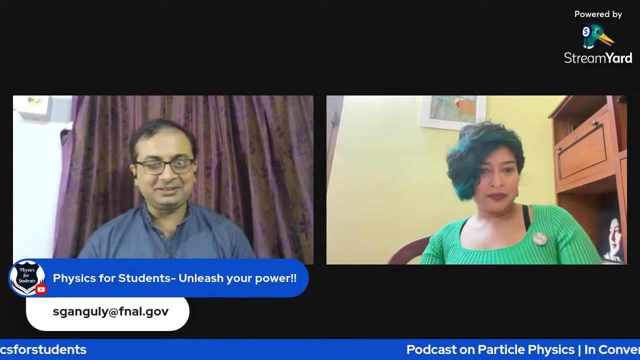 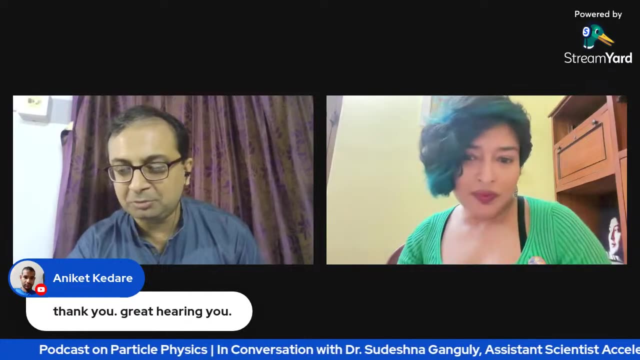 for students as a channel that you you get more motivated and bringing experts uh like you. uh, that's, that's uh wonderful. uh, aniket is telling that. uh. thank you uh, professor. uh, great to hear from you. uh. one question coming up from susabun is that, uh, when you showed the result for moon g2? 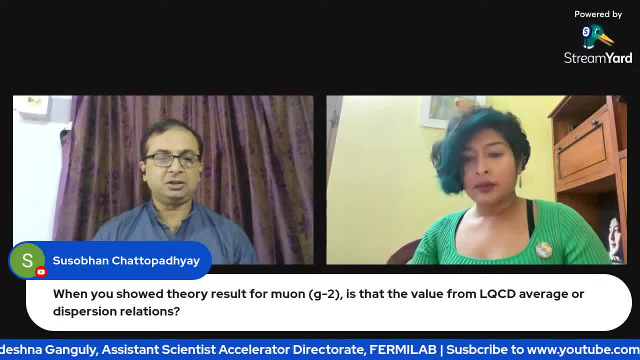 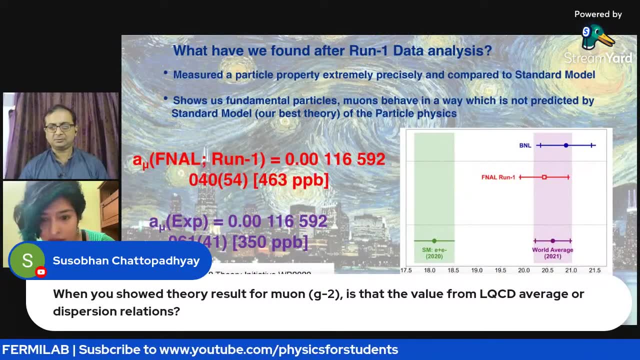 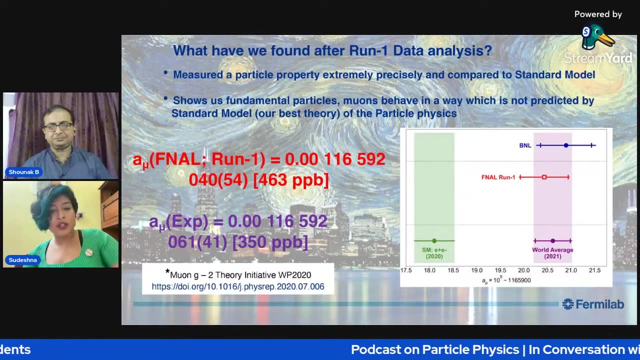 that the value from lqcd average on dispersion relations shall i show you. i think 2020 was dispersion. let me see. does it say on my slide? i cannot see so, so you can see the theory initiative. but yeah, it is. i think it is. it includes dispersion. it was dispersion 2020.. 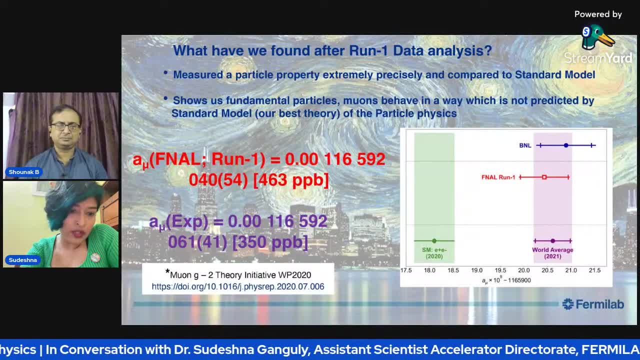 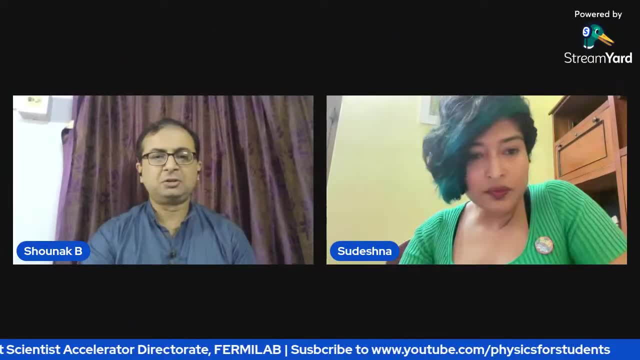 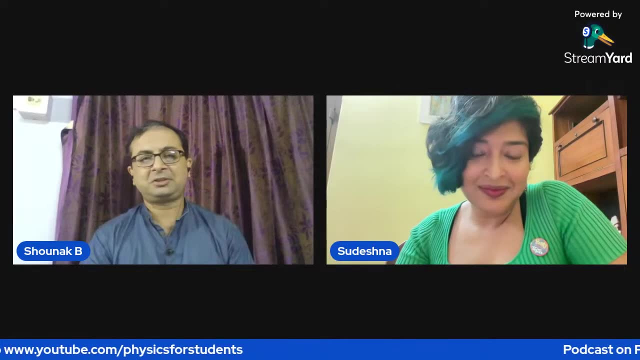 uh, but i would encourage you to check the theory initiative uh white paper from 2020. that has more details, right? so, uh, i mean to say i really have no words to thank you, doctor, because we were all waiting for this kind of uh, uh, you know, because we got huge amount of questions we never got. 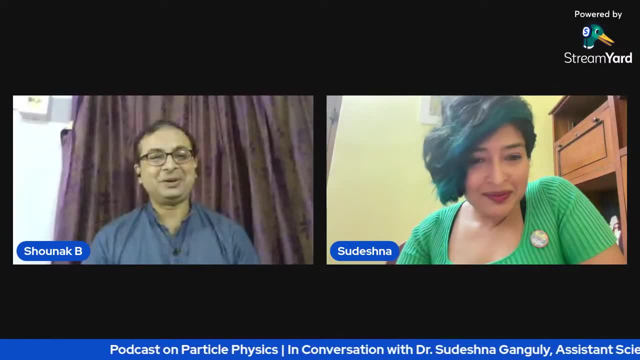 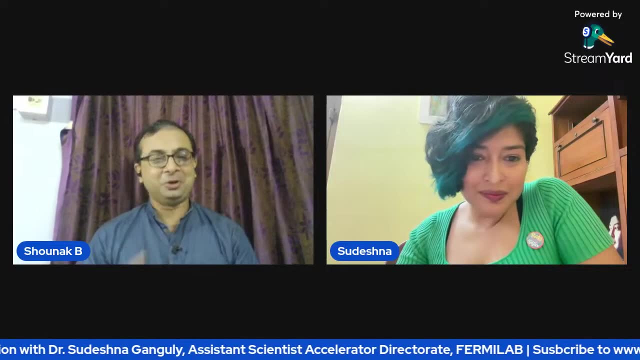 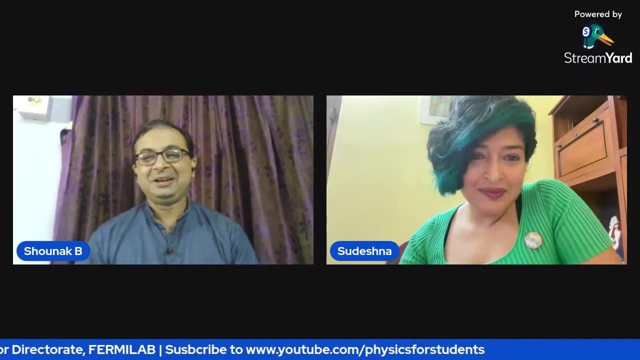 a theory, a particle physicist coming in and uh, you know asking, and i can uh request from all those people who are right now watching you that we won't let you go. i know you were terribly busy. you would be again going back to us with your experiments down deep into the channel. very busy. 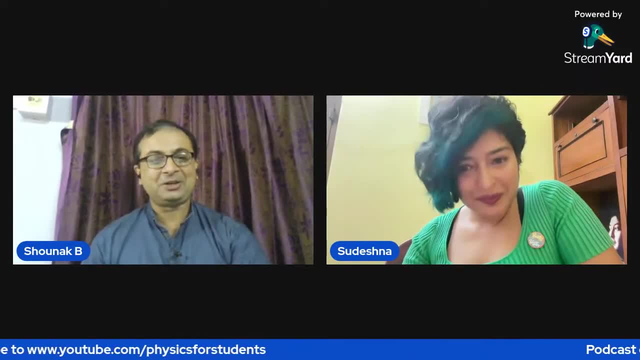 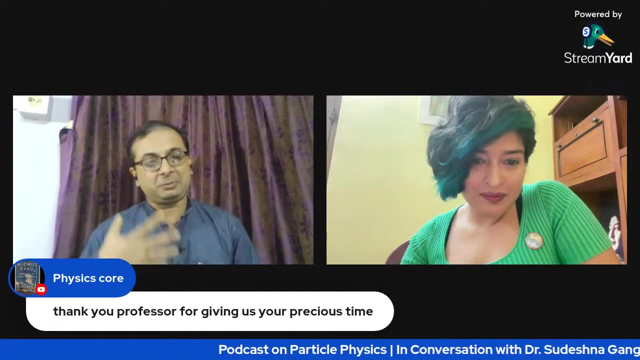 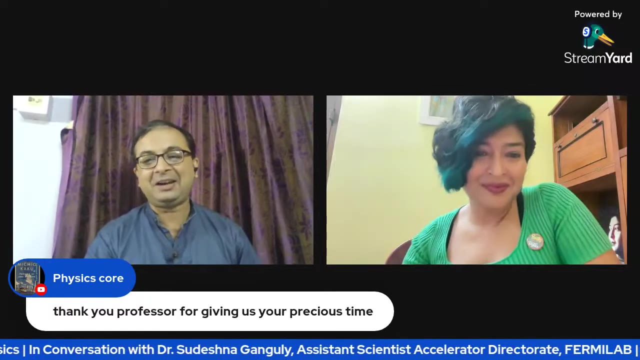 person, but i will definitely try to contact you because this is something, and most importantly thing, is that i- i think all of you would agree that, uh, the ex the complexities that are there in particle physics, that was, you know, elucidated in a very natural and a very fun, loving manner. 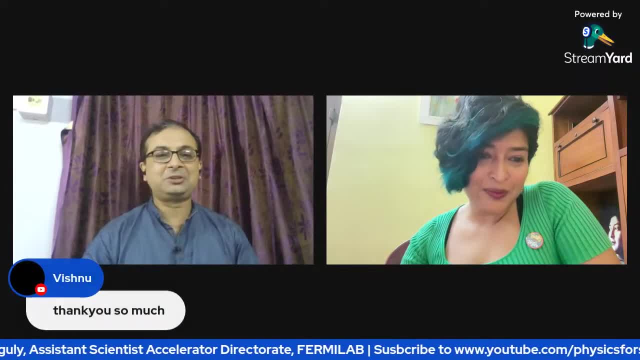 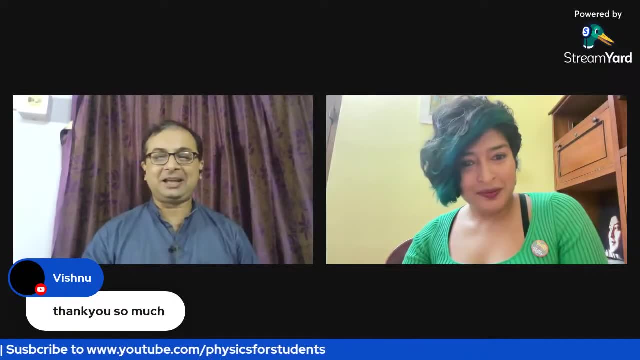 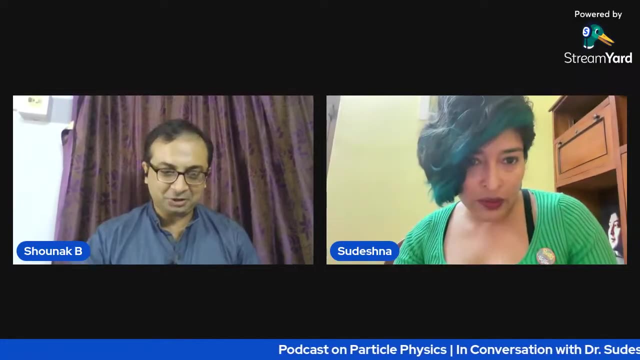 a lot of thanks coming up, fatima. uh, thank you. thank you so much, so i had a lot of fun. okay, any last message, doctor, you would like to give those who are pursuing would be willing to be coming. regarding particle physics, can you put my slides back up one second please? one last slide, it is. 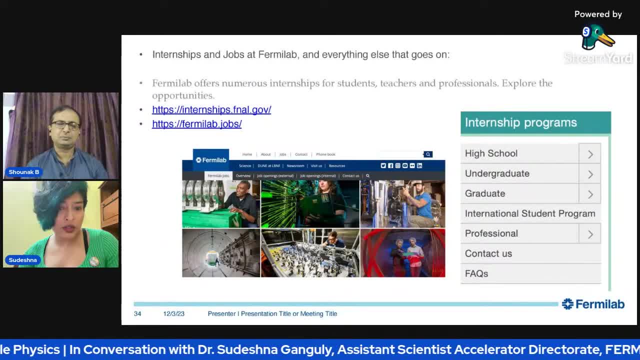 about, uh, this slide. so we do take interns at formula, both national and international. so this is a good way to work at premier lab. so we do take interns at premier lab, both national and international. so this is a good way to work at premier lab. so this is a good way to work at premier lab. 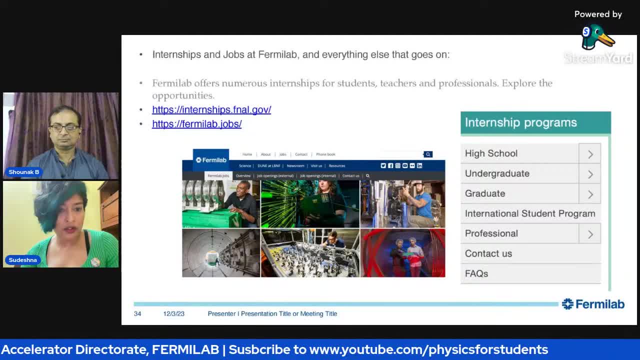 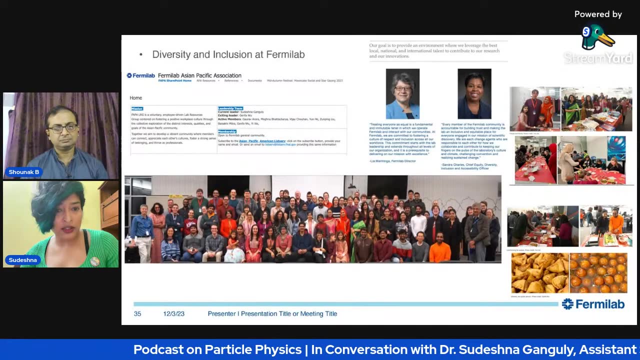 also family of jobs. they're always posting jobs for postdocs, for permanent positions, for competing associates, machine learning associates, so this is a very good resource. and we do have an asian family of asian pacific association. i'm the co-leader and we just celebrated diwali, so we will. 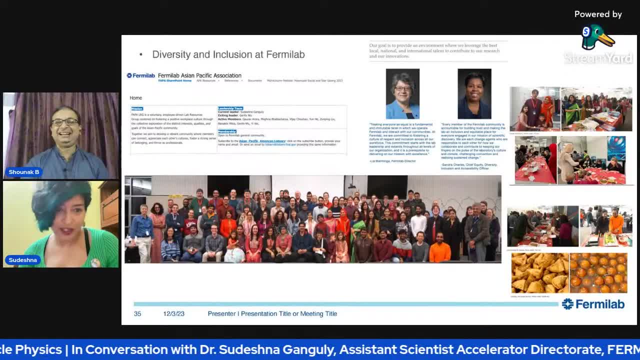 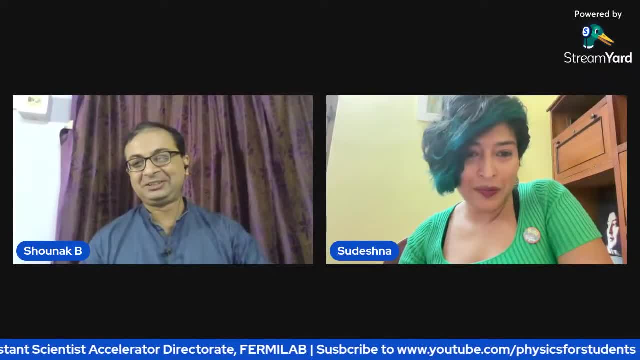 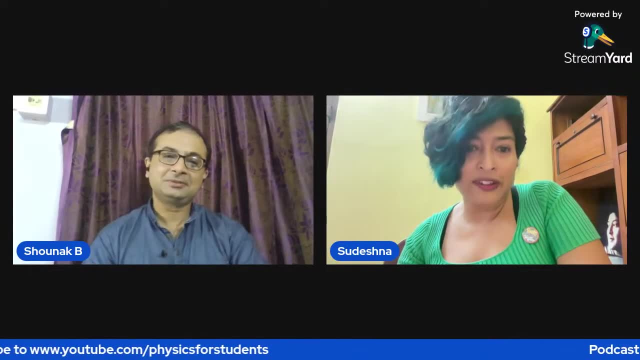 get a lot of indian food: samosas and gulab jamun. so come join us. that's wonderful, i mean to say so. you have a kind of a- you know this kind of a culture of how things would be. we do have a very active um, diversity, inclusion, uh- workforce there. 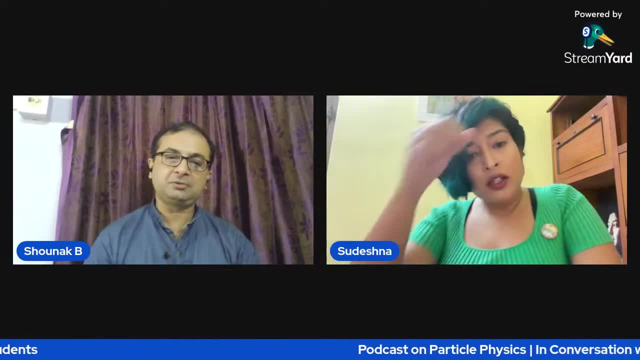 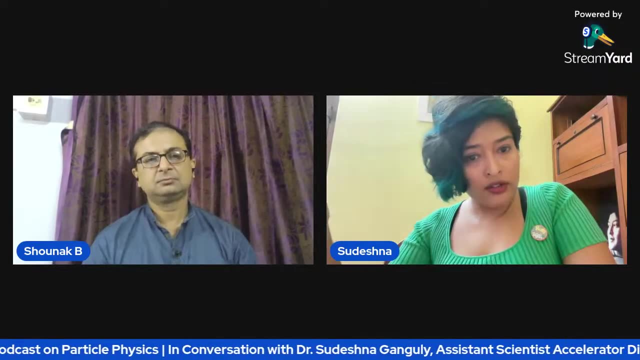 okay, so what is the eligibility doctor for getting an internship? over formula internship: we we take internships, uh at different levels, high schoolers uh, undergrads, masters- at different levels. so if you go to that page, there are many- about 20 internship programs that people can come. 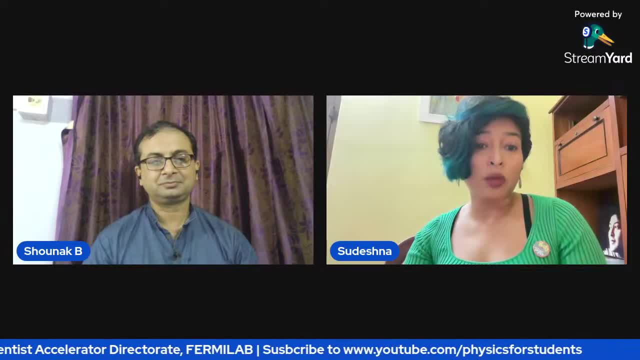 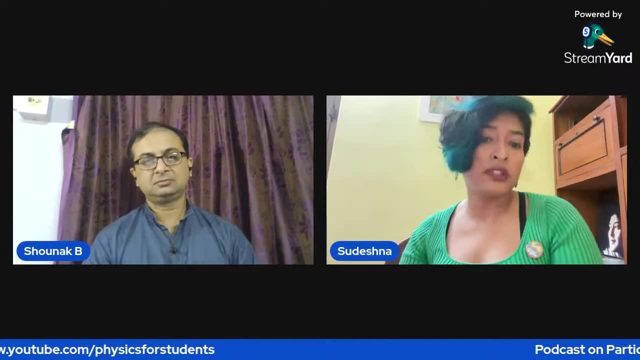 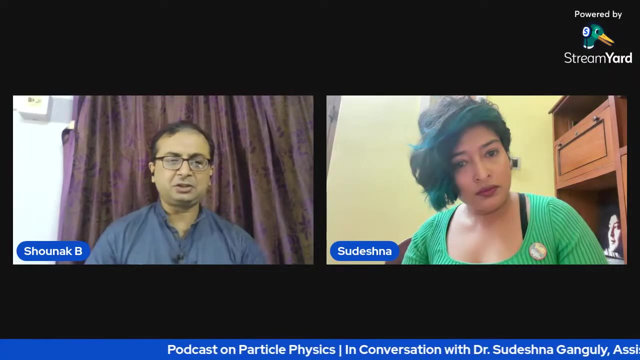 work with us and that's a very good way to find job later at the lab, because if you make an impression they will try to hire you later. so yeah, to be in the system. so that's a very good way. into formula that means if somebody has got a kind of an specialization in instrumentation or something. 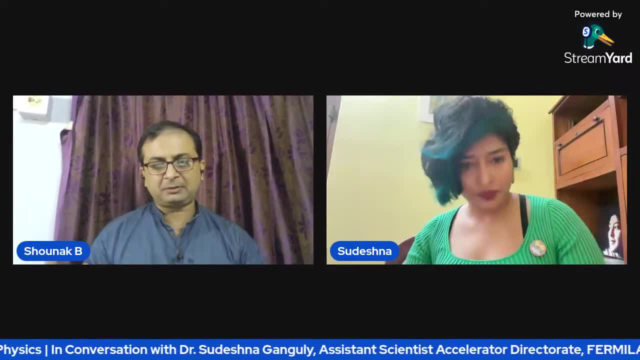 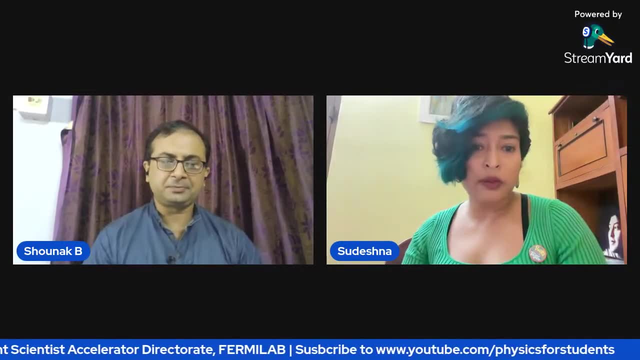 like that. i think that works much better. yeah, rather than pure mathematics or something like that. right, your mathematics would work if somebody wants to join the theory group, but if some hands on experimental experience exists, then there would be. there will be many more options to work at the 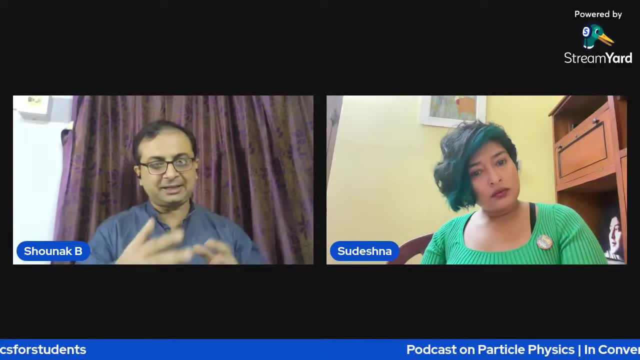 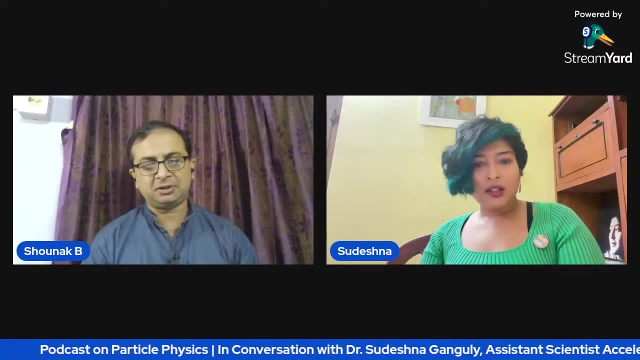 okay. so when you were telling about you control those first, second and third, both the analysis, the hardware. so is it that you took a separate course? or you, how do you think to know about the hardwares just every day, working with experts? so you learn, learn on the fly. yeah, learn on the flight. 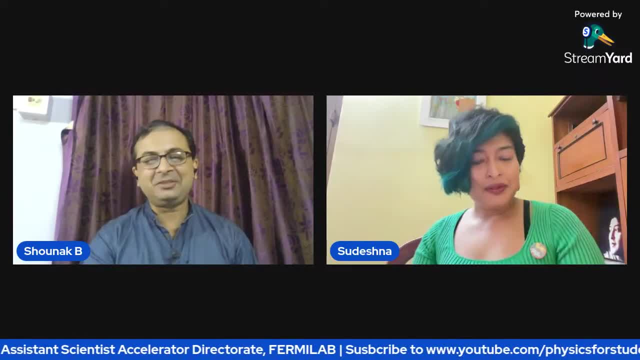 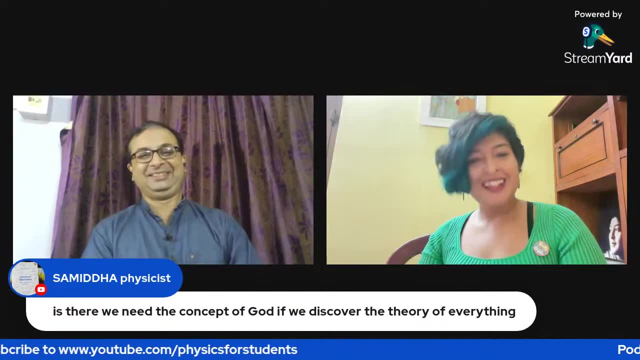 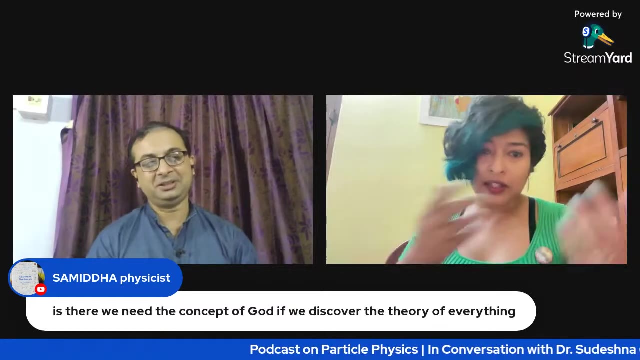 i think that is the best thing. one last question, i think it is. we can take it on a very casual mode. it's little bit. this is there. we need the concept of god if we discover cam, the theory of a kind, well, yeah, so this is, physics is always in the realm of spirituality, back in the days, like olden days. 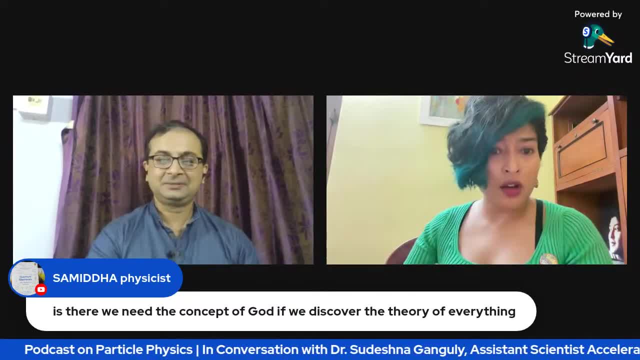 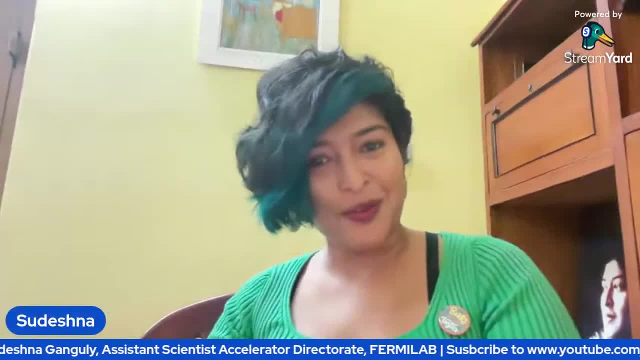 ancient time, philosophy and physics, they were the same. that's why it's doctor of philosophy, right. so how you would look at it, you would look at it technically or you look at it spiritually, it's totally up to the people, because from the experiments also, it seems that everything. 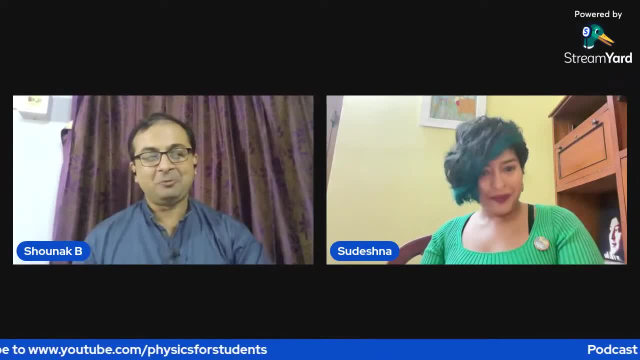 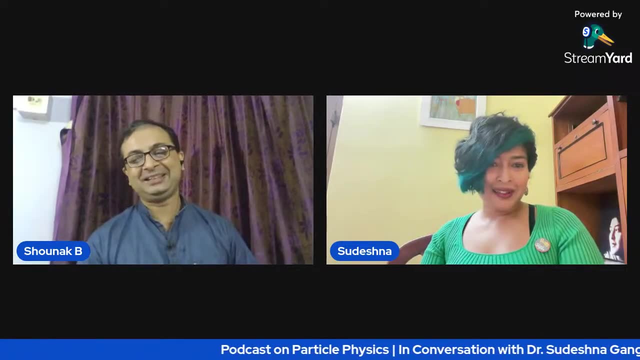 is merging to the same superpower. whether you got it as 120 gev or you got it god, it is ultimately the same thing. thank you very much, doctor. a special thanks from my side. uh, so you have already told that there are interns, so those who are watching wants to go, and i have already. 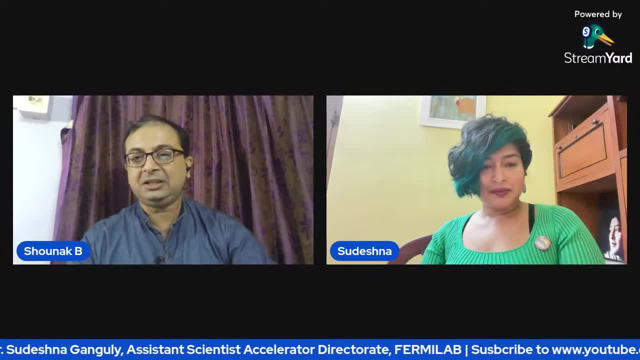 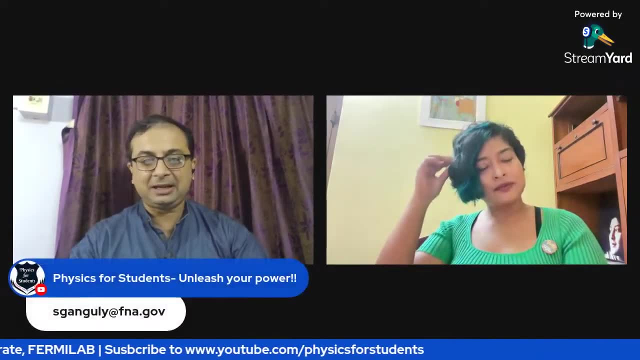 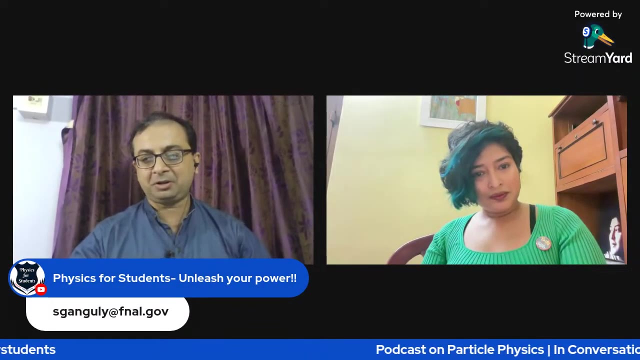 flashed uh doctor's email id right on the screen. so anybody willing to take up uh, you know a further contact her, you are welcome and this is the email id. just a second. this was the wrong one. this is the right one, so i'm just flashing one more because she is an extremely important and an 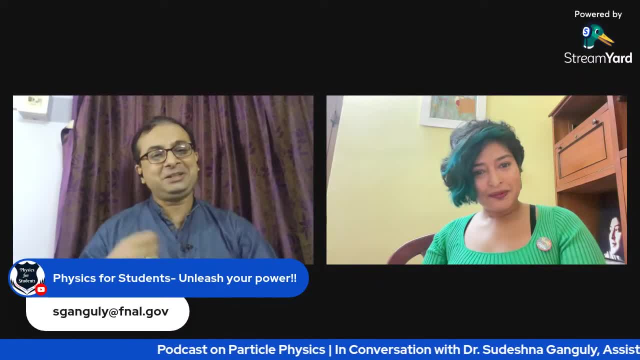 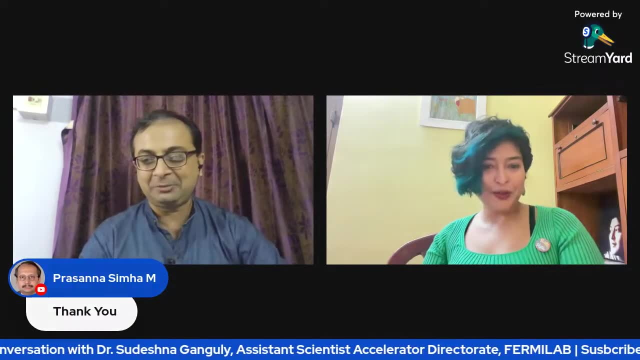 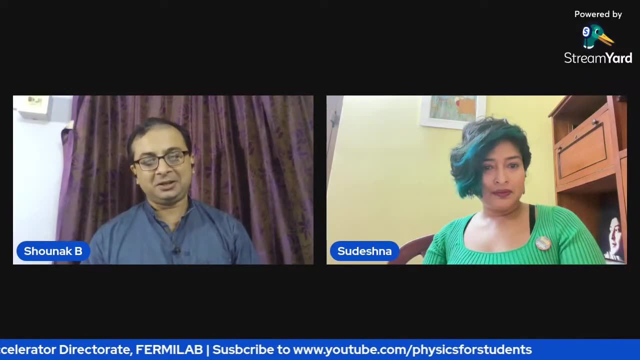 extremely experienced person working one of the most experienced and one of the greatest uh particle accelerator places. uh, our doctor extends his thank, dr prasanna, thank you very much, and just to let you know that we would be back on 17th of december uh with another uh person as a guest speaker, and this would this. 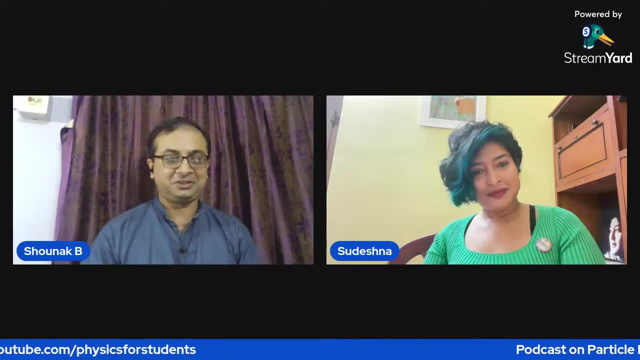 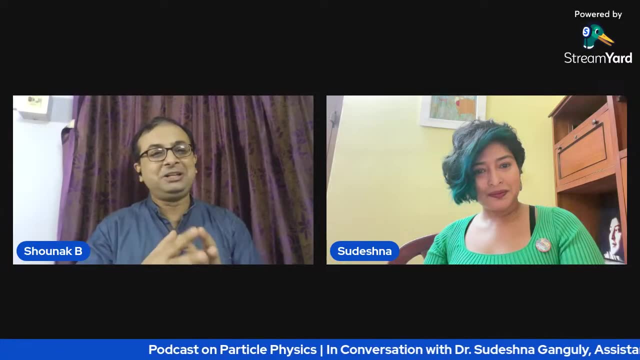 time it would be on quantum computing, artificial intelligence and data science. but i would like to thank dr ganguly again because i have been talking and, to be honest, you really don't know that how we actually make up the time, because she was extremely busy and you know every.